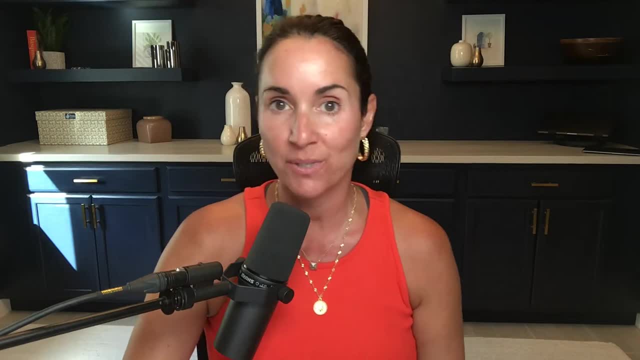 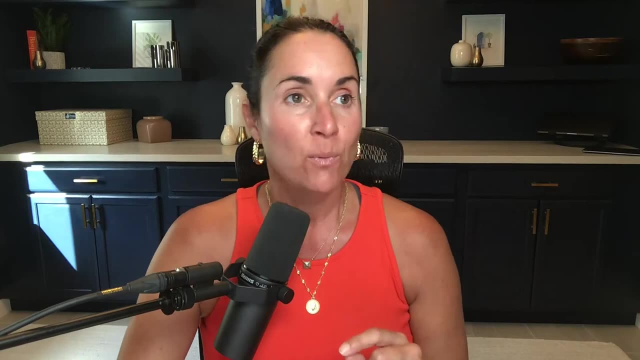 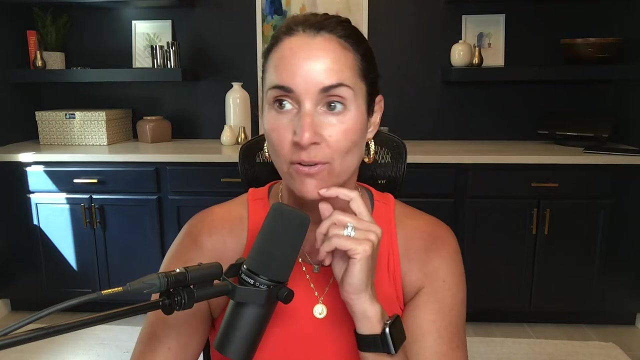 All right, Hey everybody. Kathleen Jasper here and I'm so excited to be with you today for the Praxis 5001 webinar. We are doing a free elementary education webinar today and I'm just checking on all my socials to make sure that I am live everywhere. 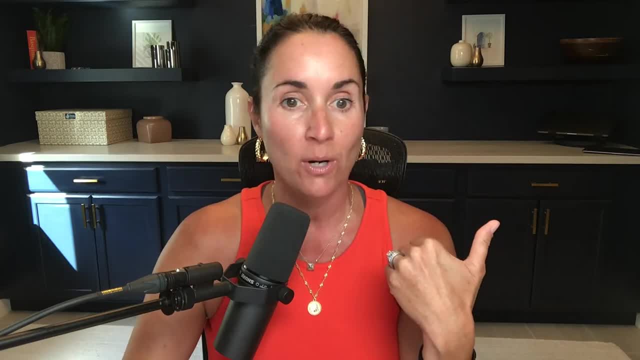 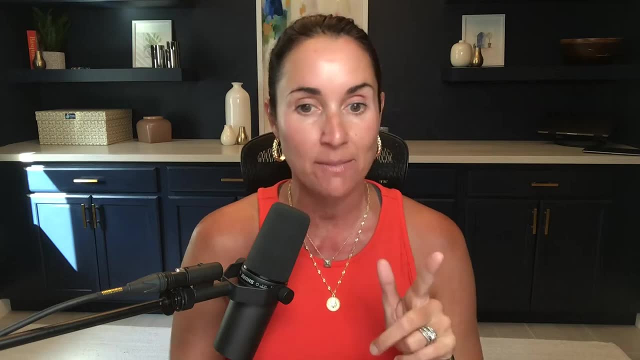 and it looks like I am. Let me just check. Come on into the webinar room and I'm live. Good, Come on into the webinar room. You can chat with me in the chat. Let me know that you can hear me and see me. okay, According to my stuff, my mic is on, My camera is on. Everyone can hear and see. 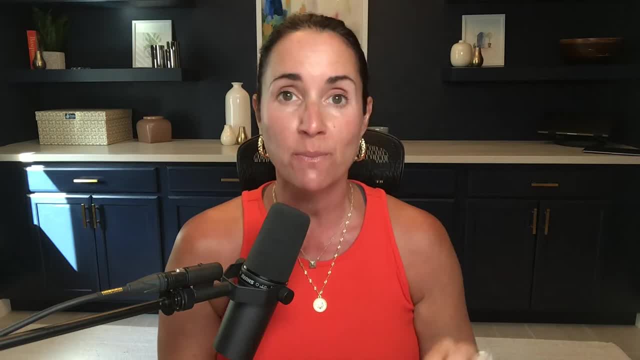 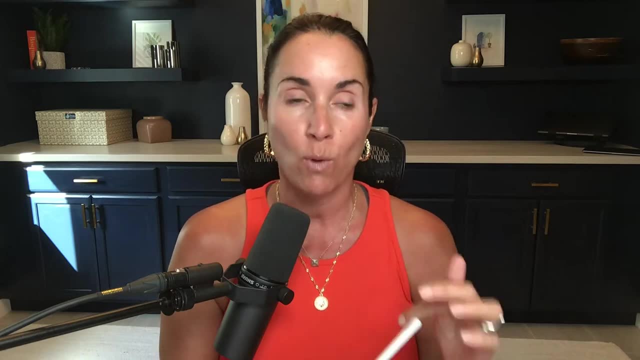 me, but just let me know in the chat that you are here. If you're watching me live on Facebook or YouTube or LinkedIn or wherever you get your social media, you can join the webinar through the link in the description. Just click the link in the description and it'll take you to grab. 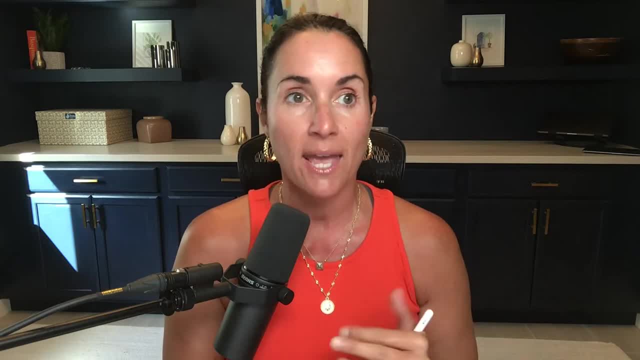 the resources for the webinar. With this free webinar comes a study guide, a mini study guide and some more information If you're interested in learning more about the Praxis 5001, and after the study guide or after the webinar is over, we will send you an email with all of the 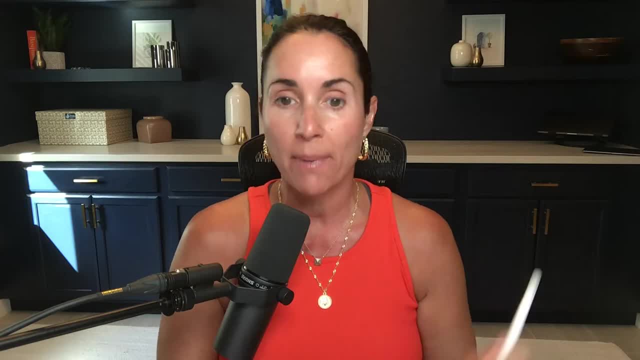 information I talk about today. Don't worry about taking notes and trying to record everything I say. You're going to get an email with everything that I say today and talk about. If you've joined the webinar through the actual webinar link and you're talking with me right now, I can see Amy. 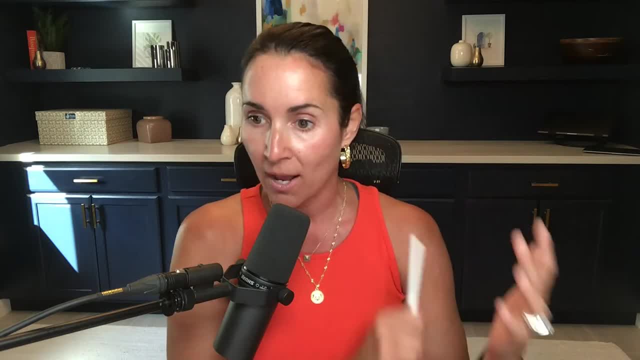 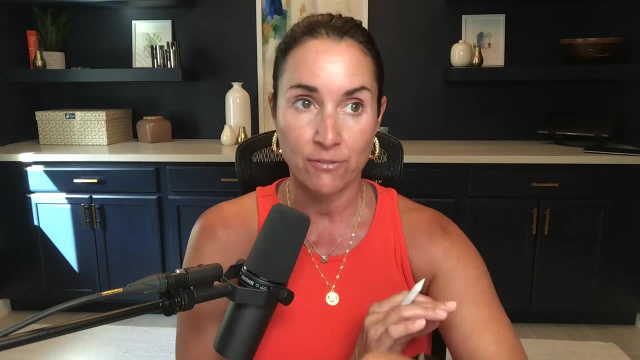 and Charles and Meredith and Jasmine and Elena and Mike and Tamara and a bunch of other people here. I'm so glad you're here. Thank you so much for joining. You're actually going to get an email after this is over. If you're joining on social, that's fine too. You can stay there or you can. 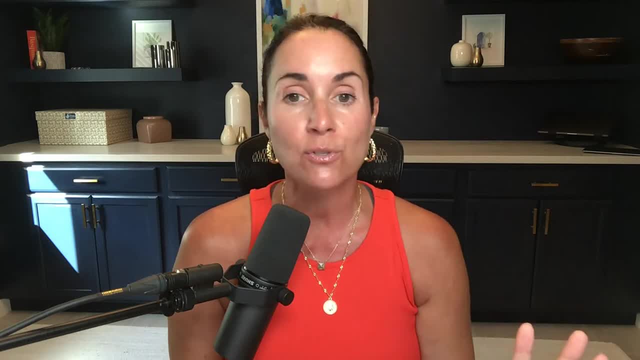 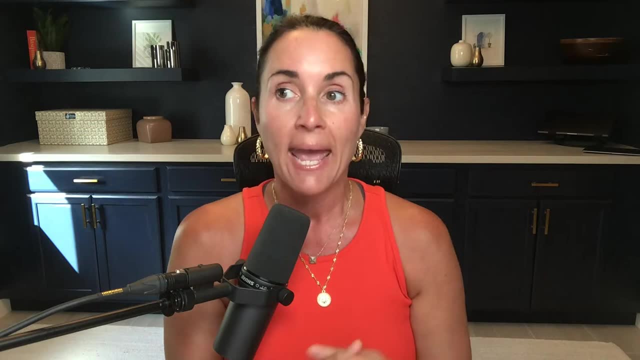 come into the webinar by clicking the link and just filling out the form. You can also do that later. Now, this did come with a free study guide for the Praxis 5001.. That's elementary education, and it doesn't matter if you couldn't download that right now I'm going to project everything. 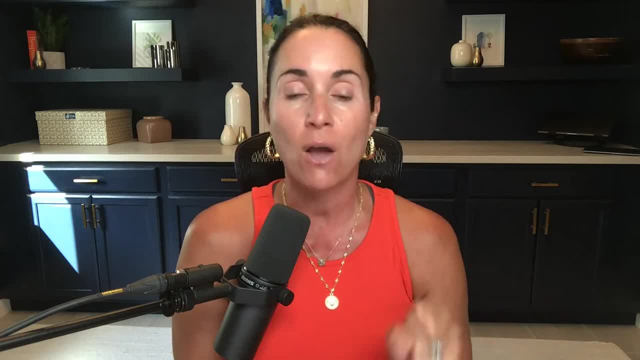 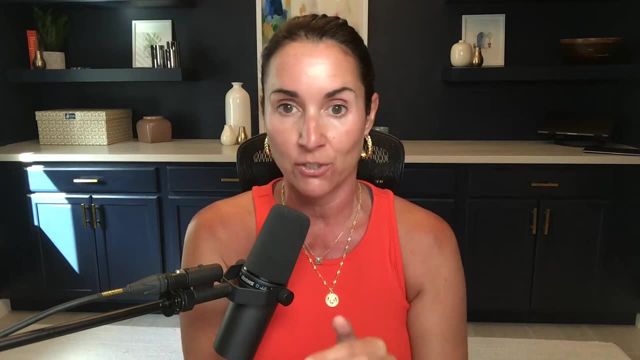 I talk about today on the screen, so don't worry about trying to print that out and have it in front of you. I've got everything on the screen. You're going to get the replay link when this is over so you can watch it when we're done at your convenience, and you're going to get everything. 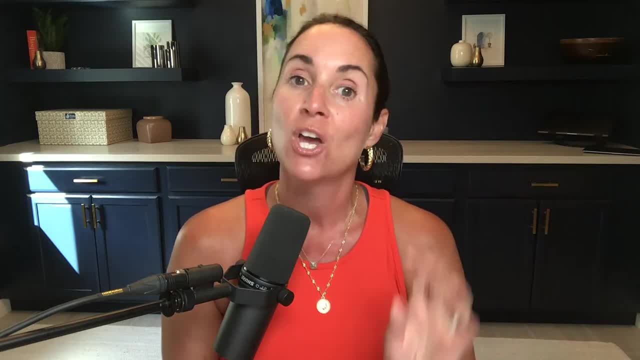 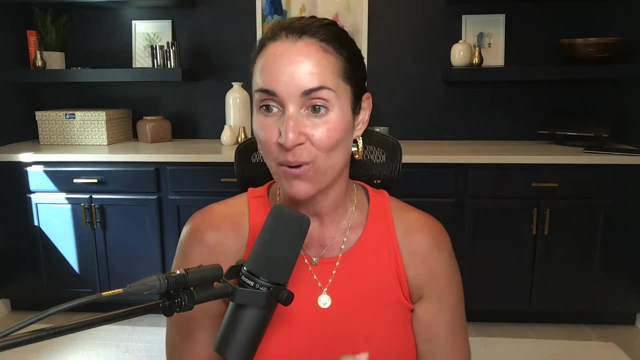 So just pay attention. today I'm going to be like the teacher in the front of the class. Don't worry about writing everything down, Just pay attention to the presentation and you'll be fine. So good morning everybody, So happy you are here. It is Saturday, March 16th, 10 am, 10 am and we are. 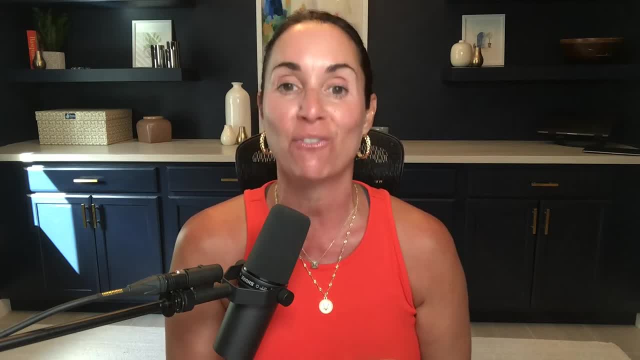 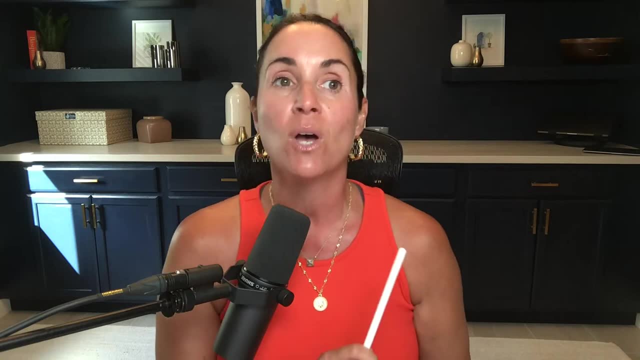 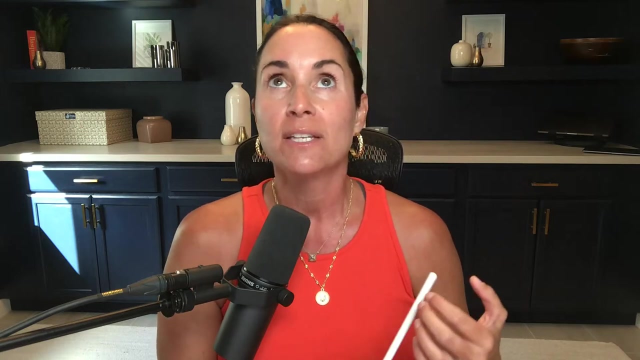 doing the Praxis. Elementary Education. Multiple Subjects: 5001.. webinar. Now, this webinar will help you, obviously, with the 5001.. It will help you with the 5901 also, which is another elementary education test. It'll help you with the 7811.. I mean, they're all kind. 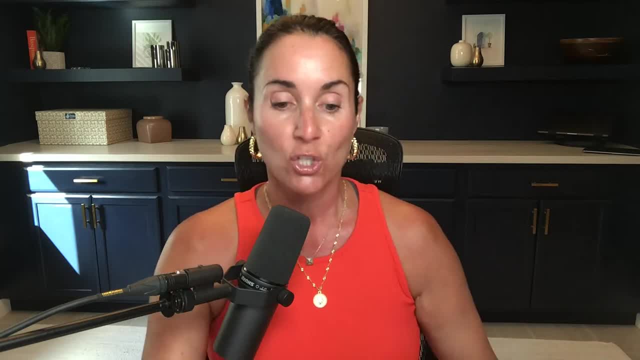 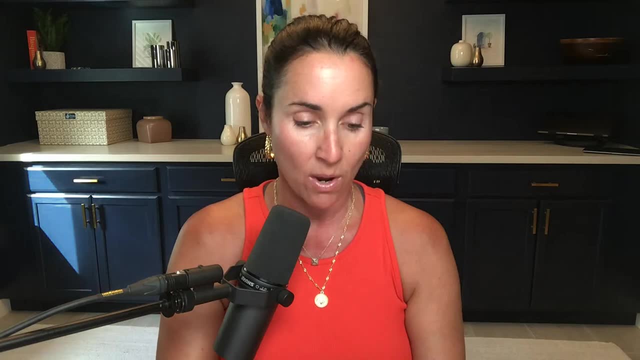 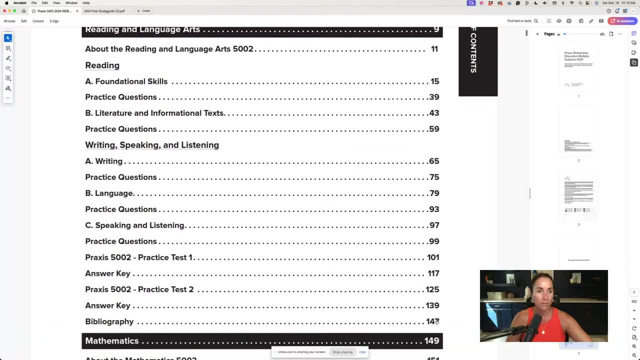 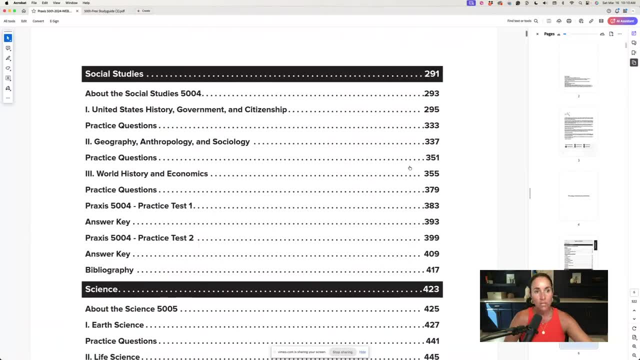 you know, it's kind of the same thing- Let me just fix my phone so my thing doesn't go off- And they all cover ELA and REIT. So you know, at each content category there are practice questions. So 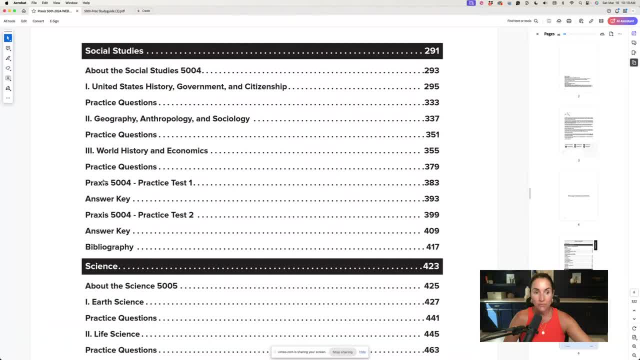 not only do we have the practice tests, full practice tests and practice questions, questions. so not only do we have the practice tests, full practice tests. you can see here for the social studies test one, test two. You can see here for the social studies test one, test two. 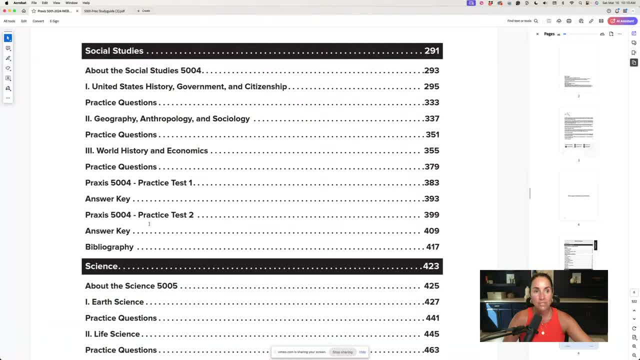 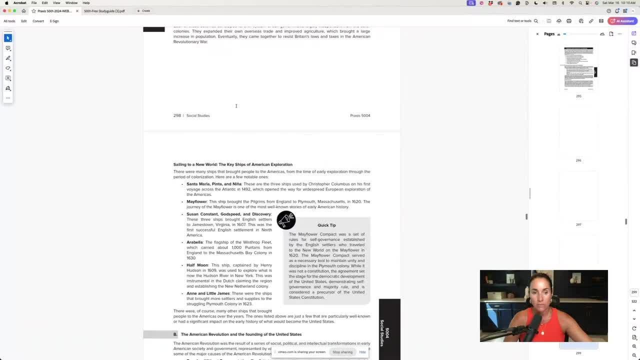 But after each section like this is United States: Your Gülems History, History, Government, History, Government and Citizenship. After each section like this is United States: History, History, Government and Citizenship. After each section. let me just scroll, just scroll here. 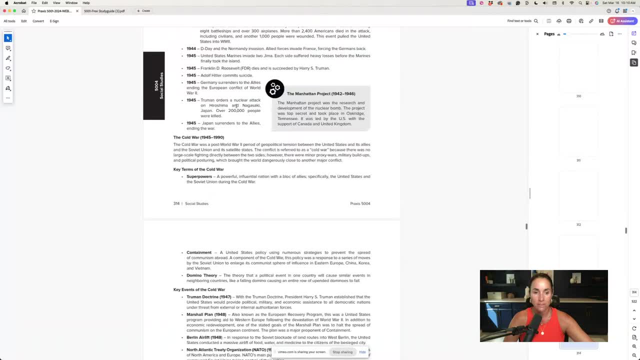 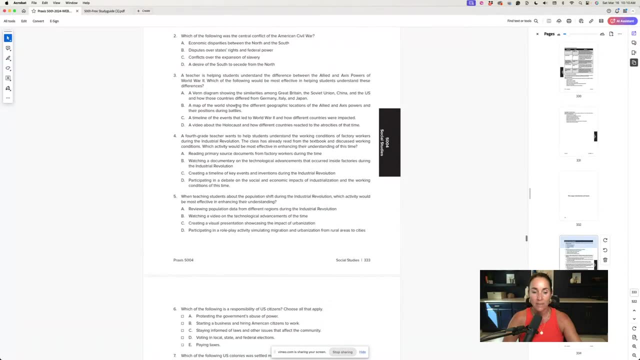 And I'll go back to in관 to women matter. just scroll here. Sorry making you dizzy. This is actually one of the biggest sections. Okay, Let's see There are 10 questions. There we go 10 questions just for that So you can see what questions would be like for that particular. 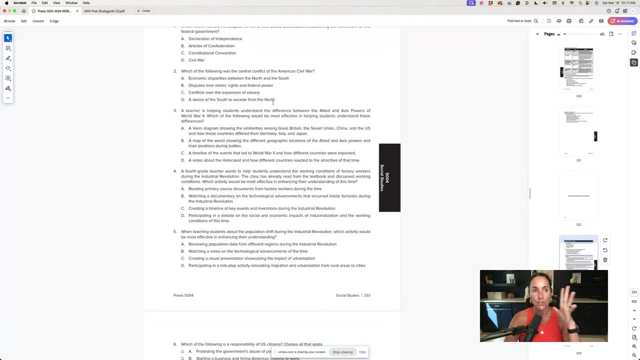 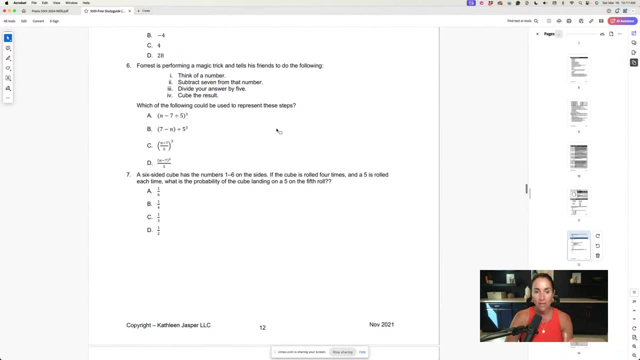 section, Cause each, each of these are broken up into sections and you're going to learn more about that today. I'm going to show you that, Okay, But today we're going to be working from this free study guide here. Definitely, check that out and make sure to read the answer explanations. 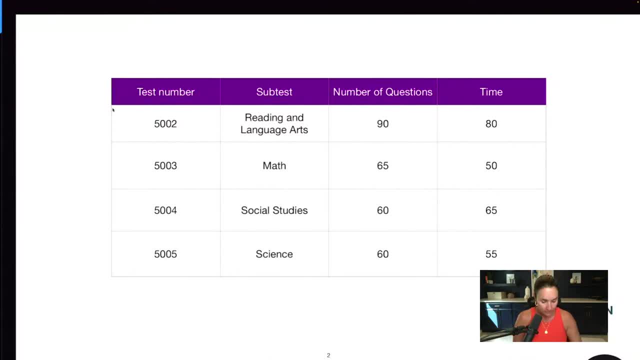 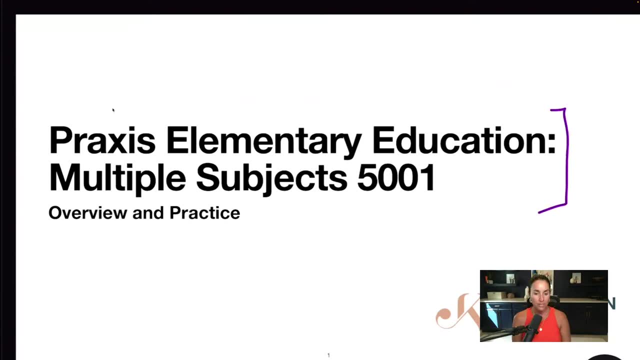 Okay, So let's go to my presentation and we'll get started here. So we are doing the Praxis Elementary Education 5001.. That's what we're focusing on today. I know a lot of people need lots of different tests. This webinar is for the 5001.. If you have questions on other tests, 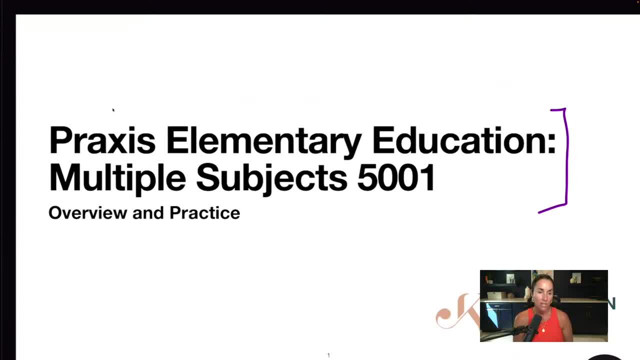 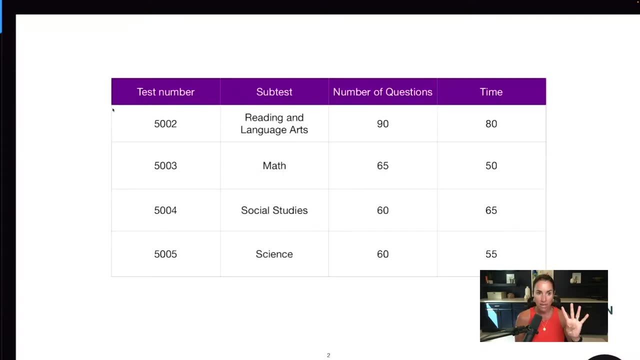 we're happy to help you. just email us at info at KathleenJaspercom and we will help you with whatever you need and we'll point you in the right direction. Okay, So we are focusing on the 5001.. All right, So when we talk about the 5001, there are actually four subtests, So the whole test. 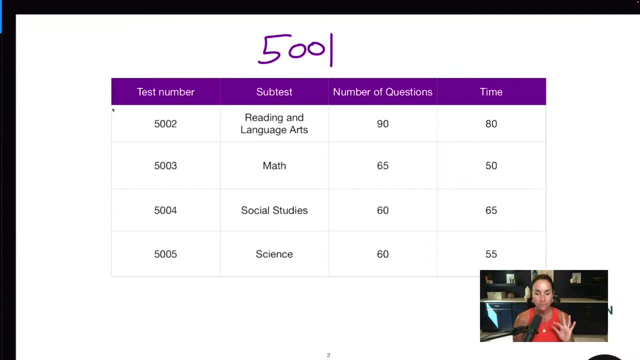 is called the 5001.. And this can be very confusing to people because, um, you know, it's like all these numbers- 5001,, 02, 03,, 08, 5354, you know, they all have these. 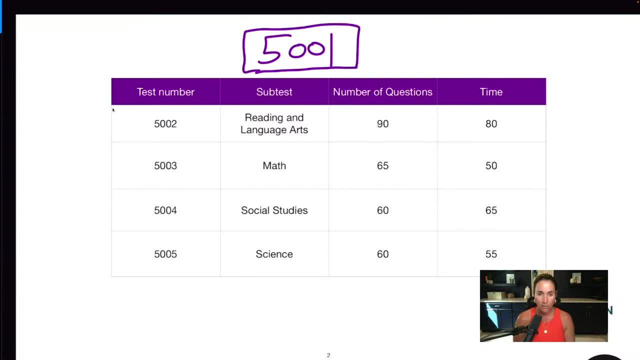 different numbers. The 5001 is the whole entire test but it's broken up into these three subtests, So the 5001 is called the 5001.. And this can be very confusing to people because you know it's like all these numbers- 5001,, 02, 03, 08, 5354, you know they all have these. 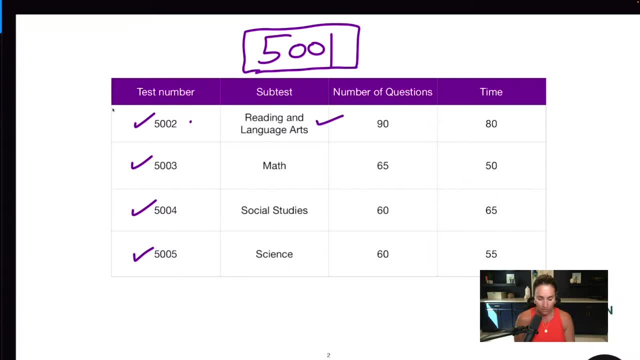 different numbers. So when we talk about the 5001, there are actually four subtests: The 02 is reading and language arts, The 03 is math, The 5004 is social studies And the 5005 is science. 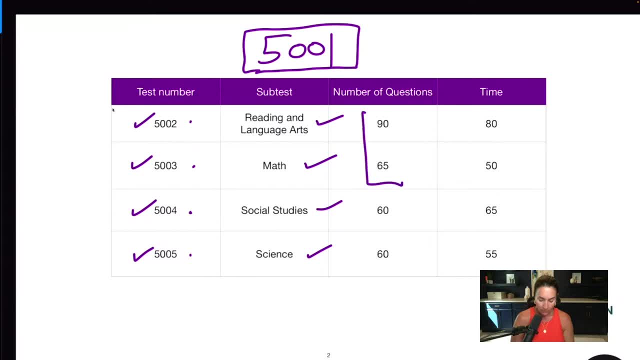 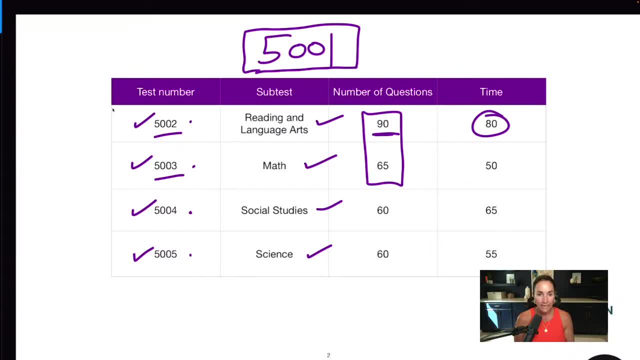 You are a reading teacher first and foremost. You can't teach social studies, You can't teach science, You can't teach anything without those reading foundations And arguably you can't even teach math either, because there are a lot of word problems in math. Now, a lot of math teachers would 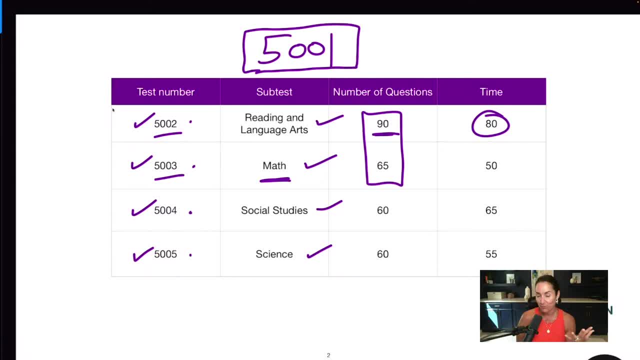 disagree with me. They would say- and I know this because I was an assistant principal and I worked with lots of math teachers- Math is math, Reading is reading, And you are correct. However, having the foundations of both math and reading is very important when we're teaching social studies and 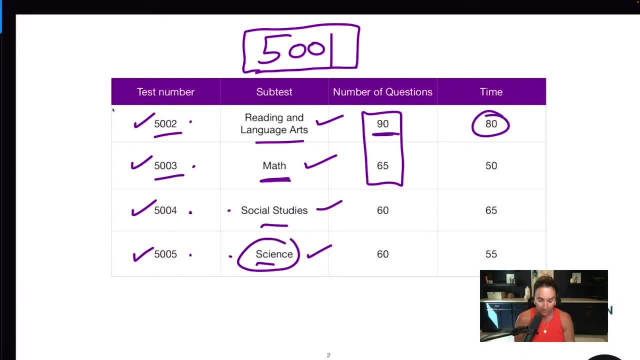 science. There's a lot of math and reading. There's a lot of math and reading. There's a lot of math and reading. There's a lot of reading. in both social studies and science There's math and science. You know, all of these subjects are interdisciplinary, They kind of intermingle. 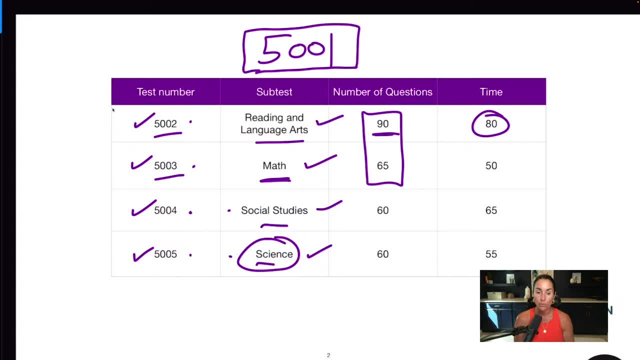 especially in the elementary grades. So we want to make sure we have teachers who are very well trained in these areas. The thing about the reading and language arts subtest is that it's got a lot of teaching scenarios And remember I always talk about working backward on those. 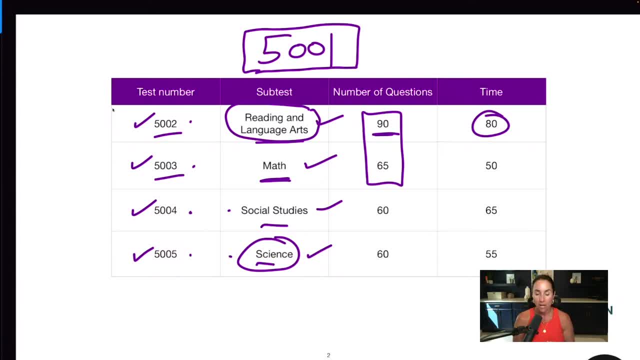 particular questions. I have a lot of videos. I have a lot of videos. I have a lot of videos on test strategy And we're going to hook that up in the email we send out to you guys today for this particular webinar And I will send you to that test strategy playlist And that's going. 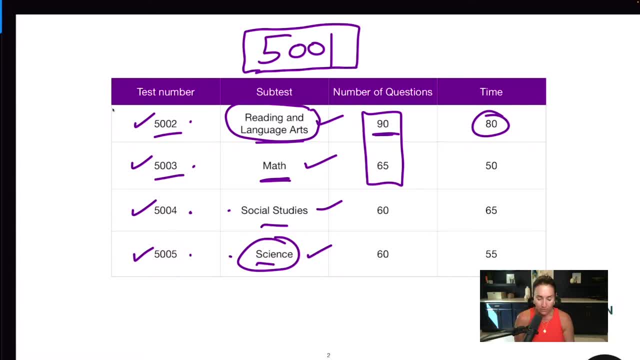 to show you how to work backward, how to find key words, especially for the reading and language arts. This one's a really good one to use those strategies And I'm going to show them in context in just a minute. And then the math as well. Very difficult, People are like. 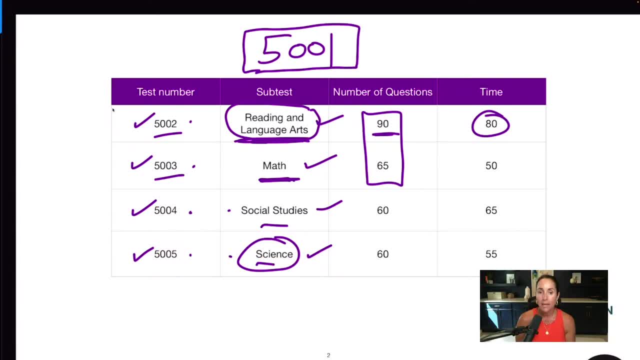 it's elementary math. How hard can it be? Very hard, actually. I would challenge anybody who thinks that this is an easy exam to take it, And I will tell you that there's only a 50% pass rate on many praxis exams. So those who are saying, oh, it can't be. 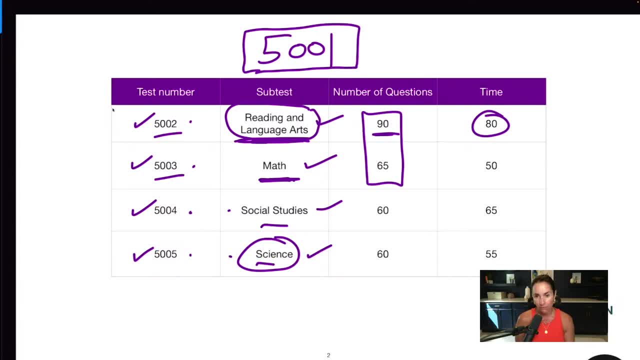 that hard, Okay. Well then you take it after not seeing math for 20 years or something like that, Because I know a lot of you are career changers. You haven't seen some of this math in a long time, But it is part of the elementary education curriculum, So we need to be proficient in. 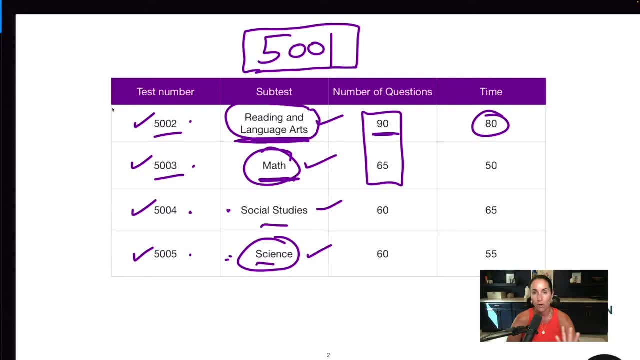 that area, The social studies and science. for this particular exam there are not really any scenario questions about teaching social studies and science. It's more about just those particular content areas. So it's a lot of memorization. Now, here's the thing People will say: well, 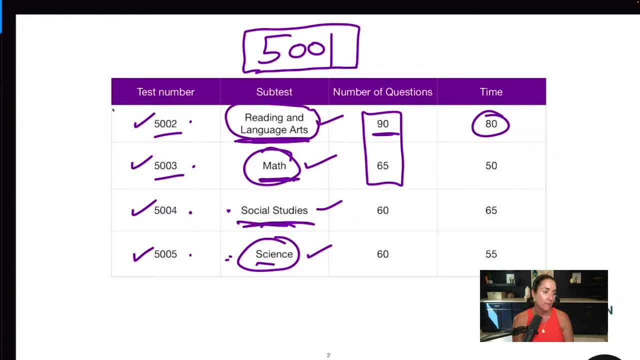 I took the social studies exam And not very many of the questions in the study guide were on the exam. Well, first of all, social studies covers a very wide range of questions And I have no idea what test you're going to get. I don't know what questions you're going to get. I do my best to. 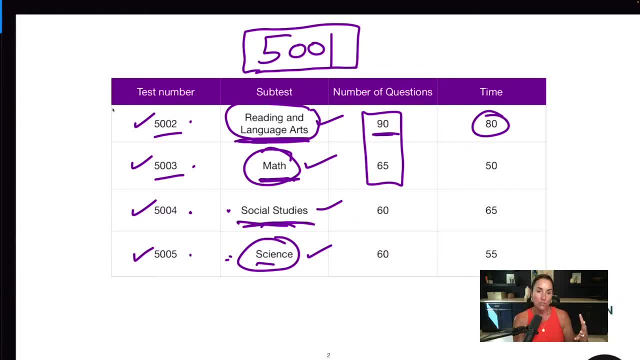 structure, the study guide. So they have a lot of questions And I have no idea what test you're going to get. But if you just look at US history, there are a million things they could ask you about US history. That's why it's really important to read the information. 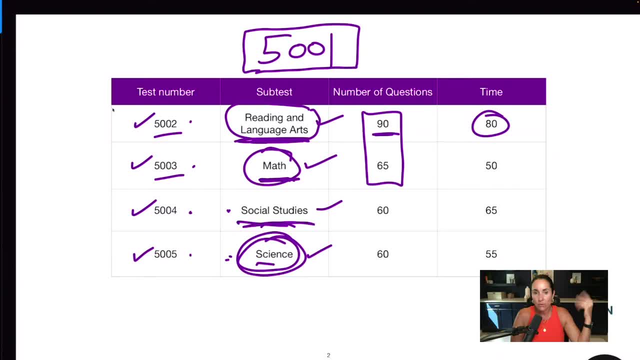 to understand. you know, like life science, There's a million different questions that can be asked for life science, from cells all the way to ecosystems, animals, respiratory systems, circulatory systems, I mean, the mitochondria, I mean there's so many things that can be asked. 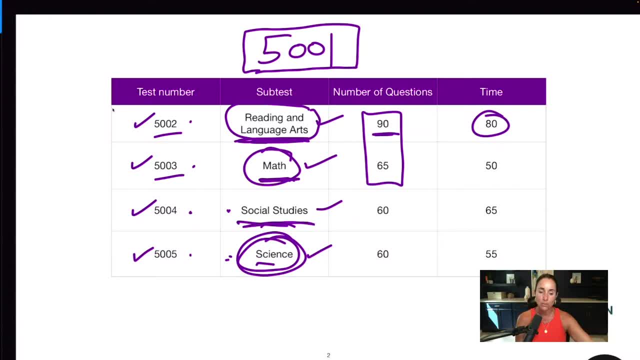 That's why it's so important, And I have no idea what test you're going to get, And I shouldn't know. It's a state-standardized assessment. Nobody knows what questions you're going to get, So trying to memorize your study. 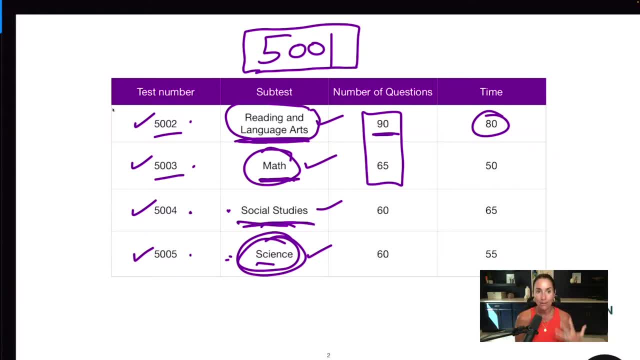 guide test questions is an exercise in futility. I would recommend actually learning the information so you are ready to go on testing And you can see. these are slightly smaller tested areas And you have about 65 and 55 minutes for each of those. All right, So let's go ahead and start. 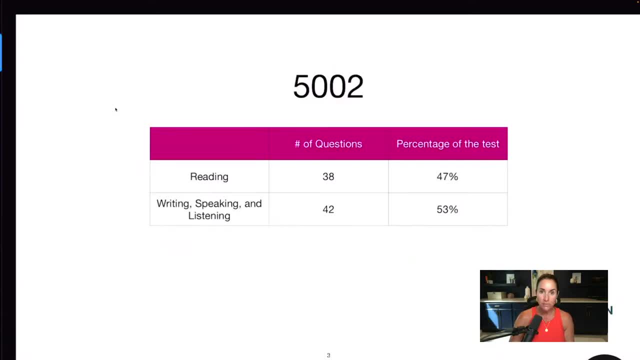 with 5002.. This is the English language arts section. Some people would say this is the hardest section Depends. I think the 5002 and the 5003 are the hardest in my own opinion, But of course everybody's different. So for the 5002, there are actually two main content. 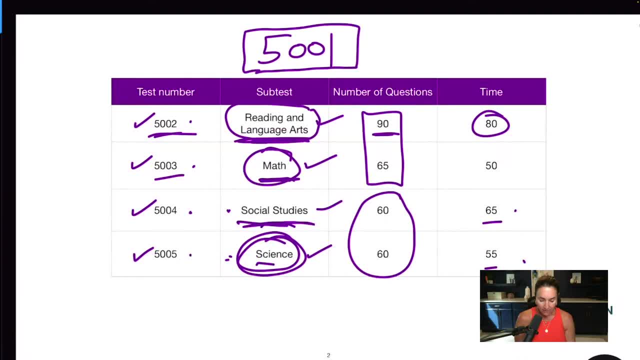 categories. So here's how we look at it. These here- the 5002, the 5003,, 5004, and 5005- are referred to as subtests. There's a reading and language arts subtest, a math subtest, a social. 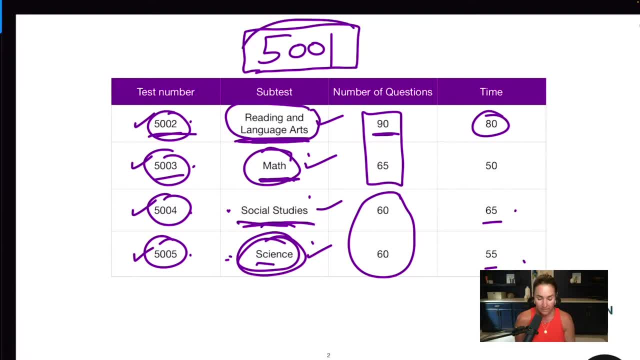 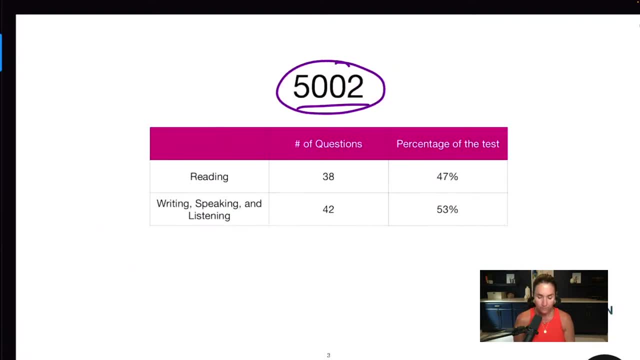 study subtest and a science subtest. The whole test is the 5001.. These are subtests Now within the subtests. so the 5002 is a subtest. there are content categories inside the subtest. So for the 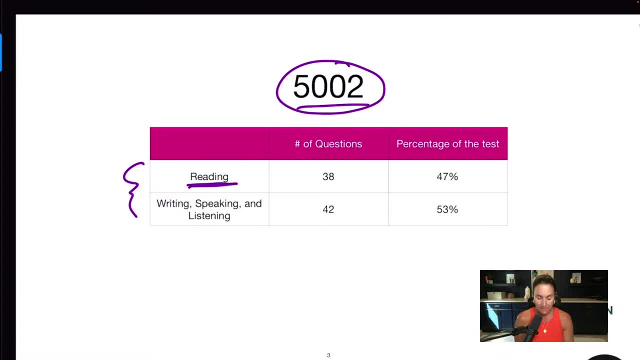 5002, reading and language arts. there is a reading section, I'm going to tell you, and there's even more topics in that, And there's a writing, speaking and listening section. And you can see the reading section is 38, and the writing, speaking and listening is 42. They're pretty. 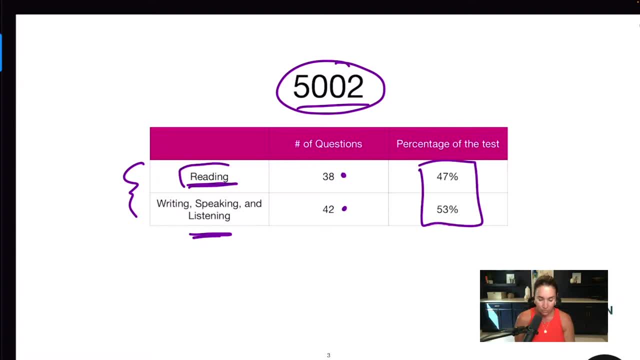 much evenly split. But you can see here reading is just one content category, one subject: Writing, speaking and listening is three. So arguably there's more reading questions than anything else, because 38 comes straight from reading. 42 is split among three different things here Just. 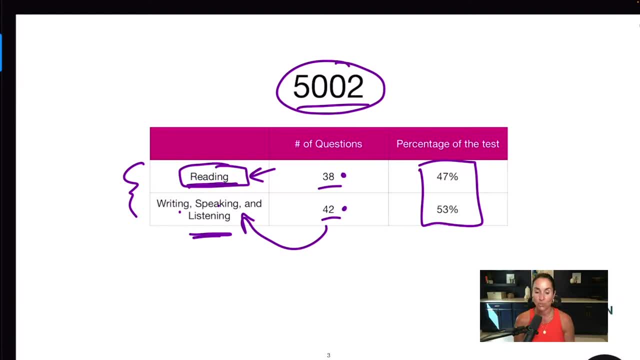 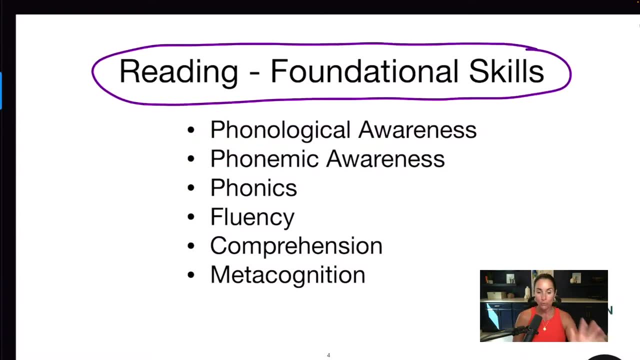 getting a little technical there. But for the most part for the 5002, you are going to want to really be schooled in the foundational skills of reading. Now I'm going to go through a lot of them here today. In the 5002 online course I go into them very 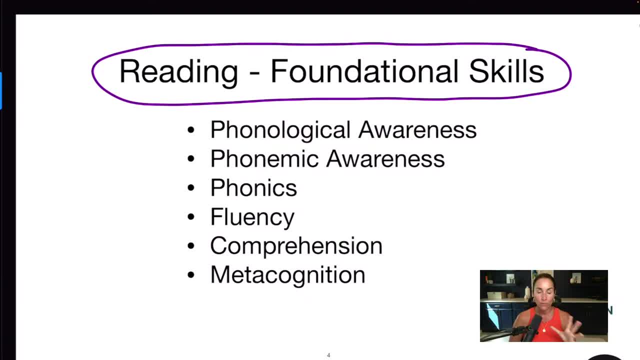 intensely, And also I have a reading playlist on my YouTube channel that goes over this as well, And again, we'll link that up in the email that I'm going to send out with you today once you finish the webinar. So these are the things you really need to know in order to do well on the 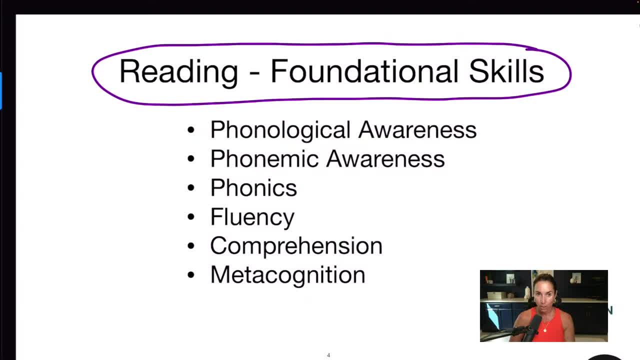 5002.. Because as an elementary education teacher, you have to understand well what's the difference between phonological and phonemic awareness, What's the difference between those and phonics and fluency and comprehension and metacognition. You will get questions on these particular topics. 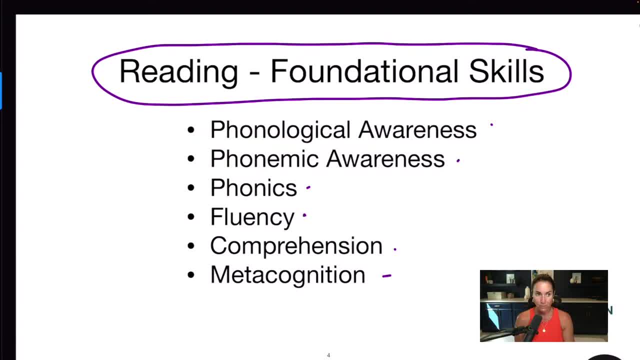 all right. So let's break them down really quickly. Of course, I have more information in a more in-depth courses and things like that, But let's give them a quick rundown here, All right. So phonological and phonemic awareness I want you to remember are sounds: 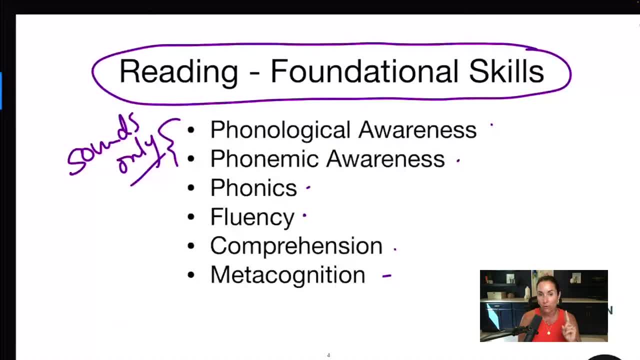 Only Okay. Phonological and phonemic awareness. I know they kind of run together and they sound a little bit like phonics, But these two here are sounds only. We are working on our listening and speaking skills. You do not have to see the word in order to have phonological and phonemic. 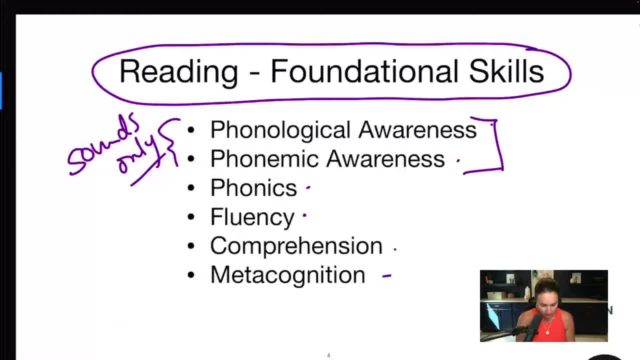 awareness. So, for example, let me see what's my next slide here. Okay, I just wanted to make sure- Is breaking words up by large chunks of sounds in the words, And phonemic awareness is small chunks, So let me do large, small, All right. So let me give you an example of phonological 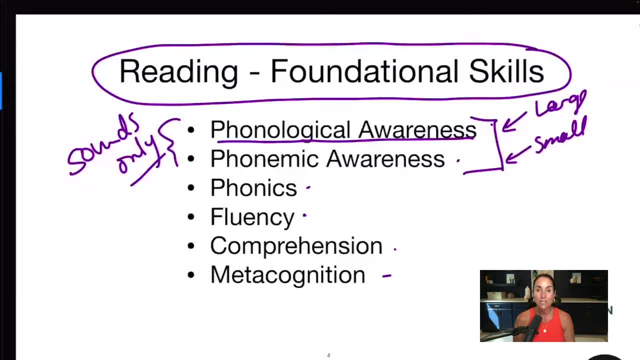 awareness. I might have you break up the word by syllables, For example something like rabbit- All right, Rabbit, That's two sounds, Rabbit, Right. I might have you break it up by onset and rhyme. The onset is the beginning. consonant or consonant? 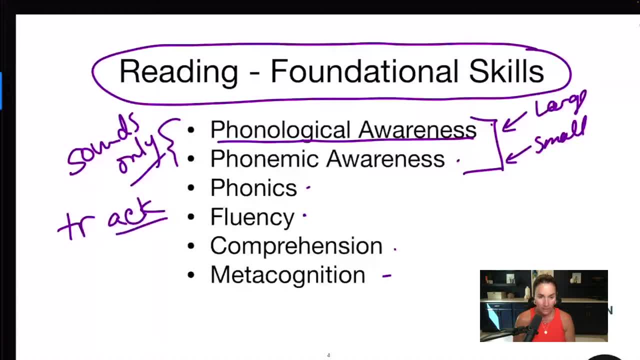 cluster And the rhyme is the ending vowel and consonants. So if I said to my class, break up the word track by onset and rhyme, they would say ter-ack, Ter is the onset rhyme and it's spelled: R-I-M-E is the 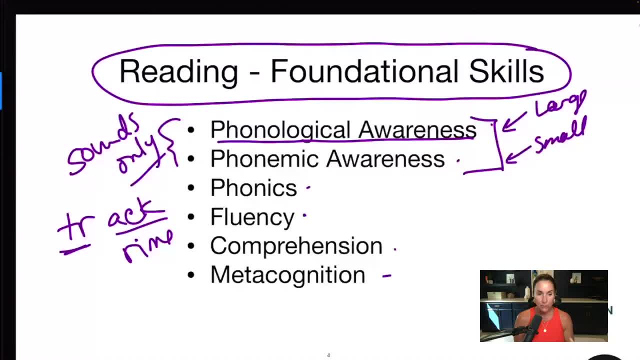 Ac is the rhyme. So those are bigger chunks of words, right Syllables, onset and rhyme. We might do compound words. They're large. That's phonological awareness. And again, I don't have to see the word. I wrote the word here for you guys, because I'm trying to show you what an 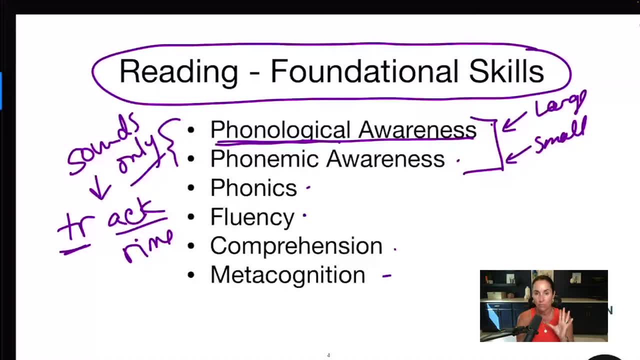 onset and a rhyme is. But you don't have to do that with phonological awareness, It's just listening. You just say to the kids: all right, how about the word stop? Break it up by onset, And the kids would go st And I would say, okay, what's the rhyme? 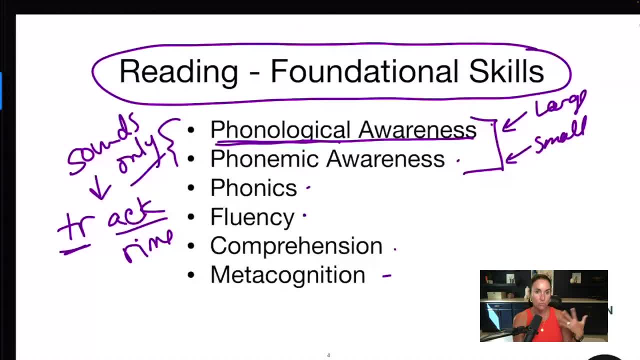 And they'd go up. They would know that because these are exercises we do, We teach this explicitly, systematically and recursively, So kids know how to do this. This is like all in the elementary grades. okay. Now phonemic awareness is a little more nuanced, a little. 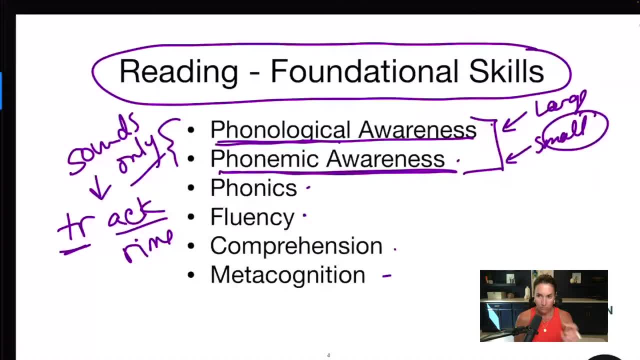 more complex. These are the small, small pieces of the word And this is the individual sounds in the word. So if I was going to break up the word track by phonemic awareness, I would do it like t r a k or the k sound. Notice that that's four sounds T r a k? Much different. 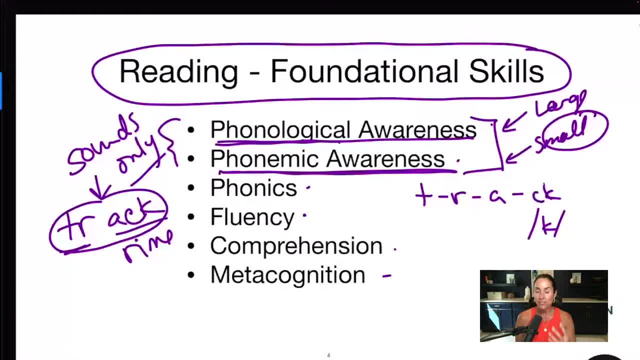 than ter ak right. So it's all about the sounds and words. We are teaching students this. These are foundational skills. They have to have phonological and phonemic awareness before they can get into phonics. Phonics, you have to see the word Phonics is. when I look at a 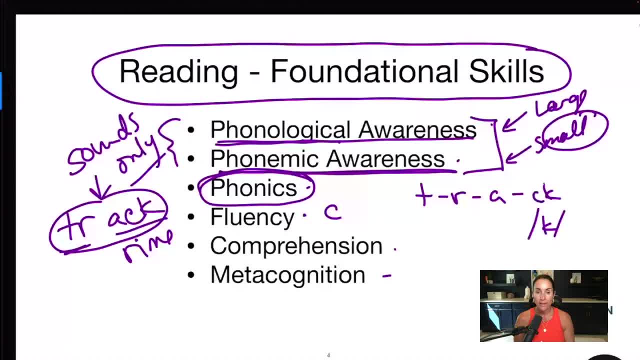 C, and I determine whether it makes a k sound or a s sound based on what it's followed by. If it's like this, I know that C makes a k sound because it's followed by an A, But if it's followed by a Y, I know it makes a s sound, as in cycle. Now, how do I know that? Well, 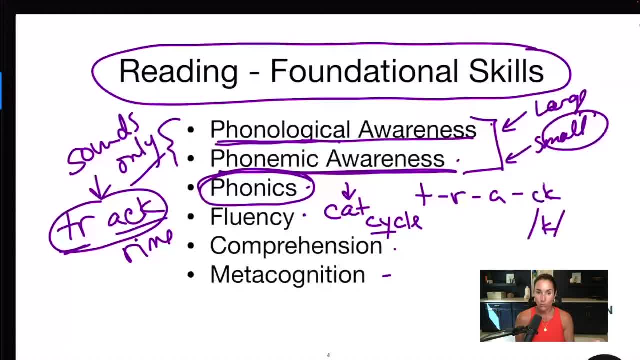 we teach students phonics Rules, And one of the rules- and there are many in phonics- is that when a C is followed by an A, O or U, it makes a k sound. When it's followed by an E, I or Y, it makes a s sound. When a P, 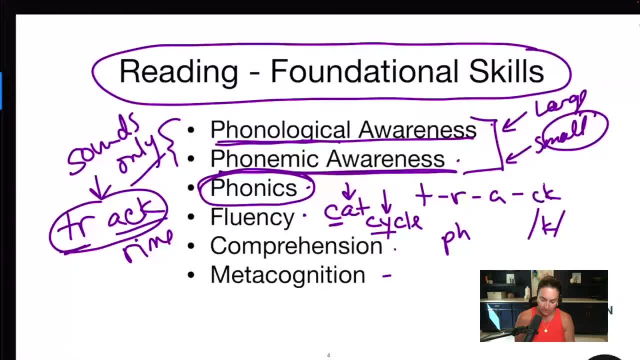 and an H are together, they make a f sound. How do I know that? Well, because I taught the students phonics. Now, before I can have phonics, I have to have phonological awareness and phonemic awareness. And I have to have phonological awareness and phonemic awareness And I have to 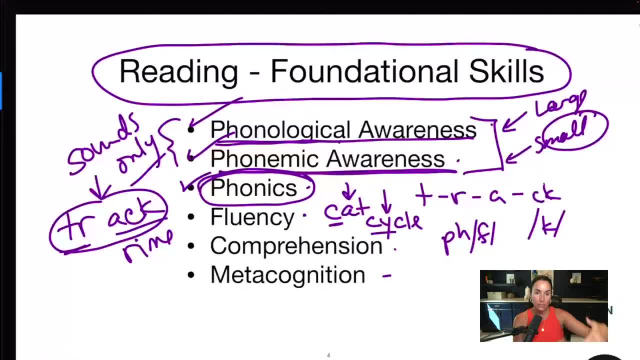 have phonological awareness and phonemic awareness. Then I move into phonics. actually, looking at the word Notice, there's a system. This is all systematic, explicit. We teach these skills in isolation and we also build on them in a systematic manner. So the words quick tip here. 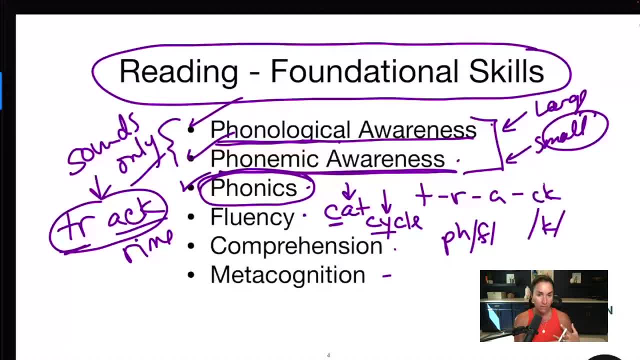 explicit, systematic and recursive are good words on this exam. If you see them in an answer choice, it's probably the right answer. Well, explicit, we know. We teach explicitly each individual thing. We teach explicitly each individual thing. We teach explicitly each individual. 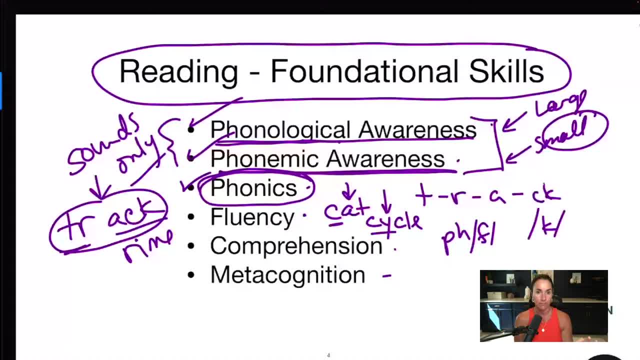 thing. We model, We go over it, We beat a dead horse. explicitly Systematic is we go by, step by step. First we do phonological awareness, Then we do phonemic awareness, Then we do phonics, Then we do fluency. We have a step-by-step process. Recursive is when I go back and I say: all right, 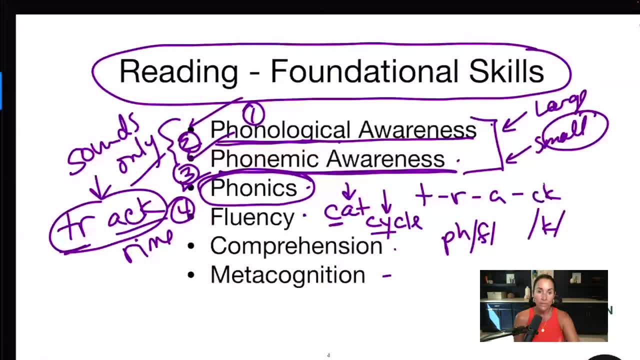 guys, we need to review our phonemic and phonological awareness so we can get better at this more complex phonics skill. It's when we go back to go forward. basically That's recursive. So explicit, systematic and recursive are all good words. 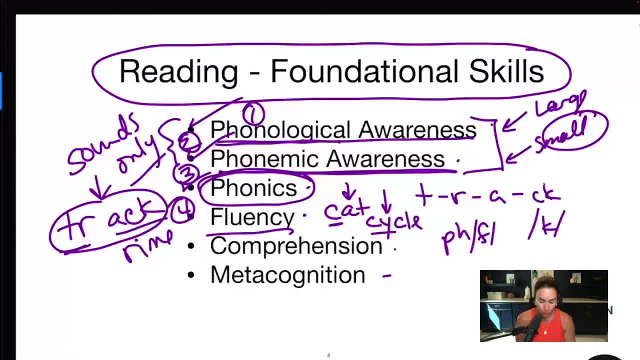 Next step is fluency. That's when students move from just decoding words in phonics to actually reading strings of words, sentences, paragraphs, right. And we need students to increase their fluency because without it they can't have comprehension, And fluency is the bedrock. 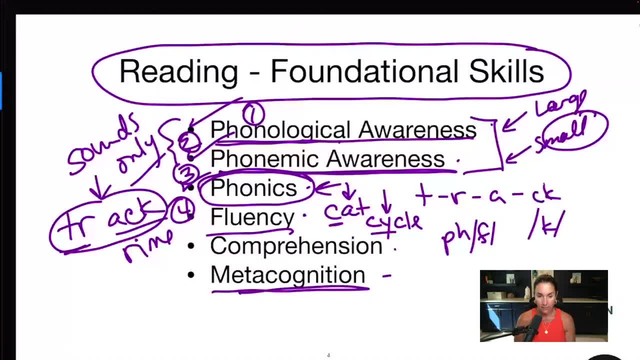 of comprehension because of a little bit of this metacognition- I'll talk about that in a second- And also their cognitive endurance. When students have fluency, they're moving through the text at a good pace. They're automatic, They're reading things. 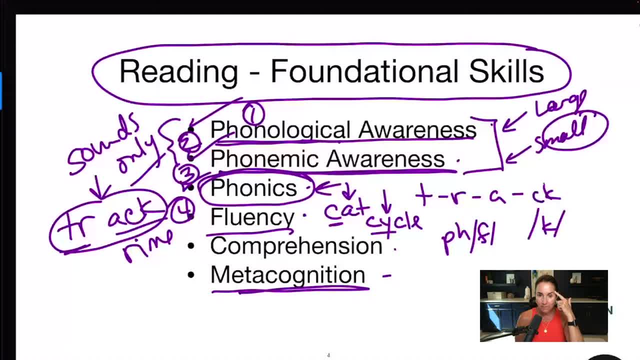 accurately. That frees up cognitive demand, cognitive energy that they can then use on comprehension. If you're watching a kid sound out every single word of a passage, you know that is exhausting and they're not comprehending it. They're decoding, They're. 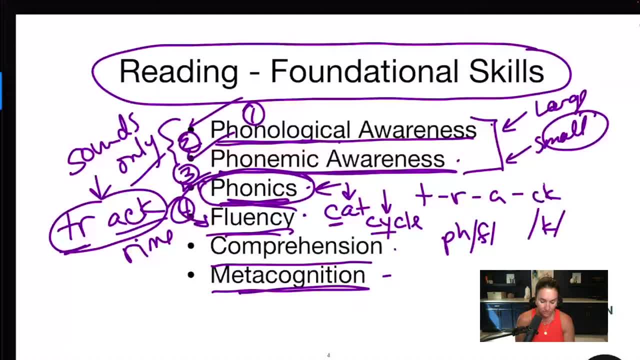 using phonics and not fluency. So I moved from phonics to fluency, fluency to comprehension, and then metacognition goes with comprehension, because metacognition is thinking, about thinking. That is when we model our process as teachers on. 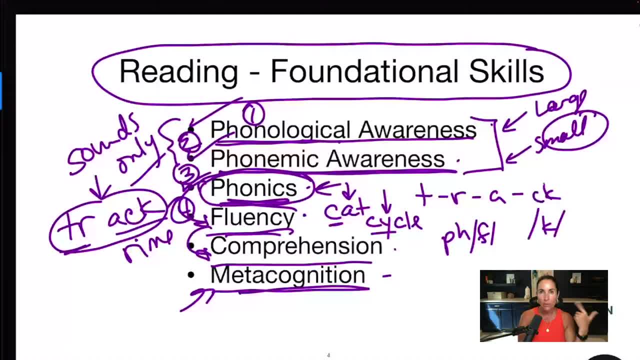 how to figure out words, how to understand words, predicting going. hmm, I wonder what's going to happen next. Oh, I know how to sound out this word. Let me use the words around it: That process of trying to figure things out. we model that for students. That teaches them metacognition. 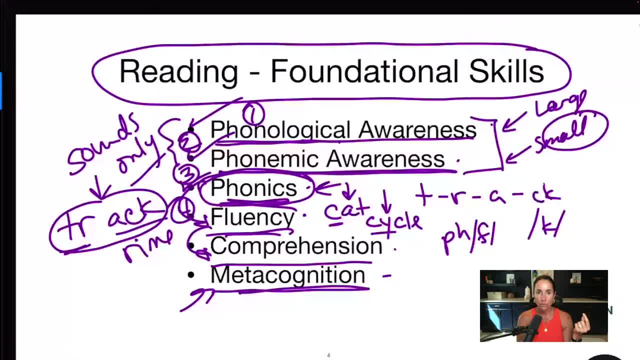 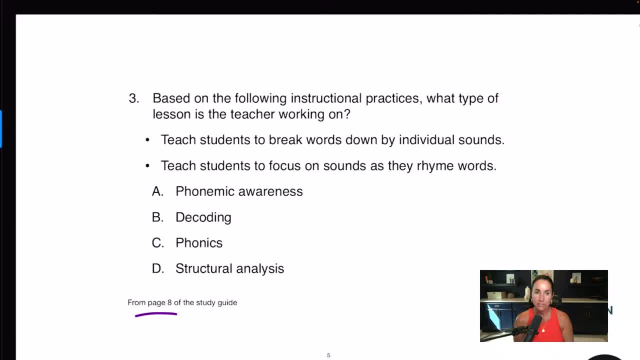 thinking about their thinking. How do I use my brain to figure this thing out? All right, And that's really important. All right. So let's have a look at what a question might look like. This is number three from page eight of the free study guide. Of course, I'm always going to work. 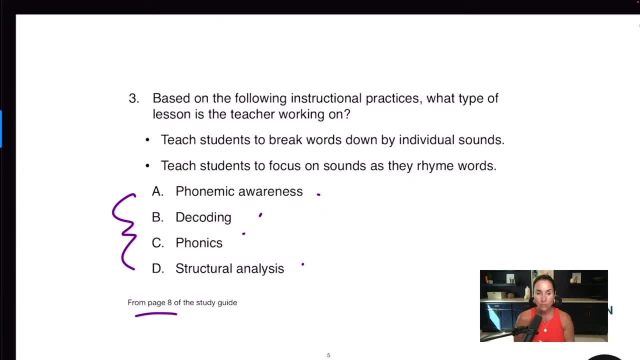 backwards here And I could see I have skills here. Can't do much about that, But here's a quick tip: Decoding and phonics are the same thing And if it's asking for just one right answer, you can't have two of the same thing in the answer choices. right If there's only one. 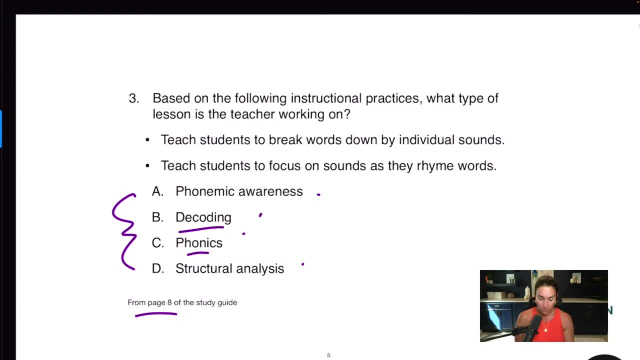 correct answer. two of the same thing is incorrect. So just thinking like a test maker- and I always do- is to think like a test maker, And I always do, And I always do, And I always say that: Think like a test maker, not a test taker. Want to cross off B and C? All right, 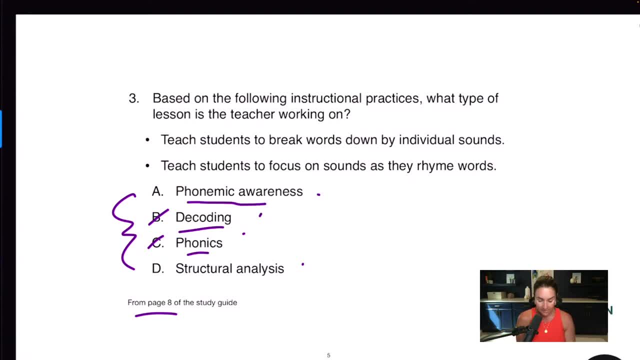 Because they're the same thing. Now, phonemic awareness is sounds only And structural analysis is sort of a phonics skill. I'll leave it because it's not explicitly phonics, But phonemic awareness is standing out here. Let's have a look at the bullets: Continuing to work. 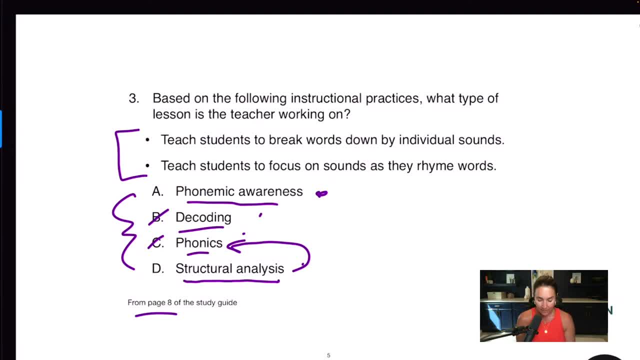 backwards. Remember, always work backwards. Teach students to break down words by individual sounds. Teach students to focus on sounds, Sounds, Sounds. What did I say before? Phonemic awareness and phonological awareness are all about the sounds in words, Decoding and phonics. 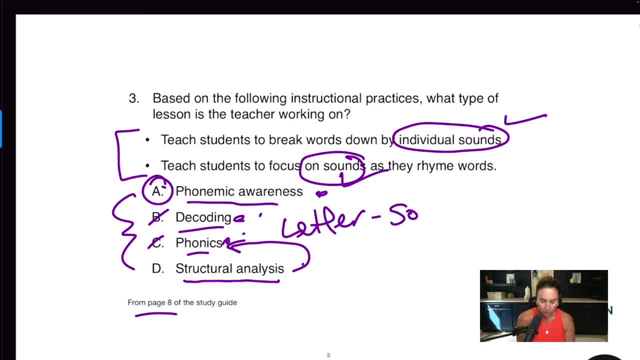 are letter-sound correspondence. You have to see the letter to understand the sound, like in cycle right. I have to see the C and then the Y to know it makes a sound in the beginning. But with phonemic awareness I don't do that, I'm just paying attention to sounds. Looks like A is my 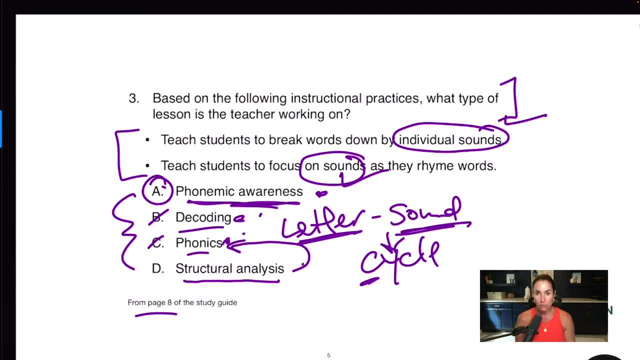 correct answer. Let's have a look at the question Based on the following instructional practices. what type of lesson is the teacher working on? Okay, Just fluff. They are really the important part. are these bullets here- And I know it sounds only Structural- 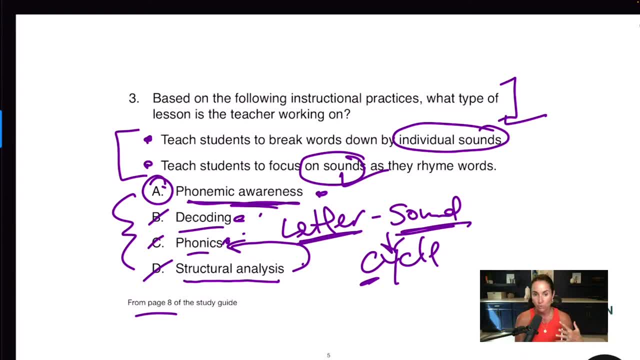 analysis is breaking up words by prefixes, suffixes, roots, Also compound words. Structural analysis goes with morphology And morphology is phonics. So really B, C and D are all the same kind of skills, So we could cross those off because we're only being asked for one, correct? 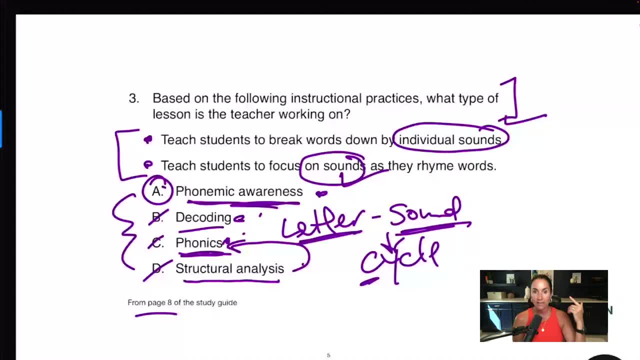 answer And A is the one that stands out. That's just a way to think. like a test maker, I study and I see patterns, And it's important that you think like a test maker, not a test taker. I say that all the time. It's going to help you, because you're not going to know the answers to all these. 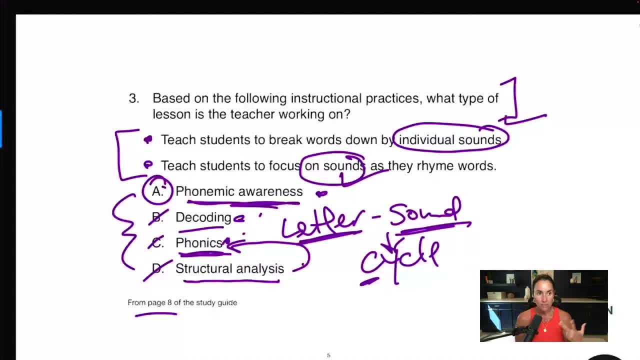 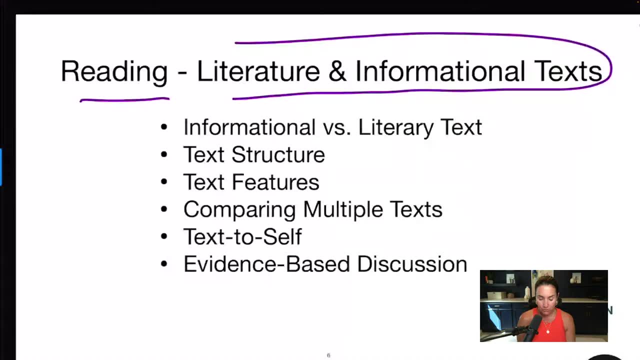 questions, You're just not. But these kinds of ways and working through them will help you be more strategic. All right, So then we get into reading of literature and informational text. This is also called a balanced literacy program, where we use literature and informational text. 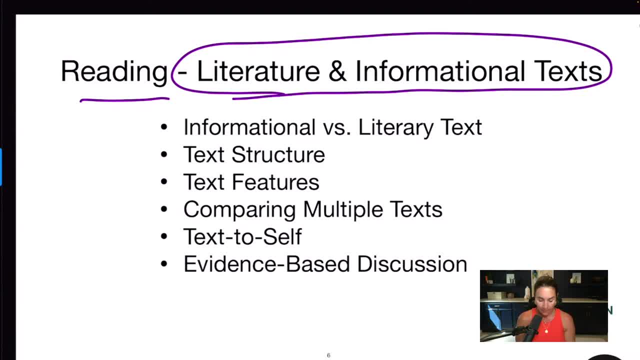 Very important that we're using both, And you can see I have that Informational versus literary text. We're going to focus on text structure. Is it cause and effect, Is it chronological, Is it argumentative, Is it expository, Is it a narrative? And then, of course, text features. 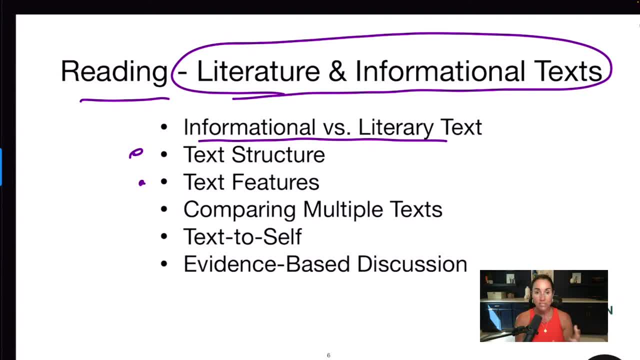 the index, the headings, the graphs, and teaching this to students at a very young age as well. When they hold a storybook, they know the front cover, They know the table of contents, They know the page numbers, Just to keep you in the loop, And then we can work around this. So this is 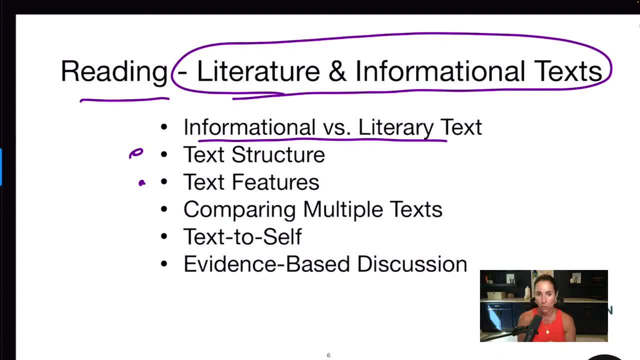 teaching them how to use the book is very important, especially in the early early grades. then, as we get up into more comprehension and critical thinking, we're comparing multiple texts- another good word. we want students to look at one piece and look at another piece and be able. 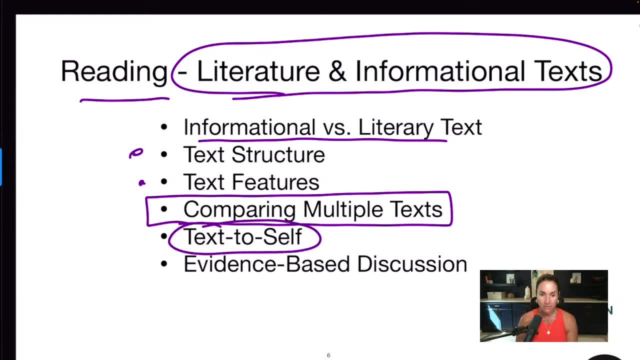 to make connections. this is also a really good word text to self. we want students to be able to see themselves in text and say, hey, how do i relate to this character, how do i understand this character? what do i know about this in my own life? very important text to self, and then of 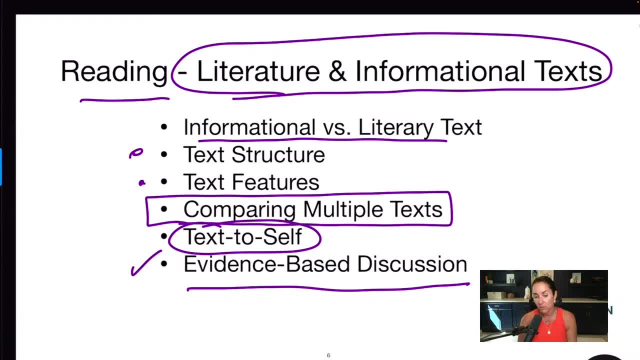 course, evidence-based discussion is a big part of the common core standards in english language arts, and it's all about requiring students to use evidence from the text to support their claims. so, for example, if a student says, uh, this person did this and that was blah, blah, blah and they 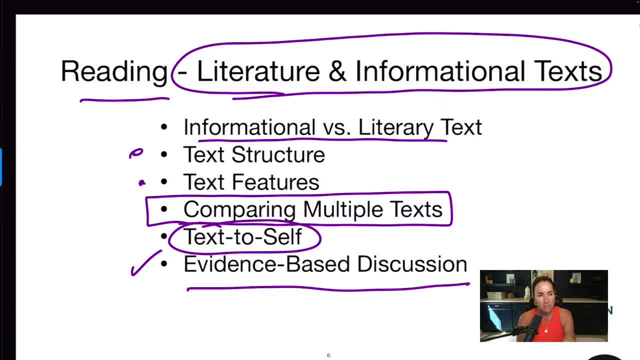 say something and you're like, oh, that's a really good observation. where in the text did you get that information? or what in the text led you to that belief? can you show me a page number? can you put your finger on it? that's the beginning stages of teaching students how to cite text. 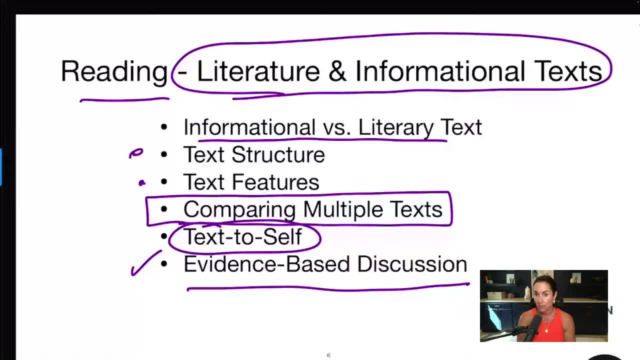 because starting at about fifth grade, sixth grade, seventh grade, all the way up through college and career, they're going to have to cite that information properly, using, you know, the author, the date, depending if they're using apa or mla, and then these skills that we're 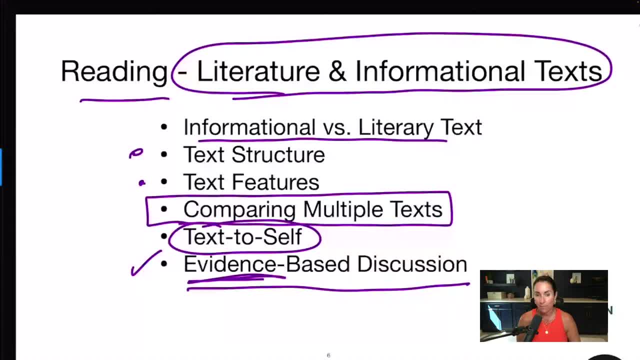 teaching them early on. where did you get that information? where did the author say that? what page number was it on is the start of that kind of skill which is really, really important? okay, you can have an opinion, but we need to know where in the text does that? 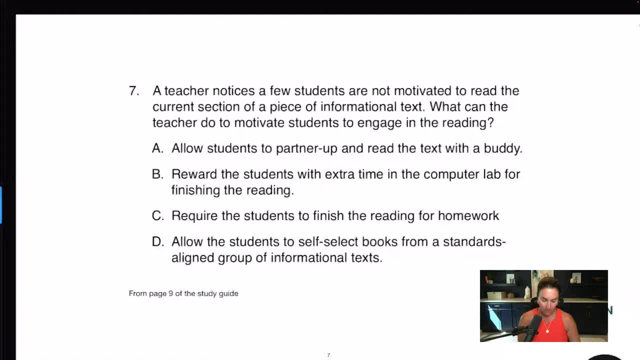 support your opinion. all right, so let's have a look at what that might look like on the exam. okay, and we're here again. this is what i call a scenario question, where we have a scenario here and all the answer choices are scenarios, and a lot of times students will say: well, all the. 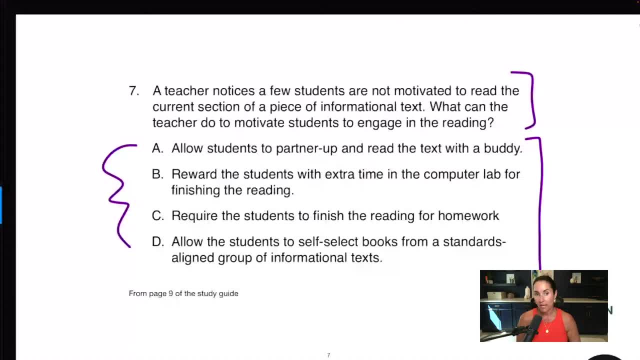 answer choices looked good. they'll they'll email us and say, hey, i. i think every answer could be the right answer, and this has to do with a couple of things. number one: uh, you're brand new to teaching, so you don't know some of these smaller nuances that you need to be on the lookout for. 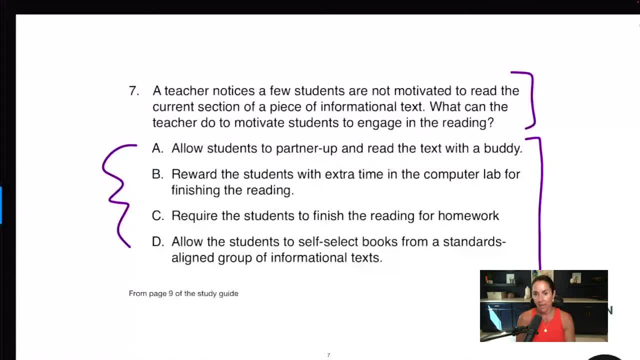 and number two, you're not paying attention to the good words and bad words in the answer choices, so this one's a good one to do that with. so i'm going to start with the answer choices. first, allow students to partner up and read the text with a buddy. okay, now if i'm a new. 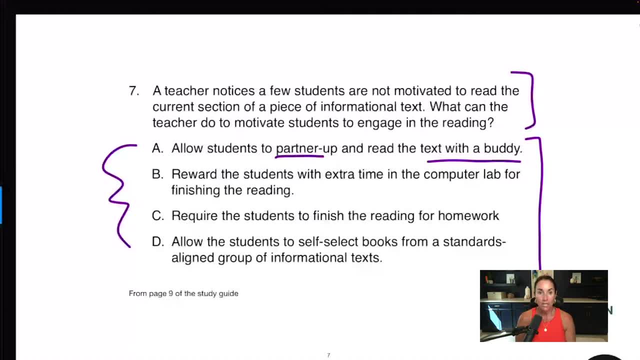 teacher. partnering up and reading with a buddy sounds good, and i might say, well, that that sounds pretty good. it's cooperative learning. i'm going to leave it. okay, it's okay. it's not great. it doesn't say what they're going to do. it doesn't say how it's going to be structured- cooperative. 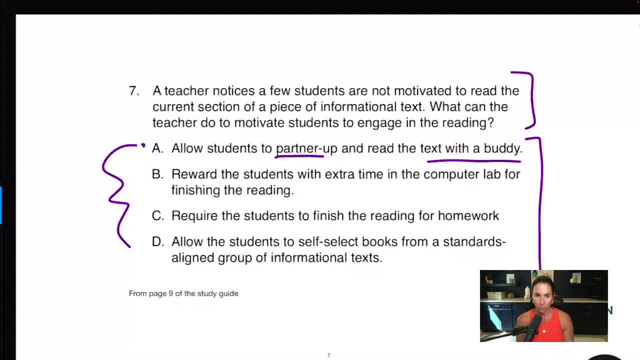 learning is very good, but this has like no structure to it. what are they going to do? partnering up, what does that do? so i? i don't hate it, but i don't love it. b reward the students with extra time in the computer lab for finishing the reading. now, if you're a new teacher, you might say: 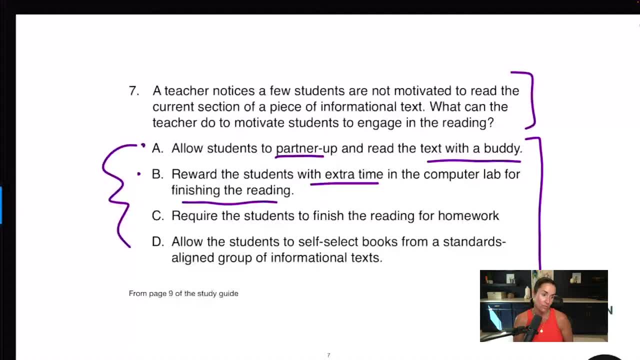 well, yeah, of course rewards are good. it works with my students and they do work with your students. i used rewards all the time with my students in life and on this exam. rewards wear off after a while. I would stay away from extrinsic rewards in the answer choices, because typically those are not the way we want students to. 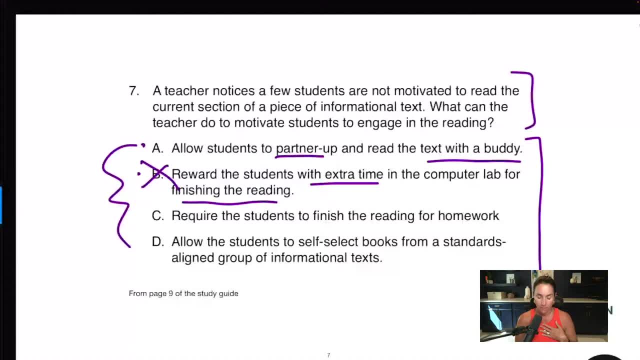 be motivated. We want students to be motivated intrinsically. right C require Already a bad word because it sounds punitive The students to finish reading for homework. Homework is a bad word. on this test, Do we use homework? Yes, of course we use homework, But on this test, homework. 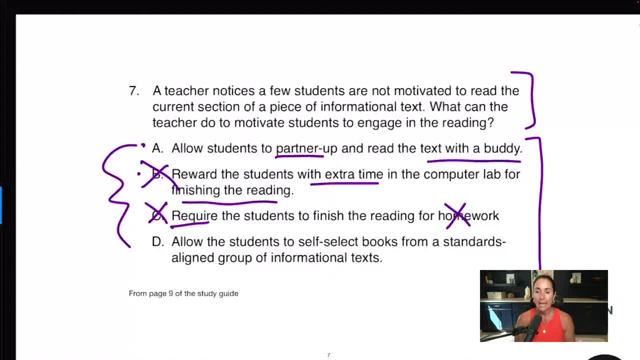 is usually attached to students who are struggling and not the best practice for those students. okay, Homework is not bad. I'm not saying homework is bad. I'm saying homework is a bad answer on this exam. okay D, allow the students to self-select books like it. those are good words. 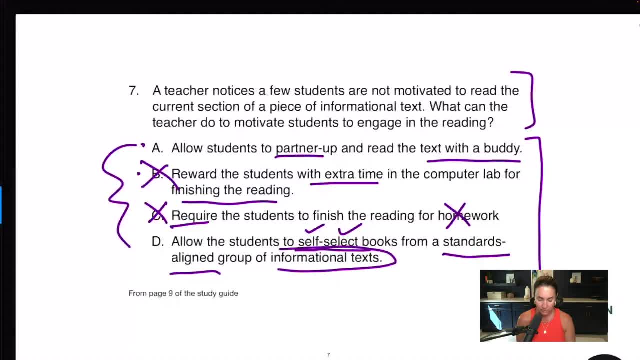 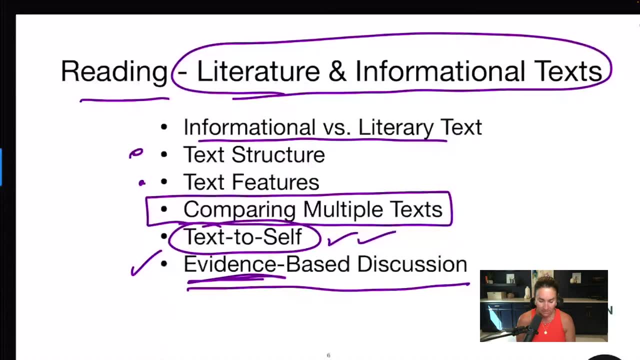 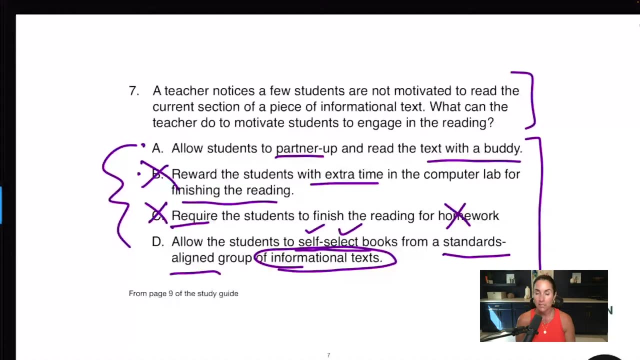 from a standards-aligned group of informational texts. Notice how many good words are there: Self-select books. Self-selecting books helps with this text to self Allow students to pick what they want to read. We want them to like to read, So self-selecting books is good. Standards aligned, Anytime you see. 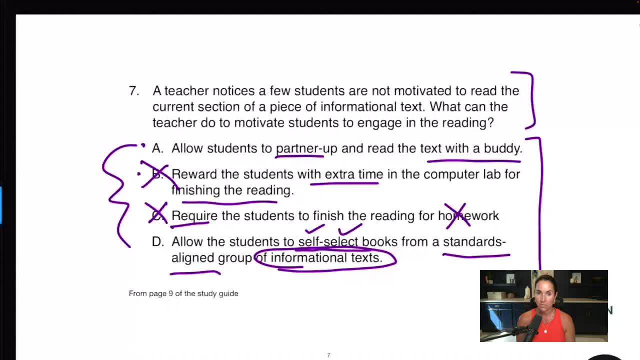 standards, alignment, academic standards, anything about standards in an answer choice. slow down, It's probably the right answer. And then we're talking about informational texts here D's got all the good words. Let's read the question. A teacher notices a few students are not motivated. 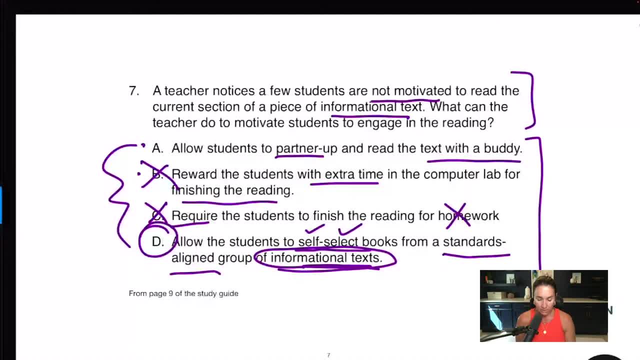 to read the current selection of a piece of informational text. What can the teacher do to motivate students? Now, if I'm a new teacher, rewarding them with extra time sounds good. right, Yeah, give them extra time, Give them a lollipop, Give them a homework pass or something like that, But in 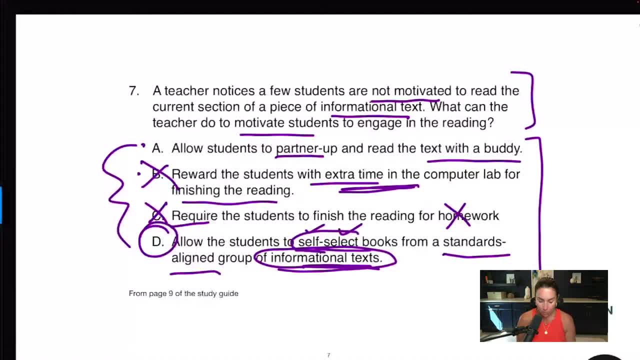 terms of best practices. allowing students to pick what they want to read is an intrinsic motivator. Notice: D is intrinsic and B is extrinsic. all right, Partnering up is okay, but that's not necessarily going to motivate them to read informational text. It might momentarily. 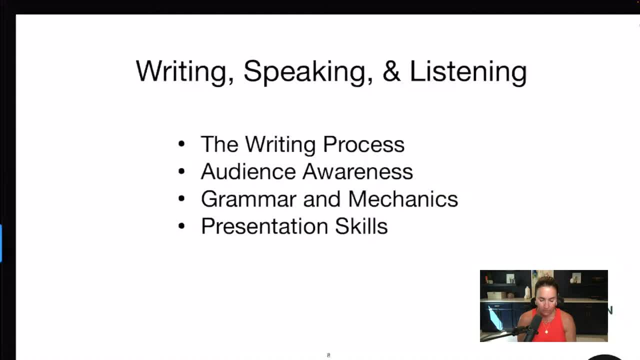 but D's got all the good words in it. All right, let's have a look at writing, speaking and listening. This is the last part of the 5002.. Then we'll move on to the math: Writing, speaking and listening. So we're. 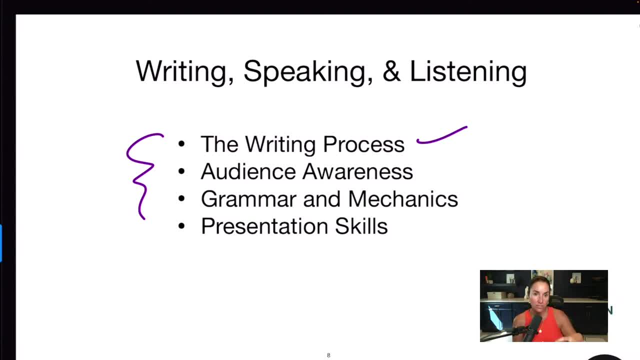 going to talk about the writing process all the way from the developmental stages of writing, which is like scribbling, mock handwriting, phonetic spelling, things like that. Then, as we get into the upper grades we're talking about, you know, the drafting process. 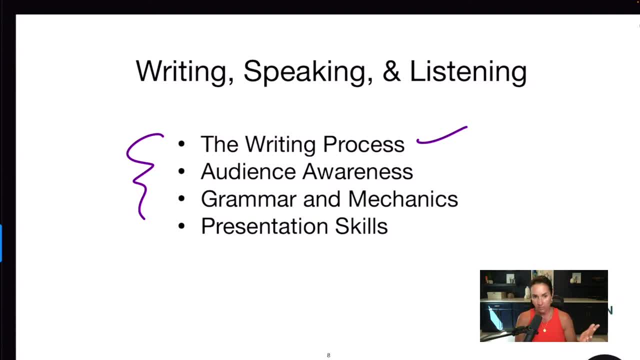 the peer review process, the revision process, the publishing process and all of that Audience awareness, Understanding audience and purpose for what we're writing for. You will have a couple questions on grammar and mechanics. not a lot, probably three or four Stuff on parallel structures. 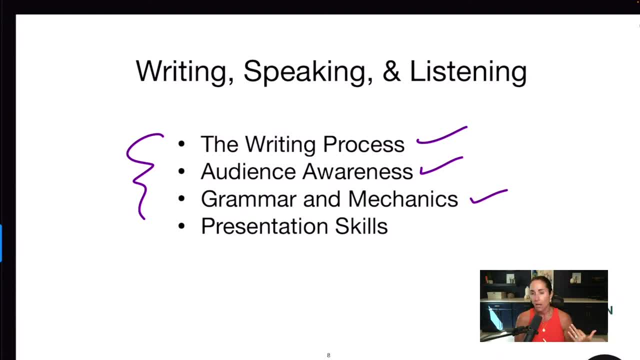 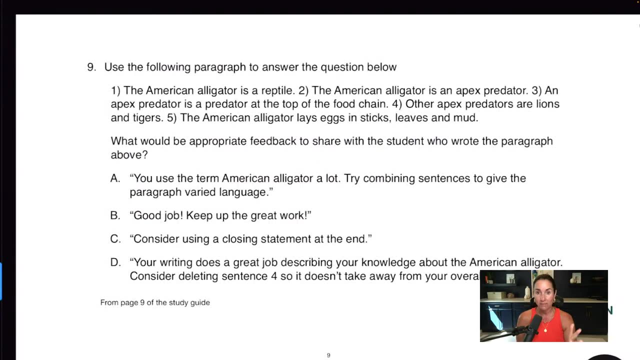 misplaced modifiers, verb phrases, pronoun antecedent agreement, things like that. And then teaching students how to present their ideas clearly and coherently in front of the class. all right, So let's have a look at what that might look like. Now. you'll see stuff like this where 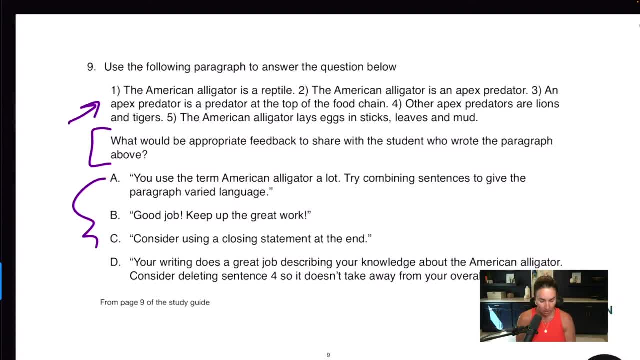 you have student writing here. you've got the question stem and you've got all of this here And I can see there's quotes here. You'll see this on the exam. Just read these and see what you think. okay, So it says you use the term American alligator a lot. Try combining sentences to give. 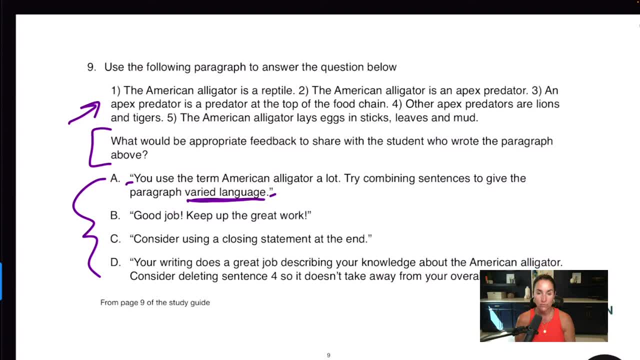 the paragraph varied language And I like the term varied language. Varied language for the writing section of the exam is good. I want to teach students how to vary their sentences so they're not so robotic, you know. So A is okay. I don't see anything positive in A which we want to. 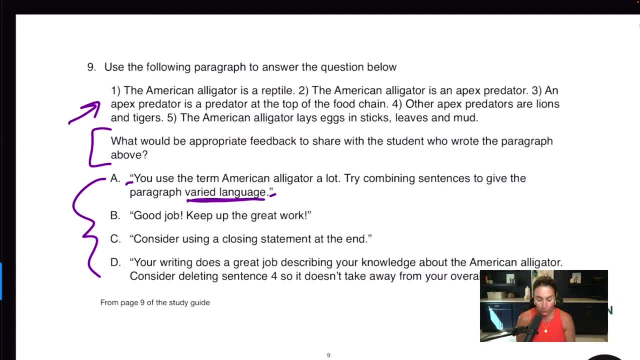 do positive feedback but I'm going to leave it. B good job. Keep up the great work. B stands out as a bad answer. Even though it's positive, it's not specific and meaningful. Feedback should be specific and meaningful And you could see here in the question stem. it says appropriate feedback. 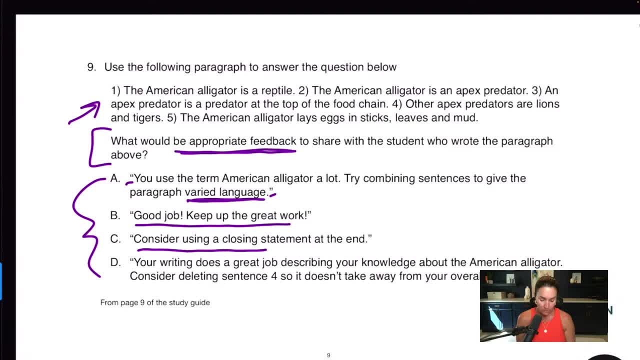 C. consider using a closing statement at the end. Okay, this is specific, but it's not real meaningful. I don't love C. B and C are out. A is okay. Let's look at D. Your writing doesn't describe your knowledge about the American alligator. All right, a positive, specific. 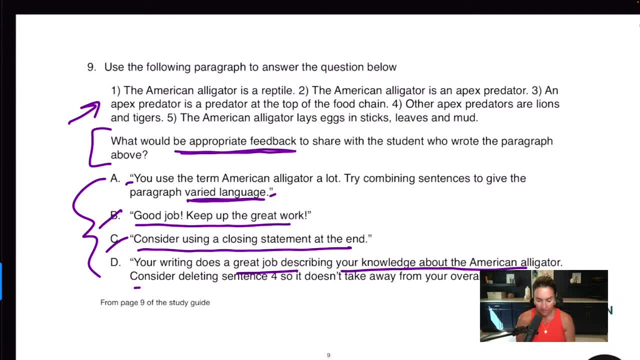 anecdote about the writing and then something they can work on. Consider deleting sentence four, so it doesn't take away from your overall theme. Not only is this positive, with a little bit of criticism, it is specific and meaningful. So I'm telling a student exactly what the student needs. 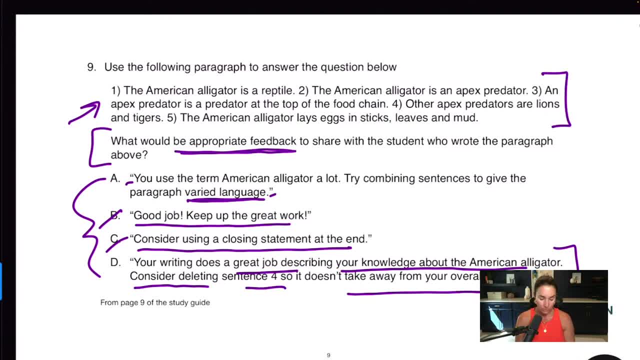 to do. I don't even need to read this, You guys. what you'll do is a lot of people who are new to testing they'll start here and they'll read all this, Then they'll read this, Then they'll read. 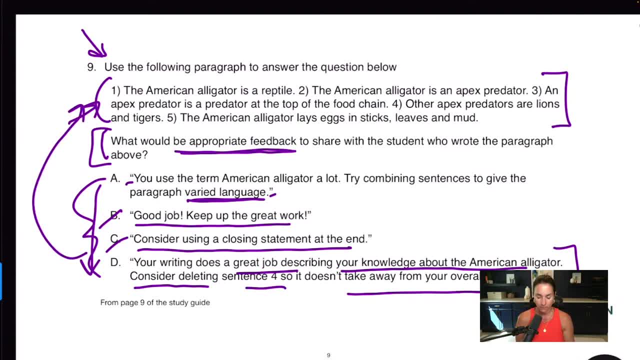 this. Then they got to go back and read this. You don't even need to read a lot of the stimulus. Now you can. of course you're taking a test. You don't want to skip things, but I'm just saying a. 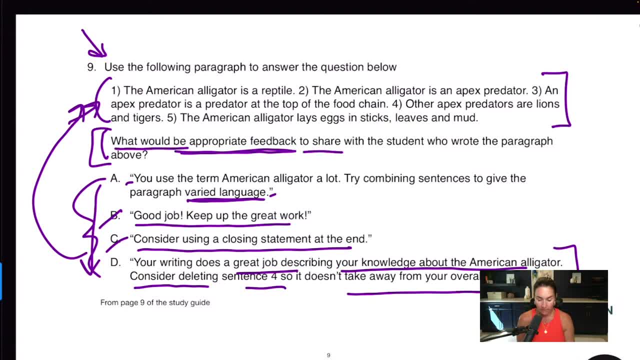 lot of times you don't have to. This stem here says it all. What would be appropriate feedback to share with the student. I don't even have to read this part up here. I know that D is the best answer because it's specific and meaningful and it's got a little positive and a little criticism. 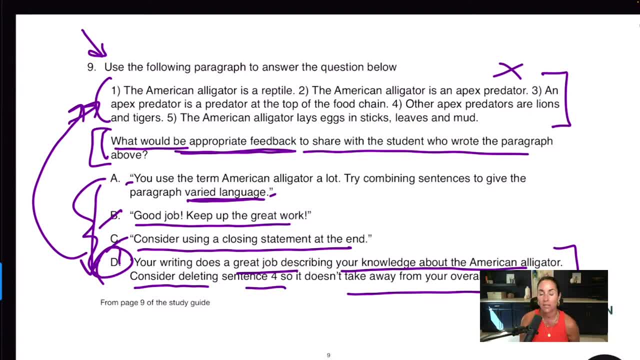 When I was a coach. I was a cross-country coach when I was a teacher at high school and my mentor used to say: you got to praise more than you kick. That means that you got to tell them they're doing a good job. 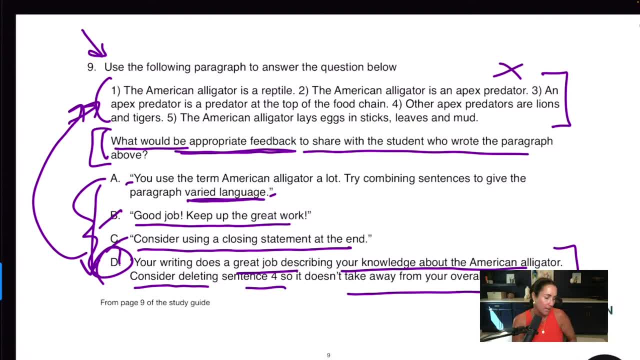 before you knock them down. You still got to knock them down, especially in sports. I'm very tolerant when it comes to reading. I think everybody learns at their own pace. I think that there shouldn't be any races to the top when it comes to reading, because everybody is learning. 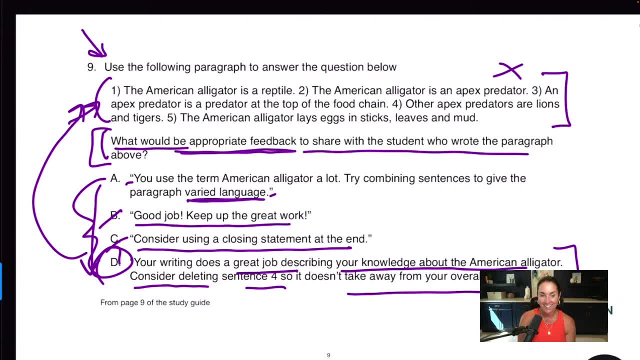 this skill As a running coach, I want to win. He had to remind me: hey, listen, Jasper, you got to go easy on that. You got to praise more than you kick. That goes the same way, especially with their writing. 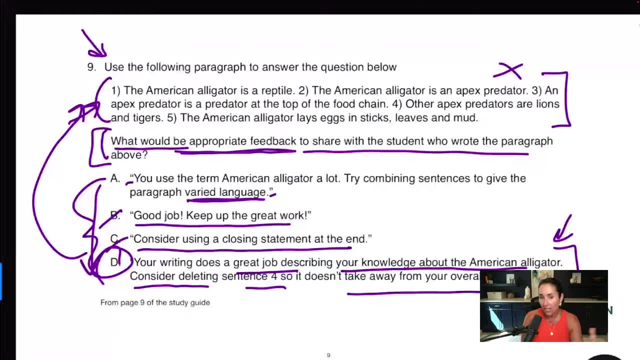 They're showing you something and they've put themselves out there. You got to tell them: hey, I really like this, and be specific, not just good job. Hey, I love the way you described your American alligator. I really liked your use of punctuation. Be specific and then hit them with. 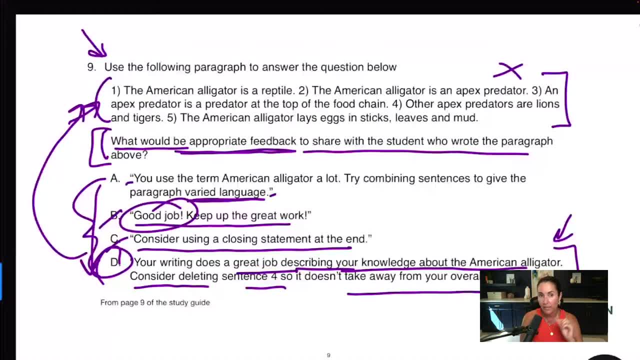 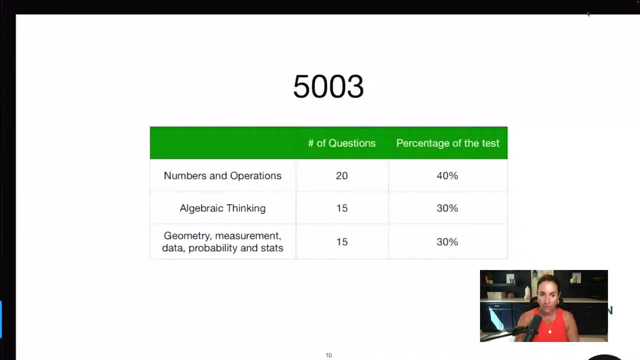 the, and I think you should also consider doing X, Y or Z. That'll be a good way to show them feedback. All right, All right, Moving on, let's go to the 5003 here Now. there are three content areas within this. 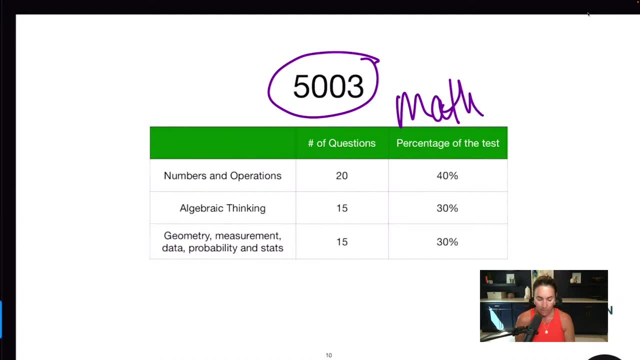 subtest. This is the math right. We have numbers and operations, algebraic thinking, geometry, measurement, data, probability and stats. Now, the biggest part is here- numbers and operations, because it encompasses so many things. It's going to encompass place value. It's going to encompass 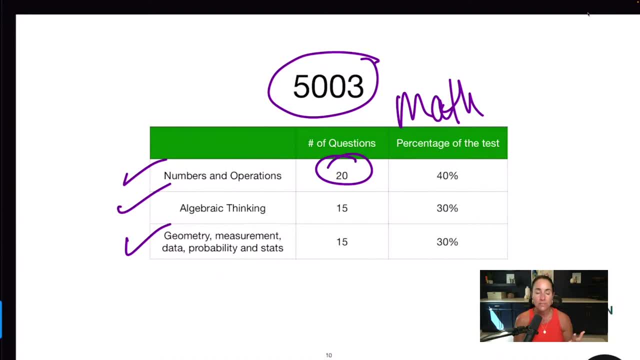 those very beginning skills like subitizing and things like that. And it's also going to encompass proportions and percents and that type of stuff. So it's a big one. Then we have algebra, and then we have geometry, probability and stats. Let's have a look at 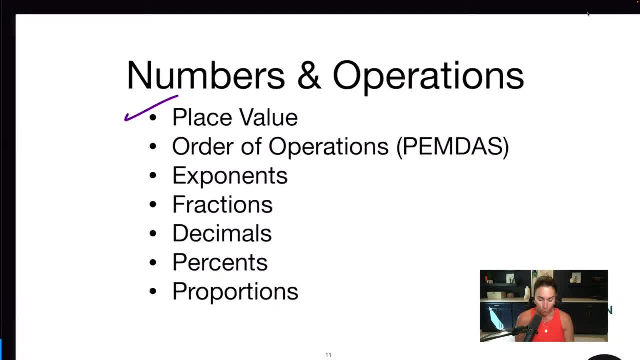 numbers and operations. So again you're looking at place value order of operations, also called PEMDAS. In this category you're going to have exponents, fractions, decimals, presents and proportions, Anything, numbers, anything, operations And most math tests. 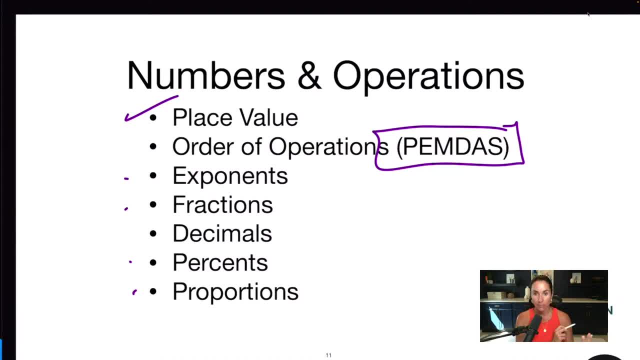 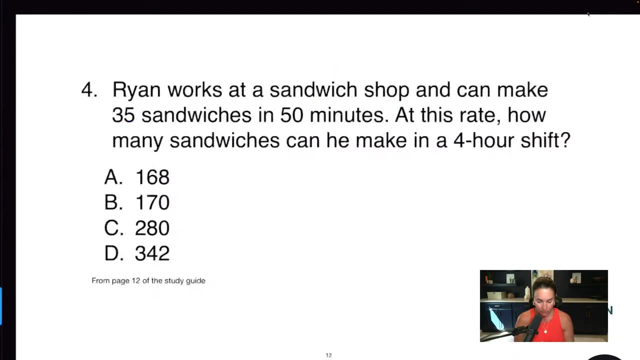 have numbers and operations, algebra, geometry and probability and stats. Even ACT is the same. 10th grade math exams are the same. Elementary math exams are the same. They're just, you know, developmentally appropriate. based on this, okay, So let's go ahead and have a look. 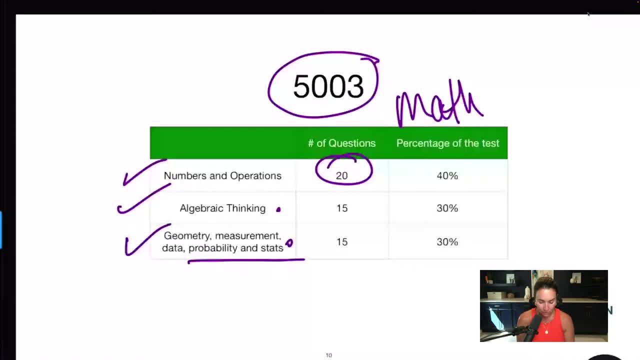 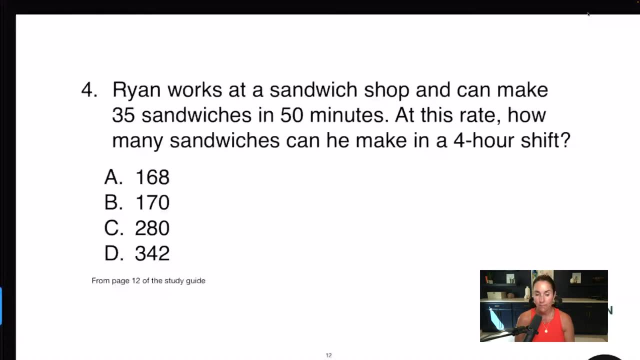 at a question here. Now, this one is coming from numbers and operations, this first content category. all right, So you can see that we have a word problem And now remember. this is why you can't try to memorize. 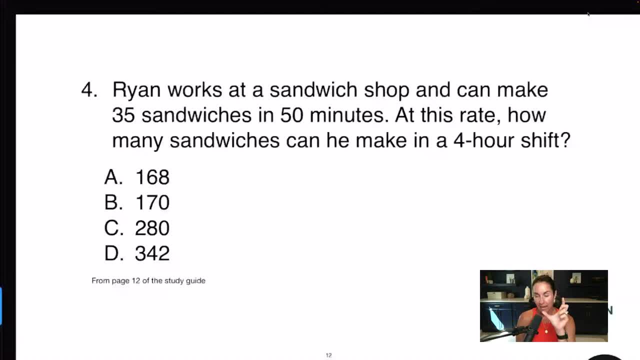 Questions, because I could ask you this question as an actual math question. I could ask it as a word problem, I could ask it as a diagram. It's why you have to have the skills before you know anything else. So don't just try to memorize. It won't work. All right, I can see again. I'm. 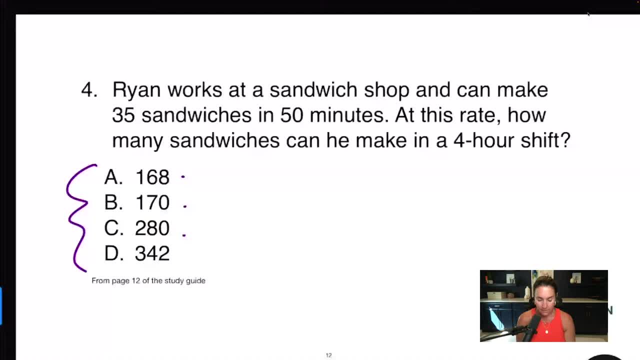 working backwards, I have to pick an actual number, so I'm going to have to work this out. Let's have a look at the question. Ryan works at a sandwich shop and can make 35 sandwiches in 50 minutes. Let me get my calculator out. Hold on. 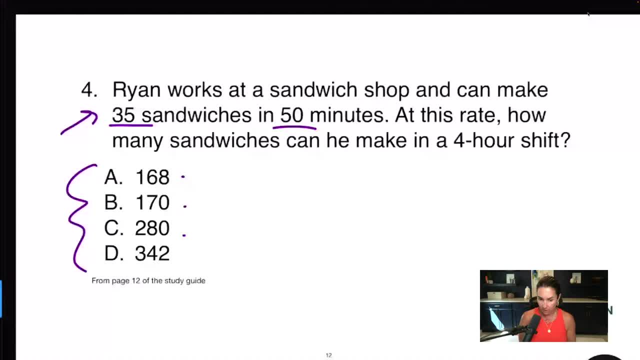 I have a calculator on this test. It's an on-screen for function calculator, all right. So Ryan works at a sandwich shop, can make 35 sandwiches in 50 minutes At this rate. it's a key word here, telling me what I need to do. How many sandwiches can he make in a four-hour shift? Rate indicates I'm 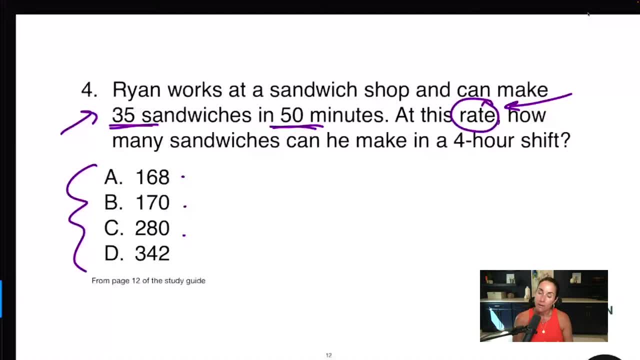 going to need to set up a proportion. Now, every time I do math live on air here, I always get criticism: Why didn't you just do it this way? Why didn't you just take the shortcut? Because people who are watching this video usually are struggling in math, and I want to. 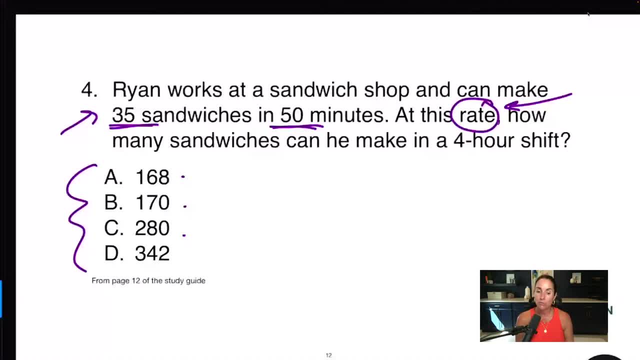 show them how to do it properly before we start taking shortcuts. I want you to get through the math quickly, but this is the best way, I think, as a teacher, to do this for my students, which is you guys. Of course, there are quicker ways to do this, but I need to set up a proportion so that 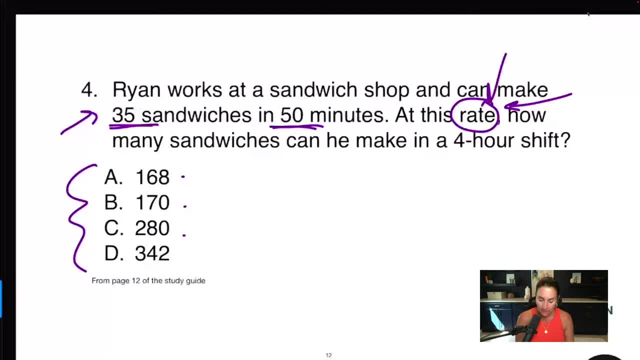 those of you who struggle with math understand what's going on. Rate is a proportion. You might see it like this: four to one. This is a ratio. A ratio or a rate? We're talking about a proportion, If we're going to use that for this. 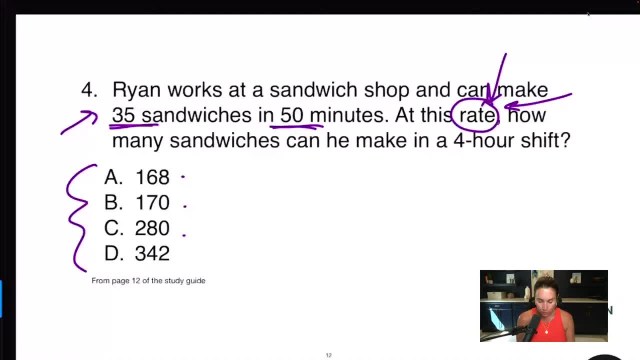 particular word problem. I'm going to set two fractions equal to one another. We're going to get matchy matchy. Whatever I put on the top is going to be the same on both sides. Whatever I put on the bottom is going to be the same on both sides. Let's start with 35 sandwiches in 50. 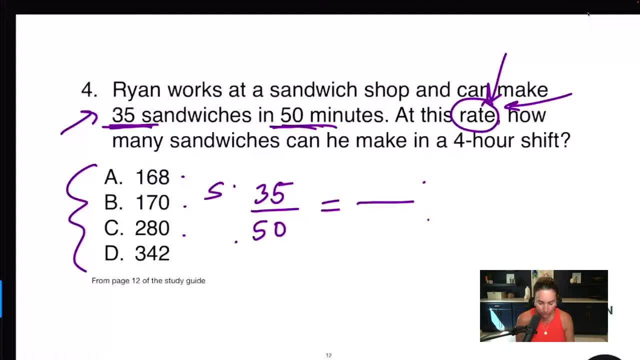 minutes. I have sandwiches over minutes. Let's do the same on the other side: Sandwiches over minutes. I don't know how many sandwiches, because it says how many sandwiches can he make. That's going to become X. I'm looking for that. Can he make it a four-hour shift? I got minutes here. I. 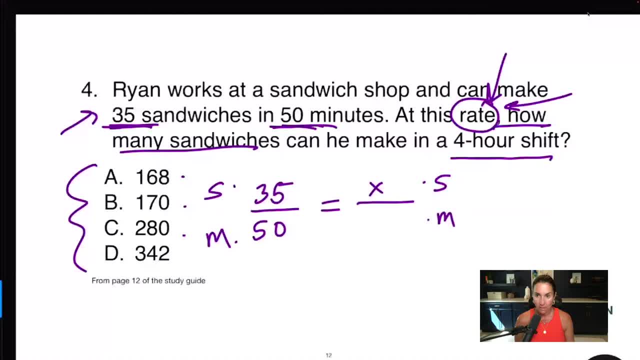 need to convert four hours into minutes. What do I do? I multiply by 60 because there are 60 minutes in an hour. I'm going to multiply by 60 because there are 60 minutes in an hour. I'm going to have four hours. This is going to be 240 minutes. Notice, I have sandwiches over minutes equal. 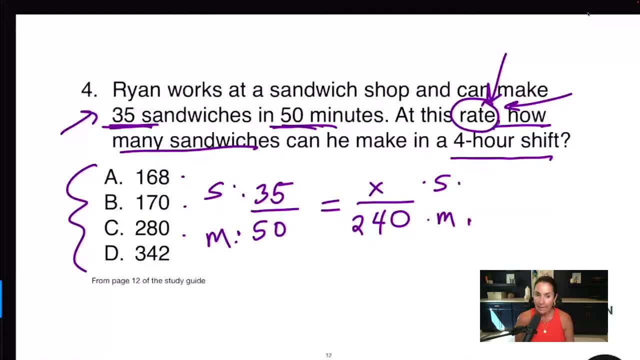 sandwiches over minutes. Matchy matchy. I can't put minutes over sandwiches equal, sandwiches over minutes. I got to have sandwiches on the top, minutes on the bottom. I could put minutes at the top and sandwiches on the bottom, on both sides, and it will work. I like to go in the order by: 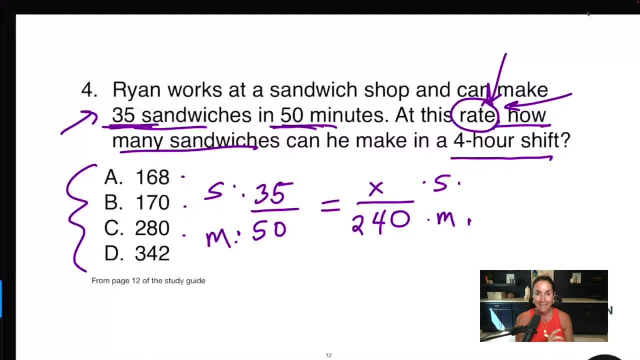 which the word problem is going. Another hint Notice: I have three out of the four values I need here. I have sandwiches and then the time it takes, and then I have the time, but I don't have the sandwiches for the other piece of it, So I need. 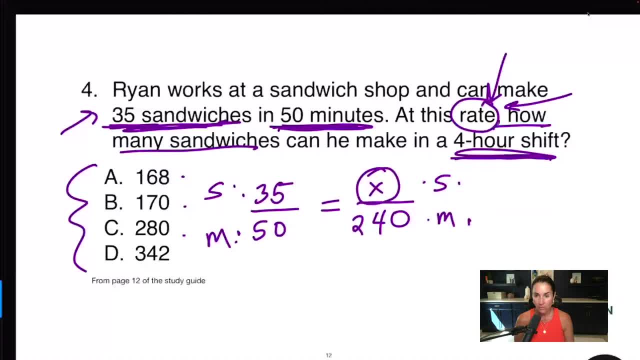 that third out of the four things. That'll also indicate you need a proportion. Now what do I do? Will I cross, multiply and solve? So 50 times X is 50X. Keep that equal sign there And I've got 35. 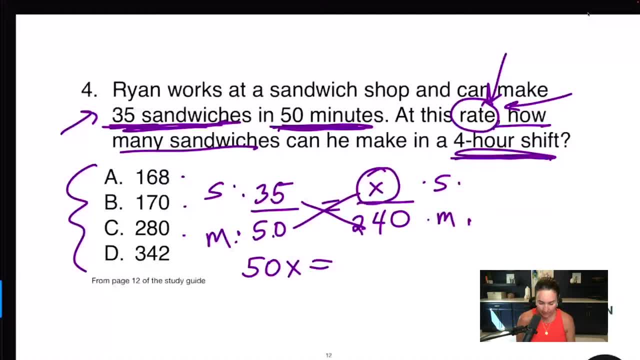 times 240. And this is going to be 8400.. Now, right away, I just want you to have a look at something. I have 50 here and I have 8400. Both ending in zeros. I know 50 does go into 8400. I can see I'm 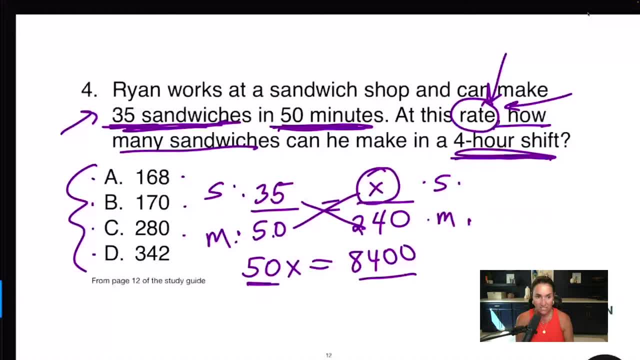 always. looking at my answer choices here, I see these are even numbers. There's no decimals going on. If I start to get weird numbers with decimals, I know I'm going in the wrong direction. But in this case I'm actually going in the right direction because I know 50 goes into 840, because, in order, 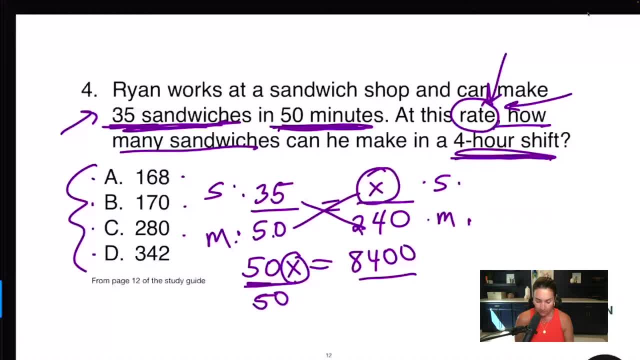 to isolate this X. I have to do it in the right direction. So I'm going to do it in the right direction. I'm going to divide by 50. Divide by 50 and I get 168 sandwiches in a four hour shift. 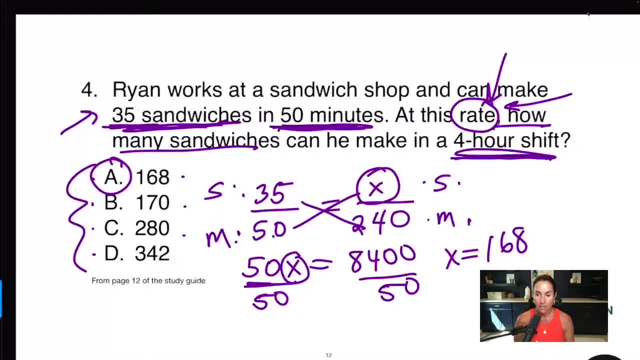 X equals 168.. All right, Now there are shortcuts you can do. There are all kinds of things you can do. I like to set it up this way: It's quick: Sandwiches over minutes equals sandwiches over minutes. I don't know how many sandwiches I can make, and I know that I'm working four hours. 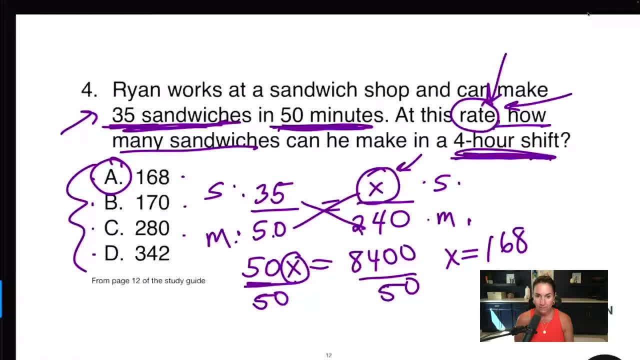 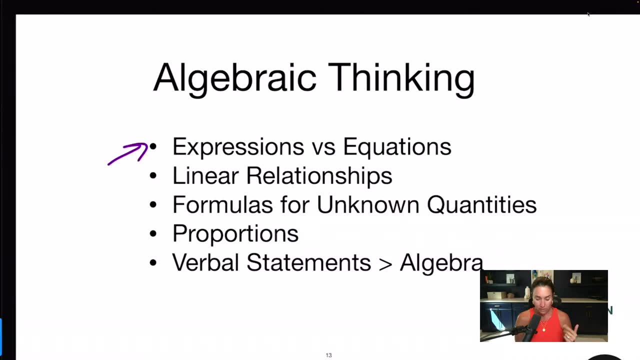 That's 240 minutes. Sandwiches over minutes equals sandwiches over minutes. I don't know how many minutes sandwiches over minutes. matchy, matchy cross. multiply, solve for X, All right, And we get 168.. Okay, Algebraic thinking. Now this is where you might have expressions and equations linear. 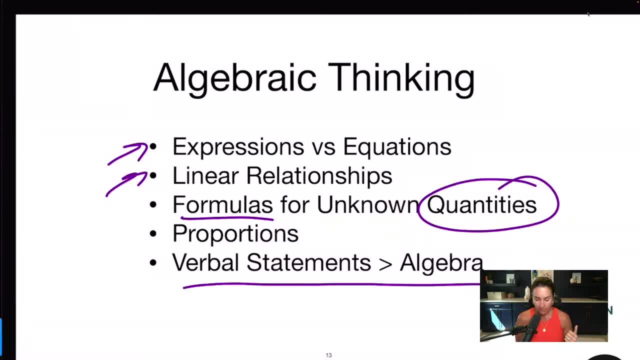 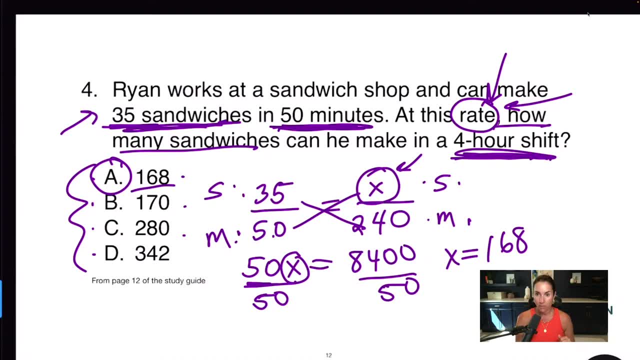 relationships, formulas of unknown quantities, verbal statements, proportions. Notice that this, this problem here, could also be considered algebra, because I had to use algebra to solve it. I had to solve for X. that's algebra. So there's a lot of different skills being assessed in this. 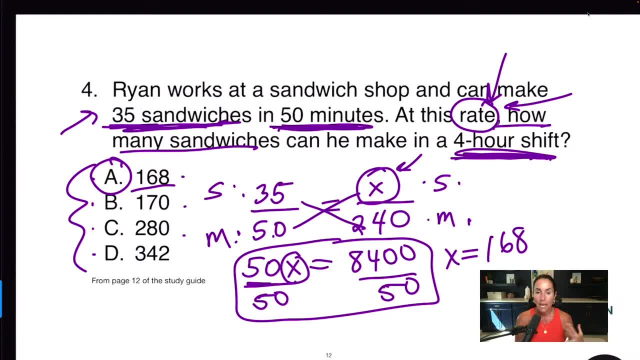 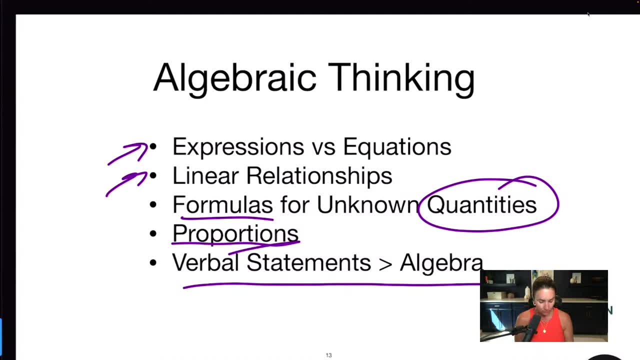 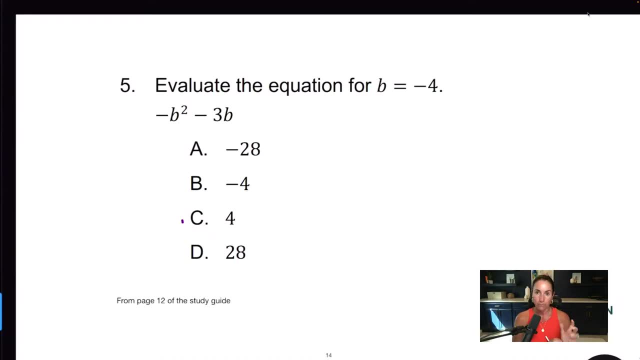 particular question. I actually really liked this question cause it's numbers and operations and it's also algebraic thinking. So just know that And we'll get into a few few here Now. a classic algebra problem is something like this, where you actually see the, the expression Okay. 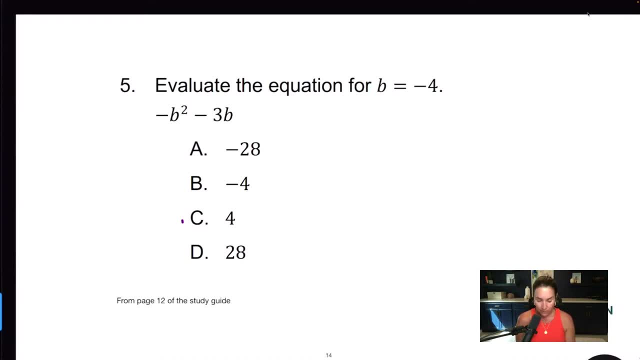 So you can see here that I'm, I'm being asked to evaluate the equation. This should actually say expression, Cause there's no equal sign. So this should say expression. Sorry, Just getting technical here. That should say: evaluate the expression, for B equals negative. 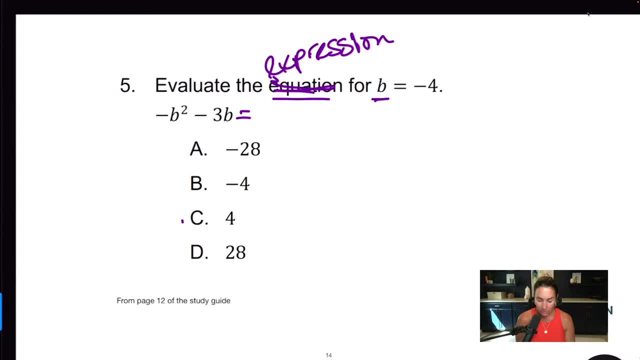 four. So basically what they're saying here is: wherever you see a, B, we're going to put in a negative four, So you can see what's going on here. So when I rewrite this- and again there's lots of ways we can shortcut it- I'm not going to shortcut it because I want to make sure my math is correct. 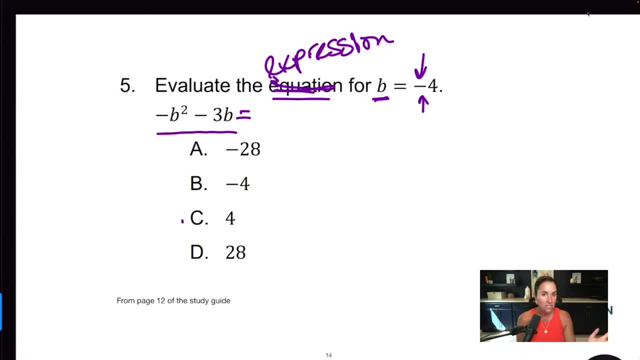 They'll do this a lot. You have to go back to the first one and you see all of the negatives and negatives and minus signs and all this stuff. They're trying to trip you up And you'll notice here that negative 28,. negative four, four and 28.. 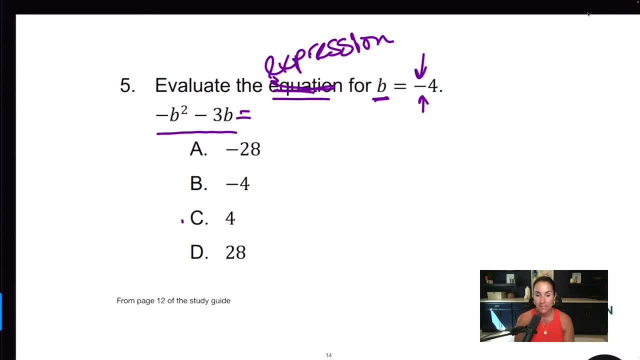 These are answer choices. If you misplace the negative, they have your incorrect answer in the answer choices. They will anticipate your errors, common errors, That's. that's what good math test makers do. So you have to be careful. So I'm going to just bring this negative four into this equation. 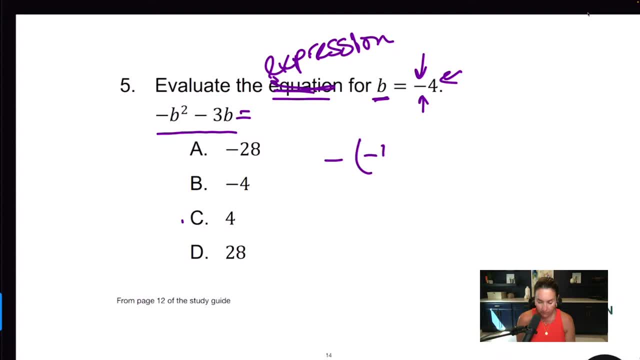 So I'm going to keep this negative And, wherever I see it now, I'm going to put a negative four into the equation, see a, B. I'm going to put a negative four minus three times negative four. Keep it proper, Don't. 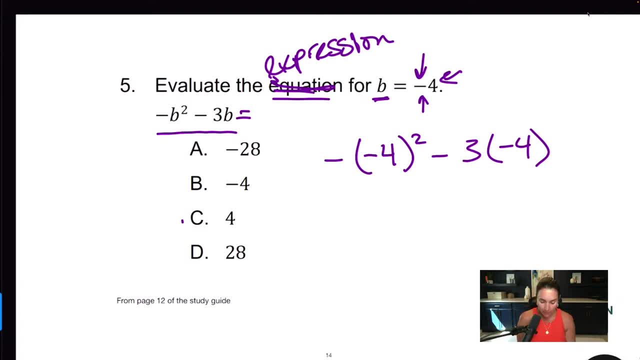 skip any steps because there's too many negatives. I don't like it. Now I'm going to use PEMDAS, Always use PEMDAS. Now I don't have any parentheses. Parentheses means there's like some sort of equation inside of a parent or some sort of operation inside the parentheses, like 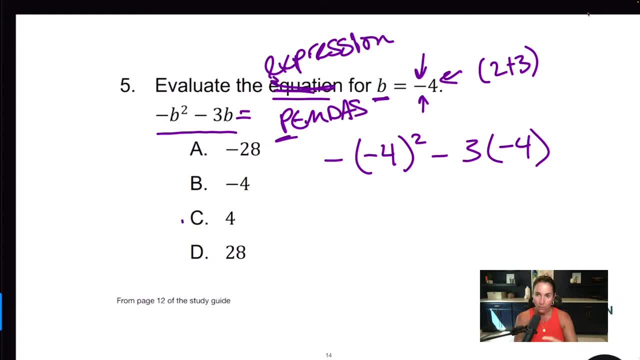 here two plus three. We don't have that. We do have parentheses, but there's nothing, no operation, going on inside of them. So I can move to exponents here Now. be careful: If I had done this first, this would be considered multiplication A negative, times a negative. 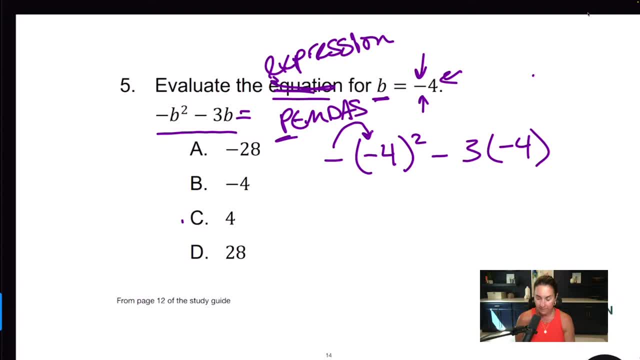 that would be a positive four, And then four to the second power would be 16.. But that's not the proper order of operations. You've got to be careful here. Start with the exponent first. negative. four times Negative four is positive 16, but I have this negative here. Notice that becomes negative 16.. 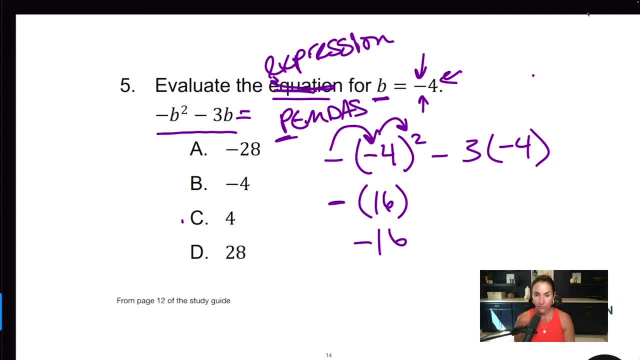 Had I distributed this first, I would have gotten an. uh, I would have gotten just 16.. It would have changed my whole thing. Now I'm going to bring this down: Negative, three times a negative, four is a positive, 12.. Notice, I have negative 16 plus 12.. And my answer is going to be: 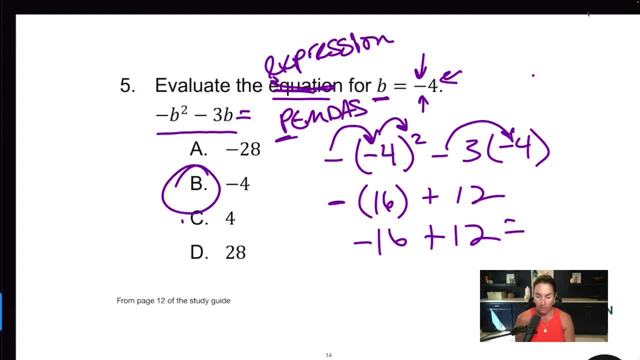 negative four, because negative 16 plus 12 is a negative four. All right, Now you can even draw a number line if you wanted to. If I had a zero here and I was all the way down here by negative 16 and I went up one, two, three, four, that would be a negative 12.. I'm still in the negative 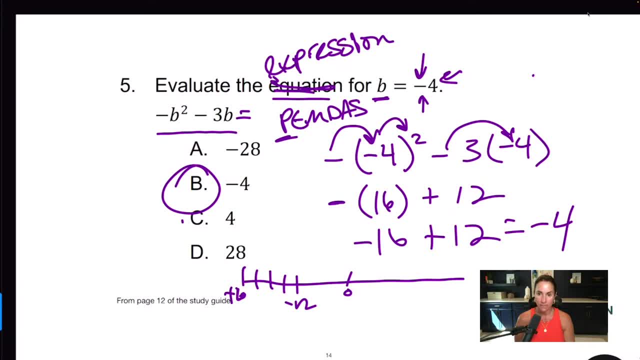 Just depends on how you want to do it. Got to be careful with those negatives, Okay. So again did the exponent negative four times negative. four is 16.. Still have that negative there. When I distribute it in, I get negative 16, and then I have a negative three times a negative. 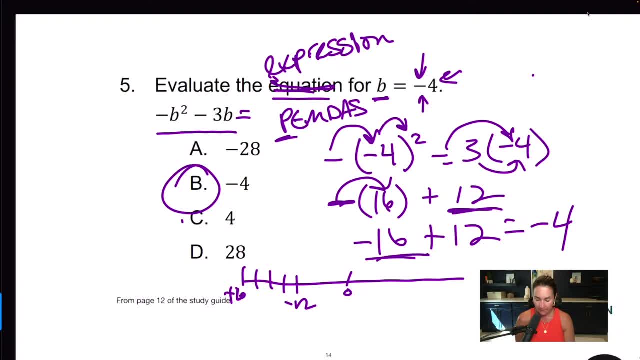 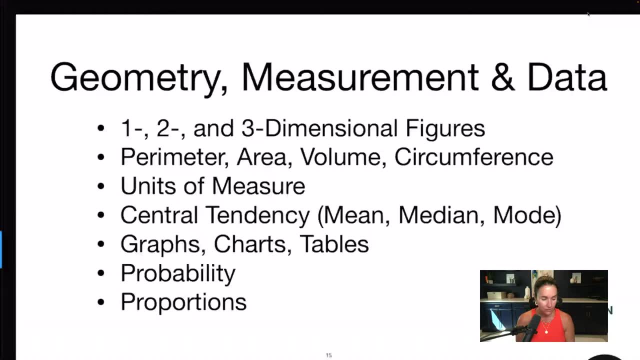 four Negative times. negative makes it a positive 12.. Negative 16 plus 12 is negative four. All right, And the last section of the math, geometry, measurement and data, probability and stats. I had to shorten that a little bit here, So we're going to have one. 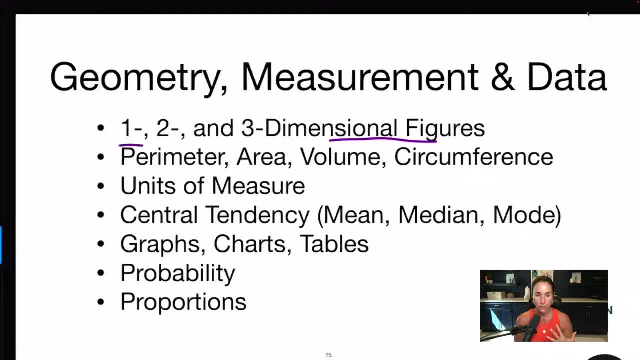 two, three dimensional figures. We might get this in a word. problem. We might get an equation, a perimeter area, volume, circumference, circles, cylinders, things like that, Units of measure, cups to gallons, pints to quarts, things like that. You might see some. 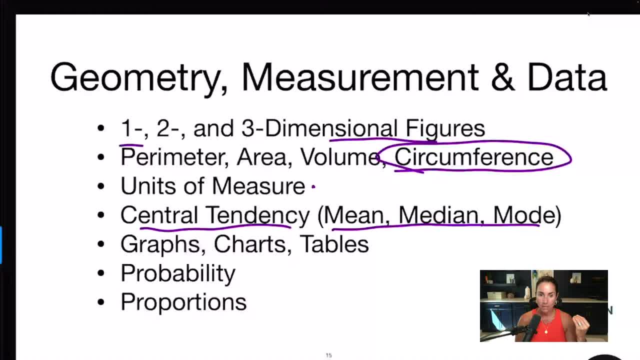 central tendency mean median and mode averages, things like that. You're definitely going to have some charts and graphs, tables, probability and, again, proportions. Proportions go across all of them in math, right? So let's have a look at this here. What is the perimeter of a square? 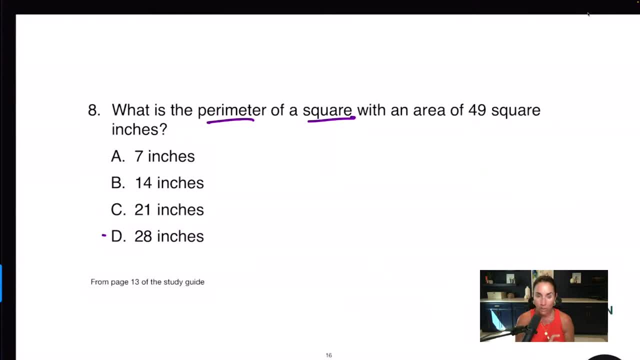 Two keywords here: perimeter of a square. Remember, perimeter is when we add up all the sides. Area which we have here is multiplying base times height. So a couple of different things here. Perimeter is this side plus this side plus this side plus this side, And area is base. 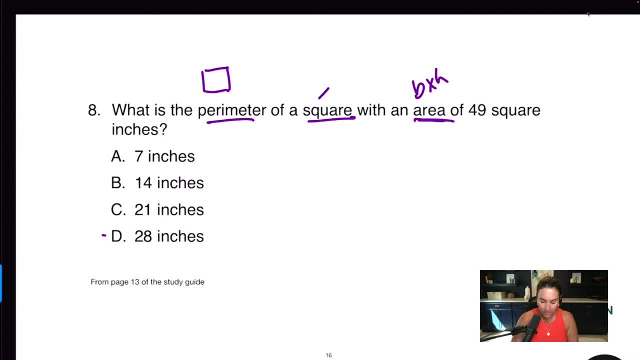 times height. All right, And we know it's a square, All sides are equal, And 49 square inches is the area, not the perimeter. the area, Okay. Well, if I have a square and the base times height equals 49, and these two are equal, this is going to be 7 times 7,. 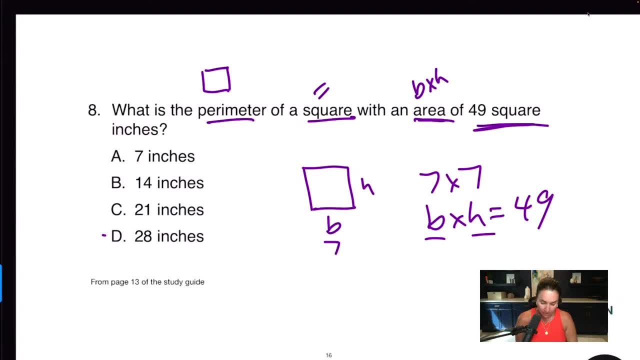 right, Because 7 times 7 equals 49.. So that means the base is 7,, the height is 7,, the top is 7, and the sides are 7.. They're all 7 because we have a square, And 7 plus 7 plus 7 plus 7,. 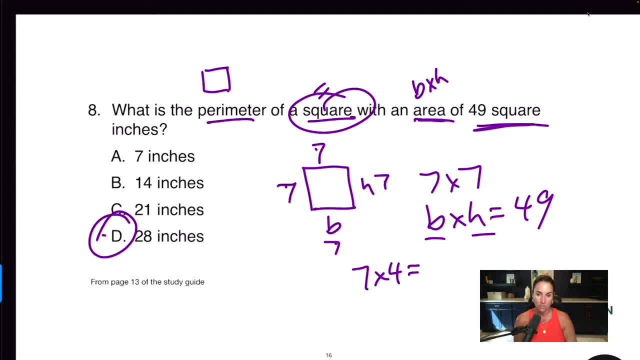 or 7 times 4 equals 28 inches. So you've got a lot of different things going on here. You have to make sure you understand your rules for squares and rectangles and rhombuses and things like that, And we do cover all of that in our book. We have a lot of information. 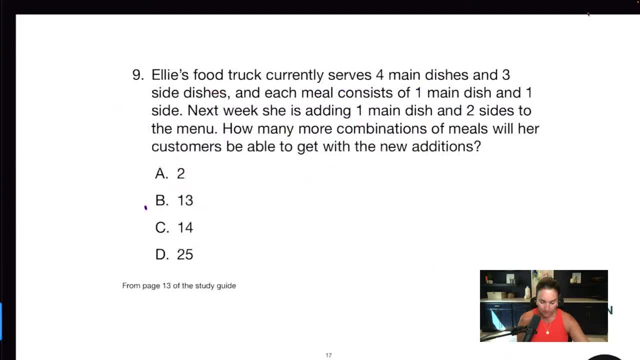 for that in our book. All right, Let's try another one. This one is more about probability and combination. So if I have a look at these answer choices here, I can see that I'm just looking for straight up numbers. Let's have a look at number nine: Ellie's food truck currently. 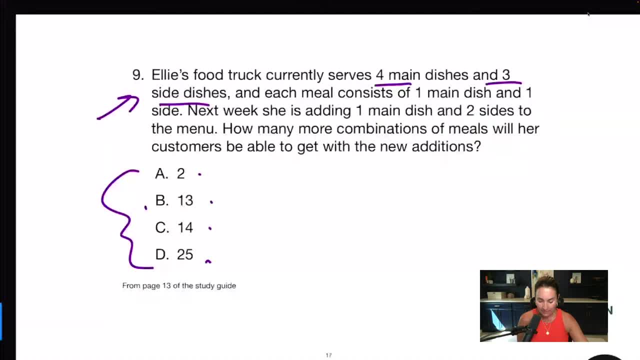 serves four main dishes and three side dishes, And each meal consists of four main dishes, one main dish and one side dish. Okay, You get one main and one side. Next week she is adding one main dish and two sides to the menu for people to pick from, So instead of four, 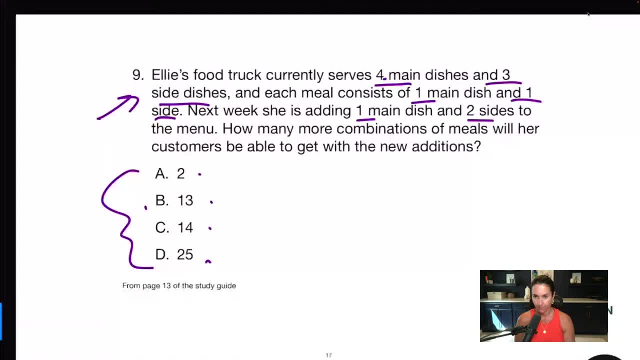 to three. it's going to be five to five. How many more combinations of meals will her customers be able to get? All right, When you see this word combination, don't start going: okay, main and a side one. main and a side two. Okay, Let me switch them around, Just use: 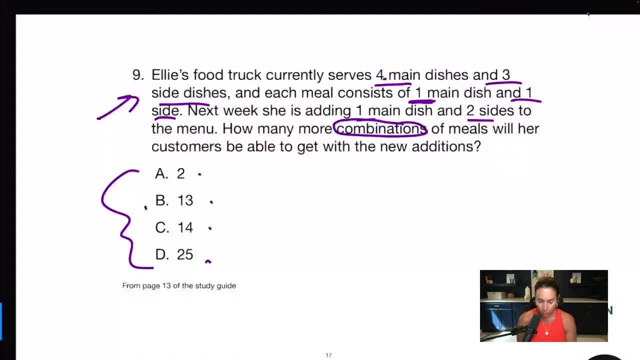 multiplication, Because there's only because you only get one main and one side. just do four times three. Four times three is 12.. There are 12 different combinations currently that I can use right now when I pick my mains and my sides. 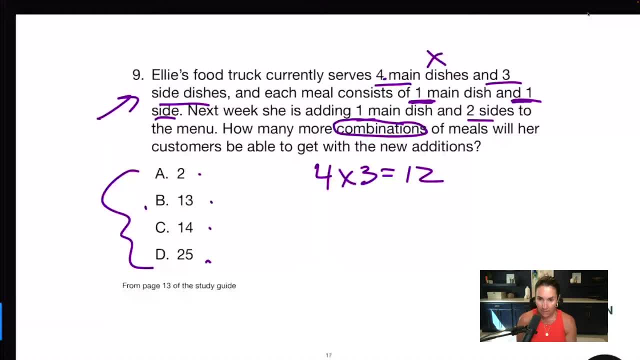 for Ellie's food truck. But she's taking these four mains and sides and turning them into. she's adding a main, which makes five mains, and two sides, which means five sides. Well, what's five times five? The new one is going to be 25.. Now, be careful, You might go okay, 25, we're done. 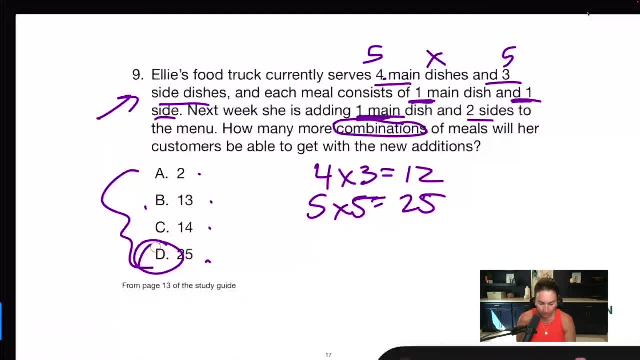 No, Read the question, stem. Be careful. They've anticipated you moving quickly. It says how many more combinations, not how many new combinations. how many more combinations of meals will her customers be able to get? Well, that's 25 minus 12.. That's 13.. There are 13. 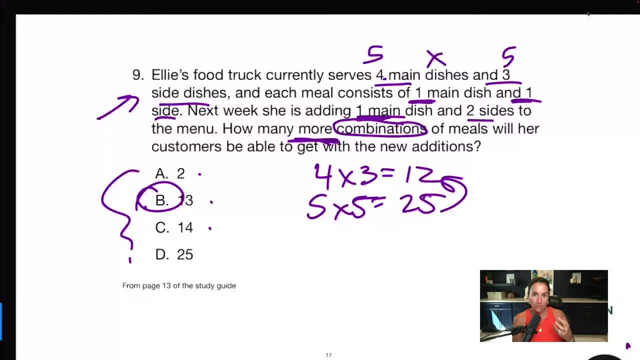 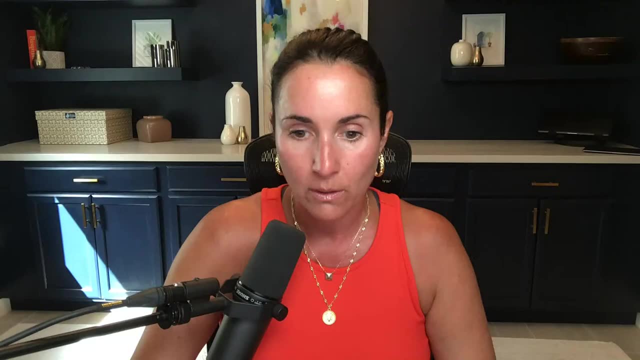 additional, more combinations that they can have now with these, this new main and these two new sides. Be careful, Read the question all the way through. Okay, All right, I'm going to just stop here, Go to my thing here and just see if 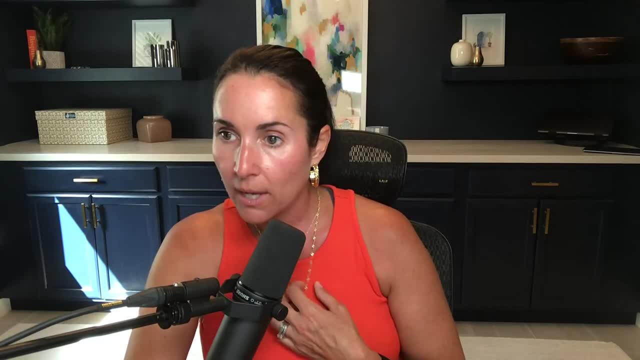 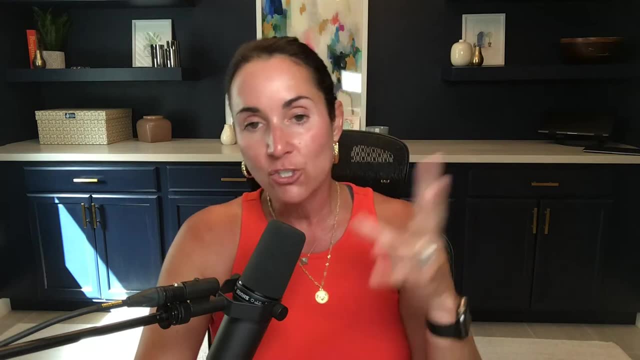 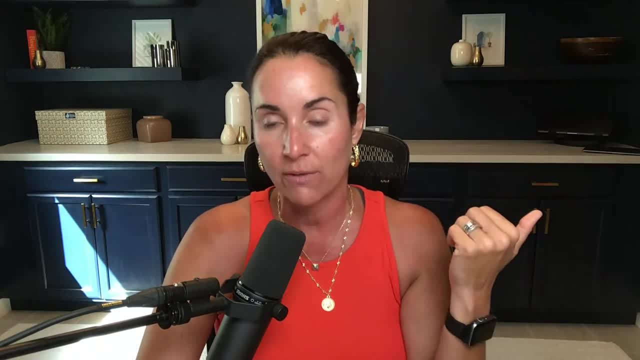 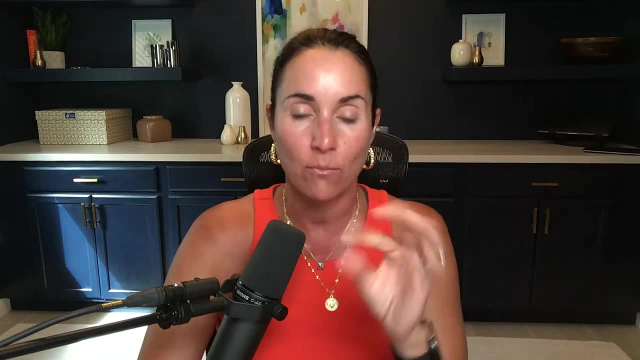 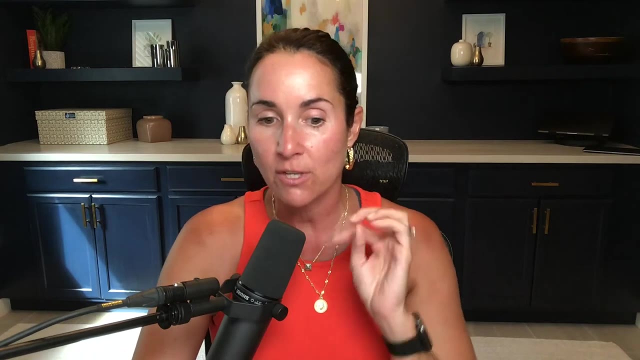 do like a week for ELA, a week for math, a week for social studies in a week for science. but you can certainly do it quicker. some people like to cram. I like small incremental practice sessions over time rather than cramming. all right, can we use a calculator button for the combination? you can, Sabrina, there is a. 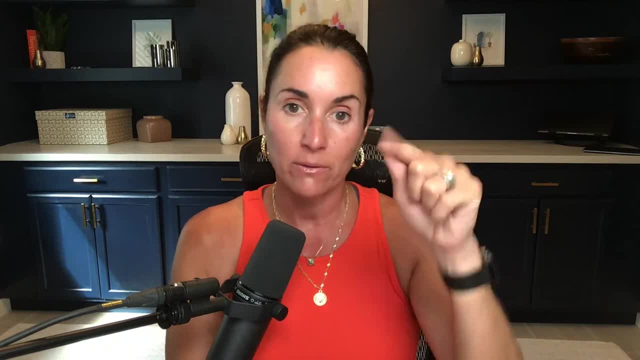 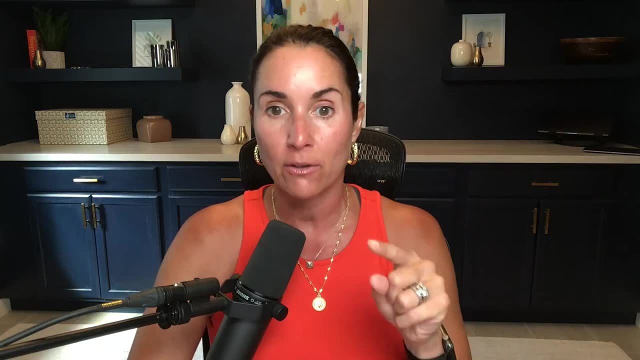 four function calculator online. so what I would do is download the online. you can if you have a Mac- there's a calculator app in there- but I would download the app for the calculator and just practice using it on your computer, because it's a lot different than typing it in here. okay, do we need to memorize? 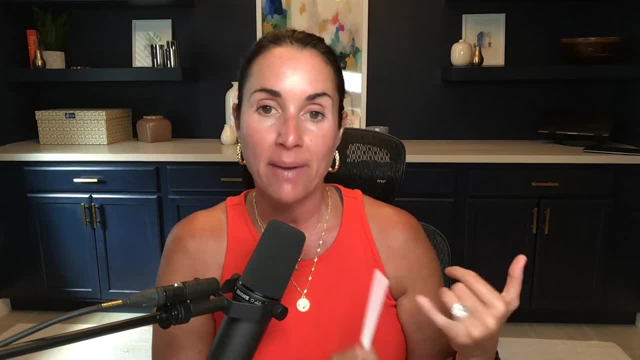 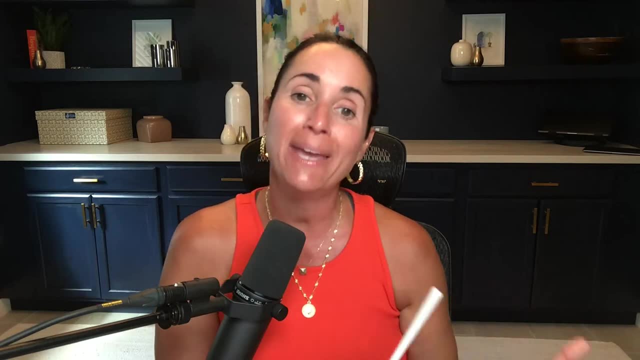 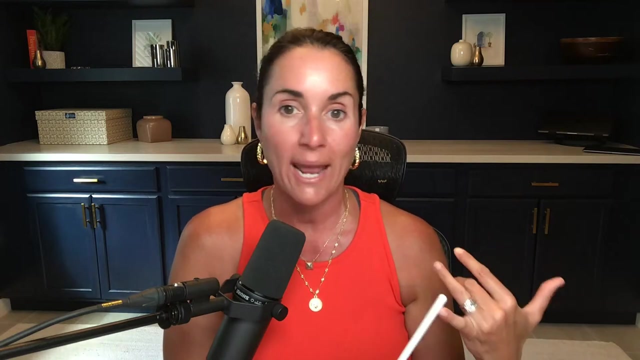 all the formulas in math? no, you do not. they have them embedded in the question and they will also have a formula sheet for all the main ones. okay, but I do recommend you know, like, what is area of a square and a rectangle, what is area of a triangle. those are things you should know. one half base times height is the. 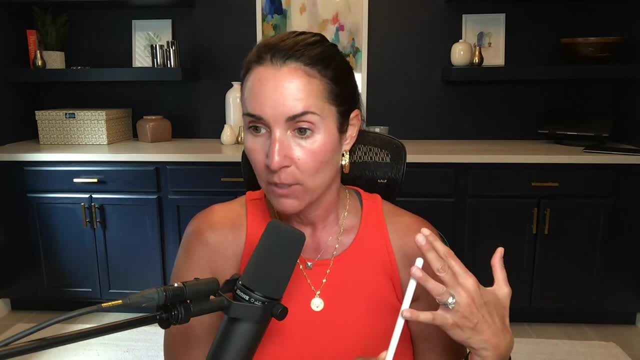 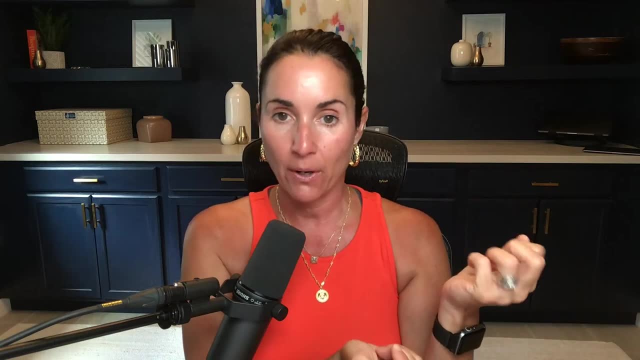 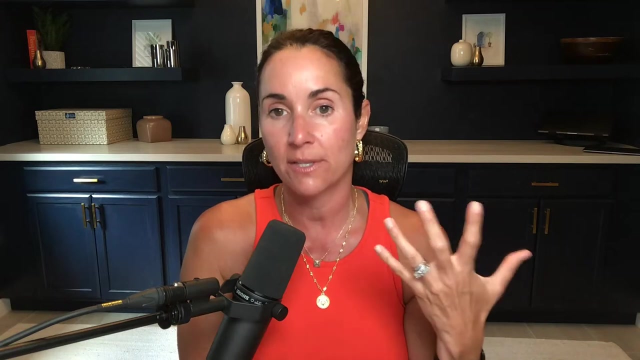 triangle base times. height is the rectangle and square. okay, do we get scrap paper? yes, you do. in my experience it's like a dry erase paper where you can use like a dry erase marker and the paper. sometimes you'll get physical paper, it just depends on the testing center. but yes, you will get. 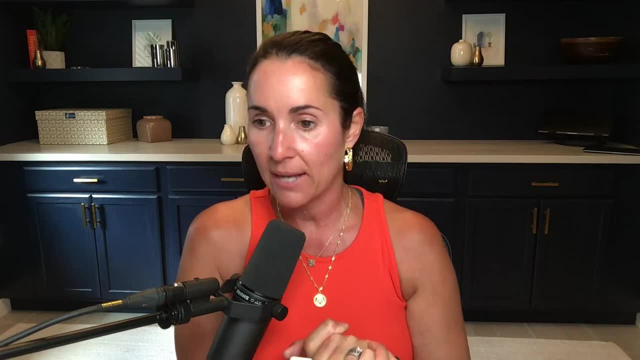 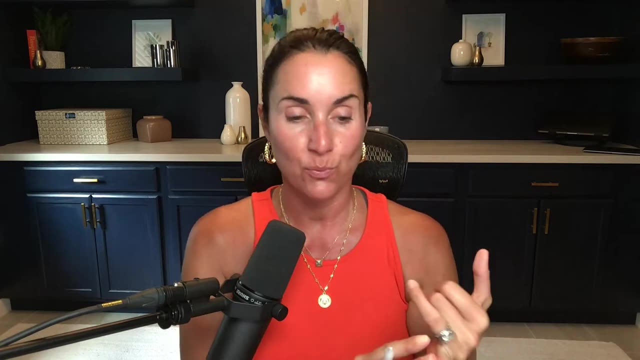 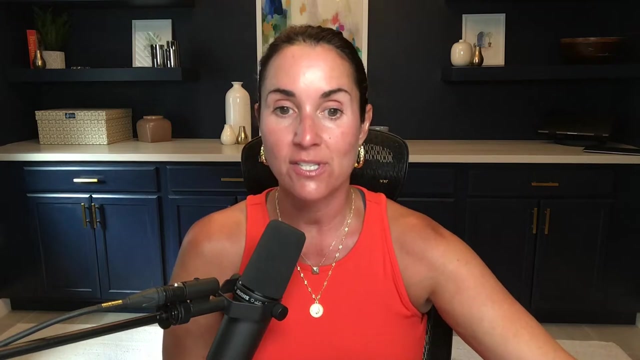 scratch paper. what is the difference in the praxis, in the praxis, to AJ? good question: praxis one is the praxis core. that is like an ACT. it has reading, writing, math and grammar. what I'm doing today is a subject area. this is about the 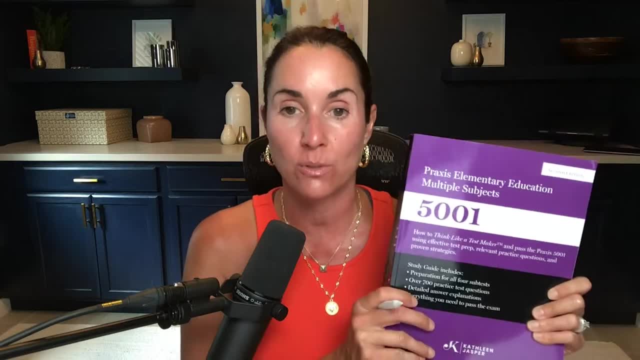 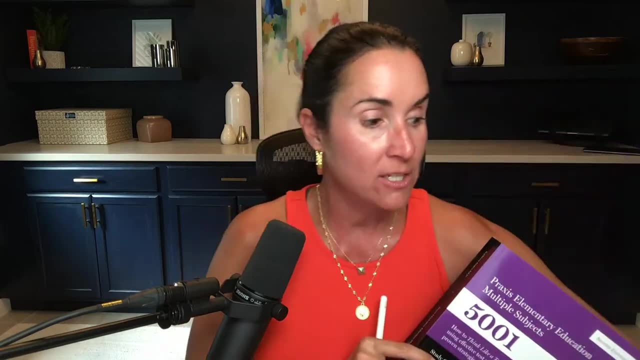 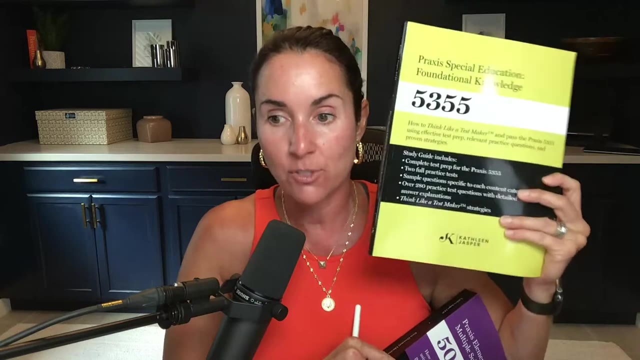 elementary school teachers want to pass this because they want to be elementary school teachers. most people have to practice, have to pass the praxis, core and their subject area exam. so like this one here is for special education. if you want to be a special education teacher, this is considered a praxis to subject. 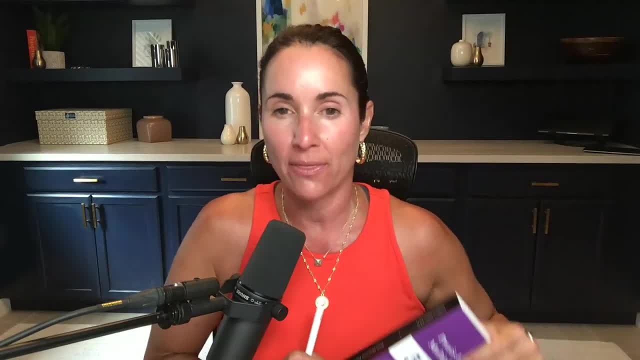 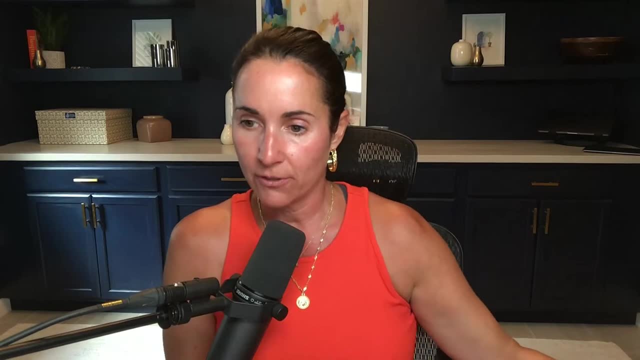 area and we have a blog on that. I'll send it out in the email. I have a blog and a video on that, so that'll that'll be good. okay, what do you recommend for science for elementary? I recommend our book. for sure, Mike T, read the questions and don't rush the. 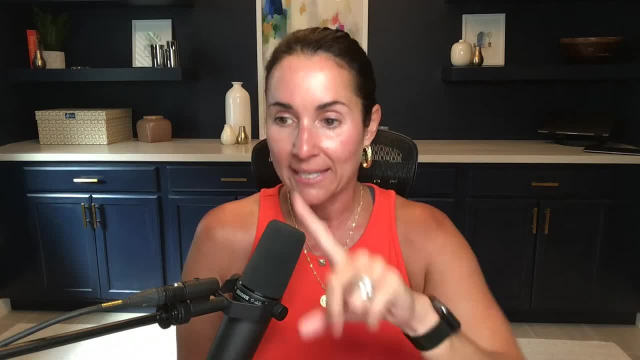 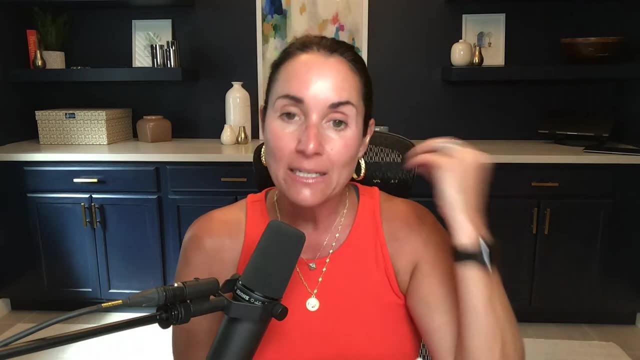 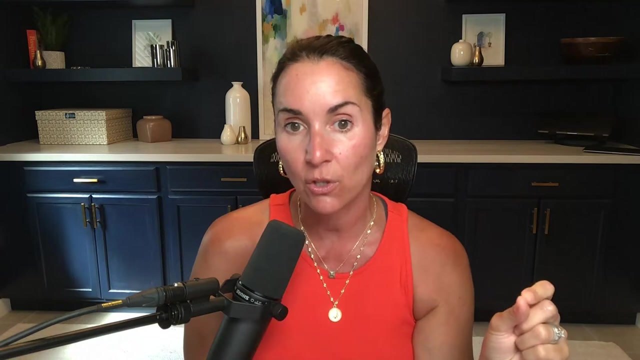 answers. you showed me that by rushing. I picked the answer quickly. yes, Mike T, it's right there, especially in math. they do this all the time. I study a CT SAT two. they anticipate your wrong answers. they put in there. sometimes they'll say how many more combinations than the original just. 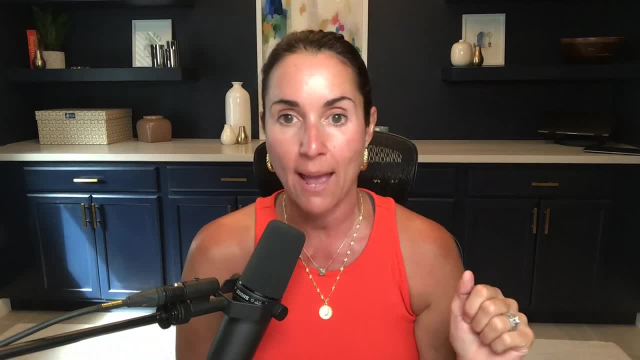 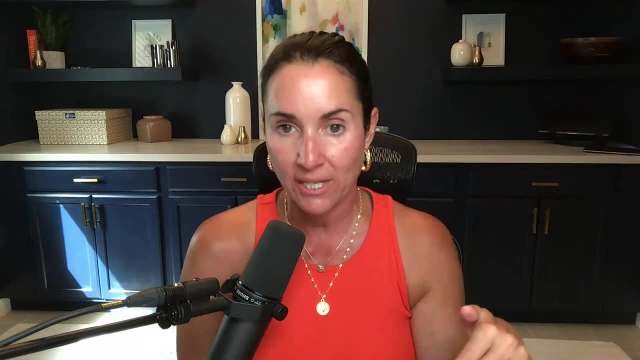 because they know you're gonna get that 25 and you're gonna go, oh, boom, 25 and grab it and move on slow down. just read that stem one more time and figure out what they're asking. you don't have to read the whole question again, just make. 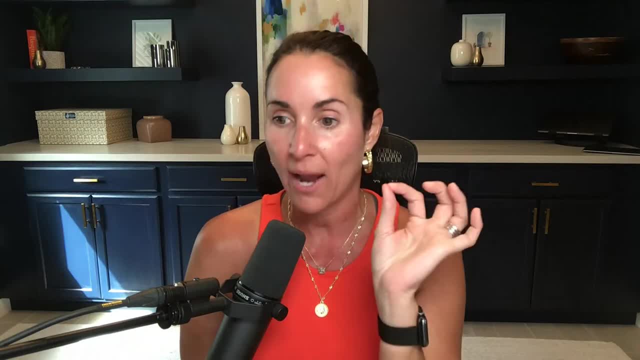 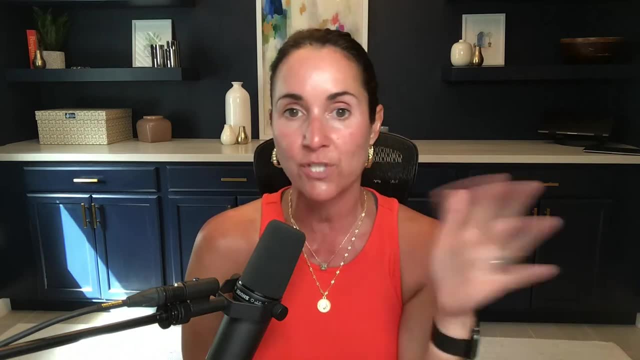 sure you read that last sentence, because that'll show you what they're actually asking. very good point. my team. i test at home and use a whiteboard too. yeah, so whiteboard mia some people. it just depends on where you're testing and what um place you're testing at. when you say one week, how many? 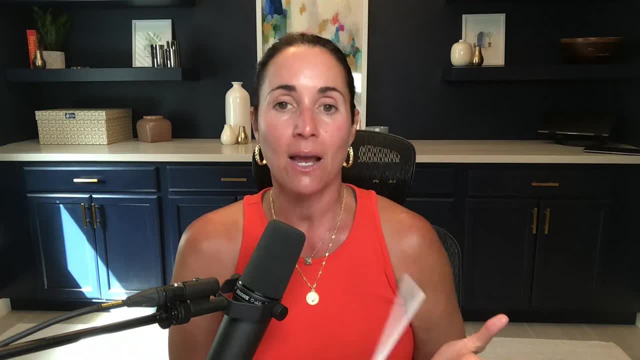 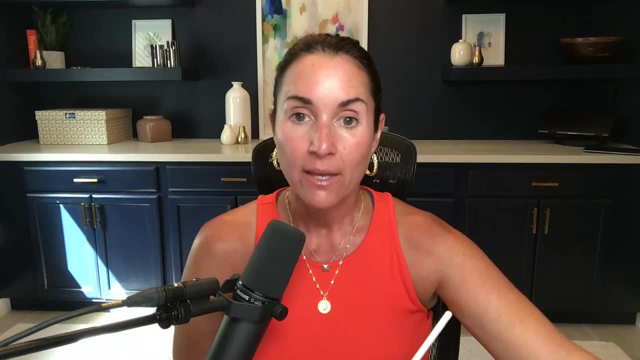 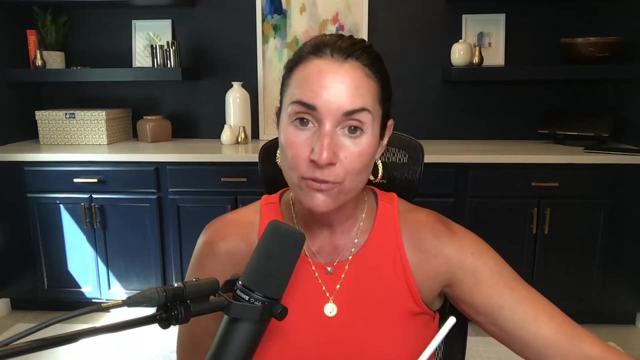 hours in, okay, so, um, a lot of people ask exactly how many hours they're supposed to study. it depends on your skill level. like for math. this could just be a brush up session for you and you're good to go, or you could have struggled with math your whole life and you've got a lot of work. 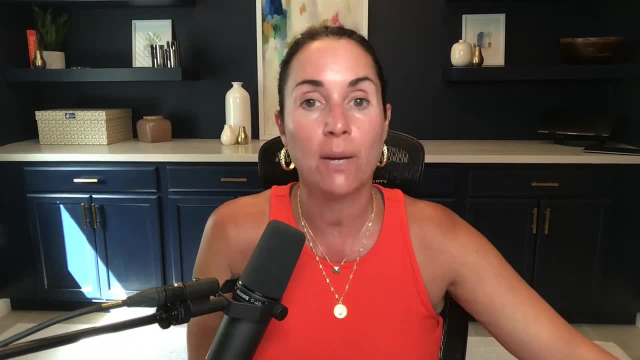 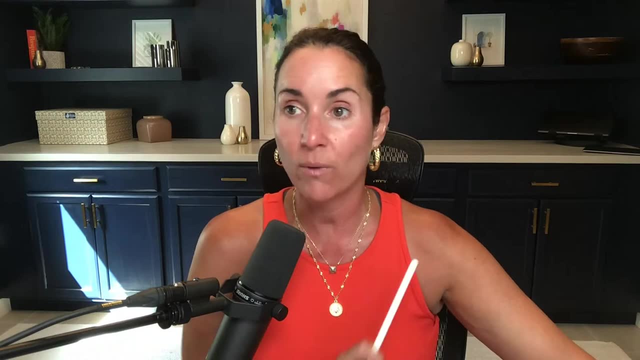 to do. it just depends. if you're just kind of brushing up on everything, i would say 30 to 40 minutes a night, that's it. you do not have to spend four hours a day on this and i don't recommend that. it's too much. 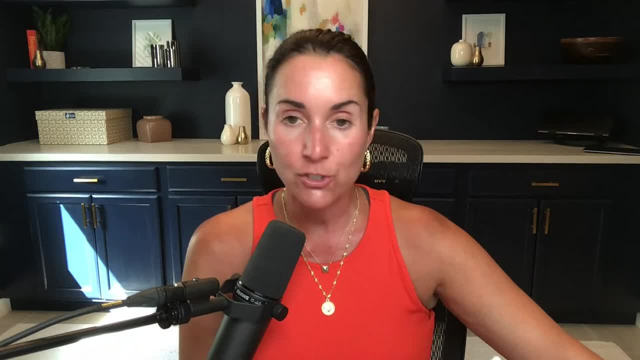 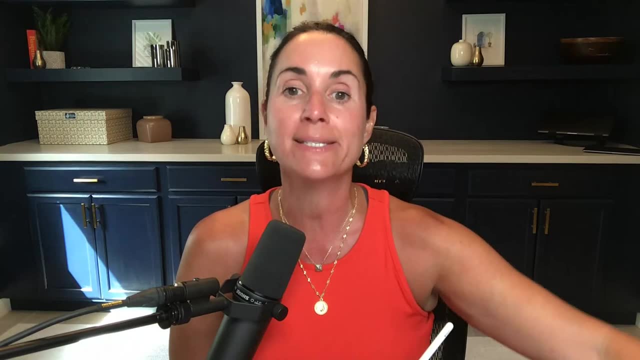 30 to 40 minutes a night. read a section: do the practice questions move on. read a section: do the practice questions move on. then i would dedicate some time to the actual practice tests, the big tests in the back of the book, because i do have those mini, mini quizzes at the end of each section. 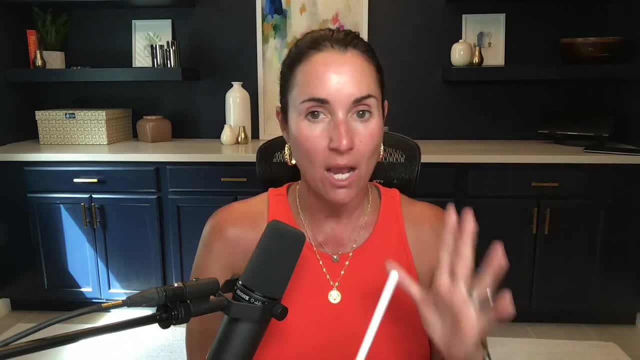 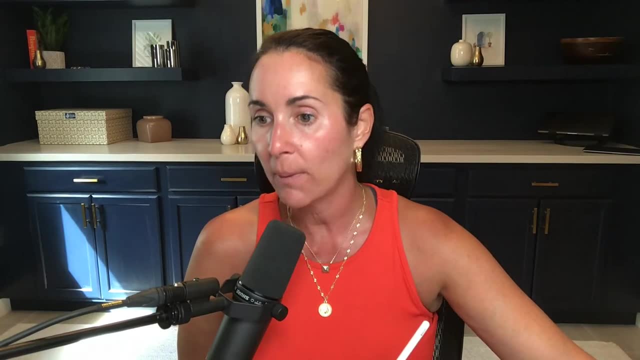 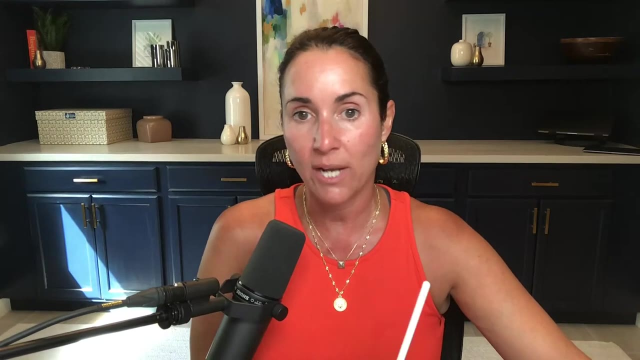 okay, so just break it up one section at a time and it's broken up that way. okay, should i schedule the test two weeks out for each to give myself time to prepare? i think so two weeks is good. yeah, and stick to it. 40 minutes a night. 30 to 40 minutes a night. put it in your calendar, tell your 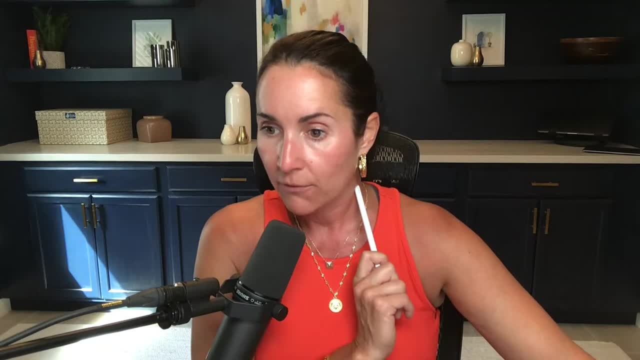 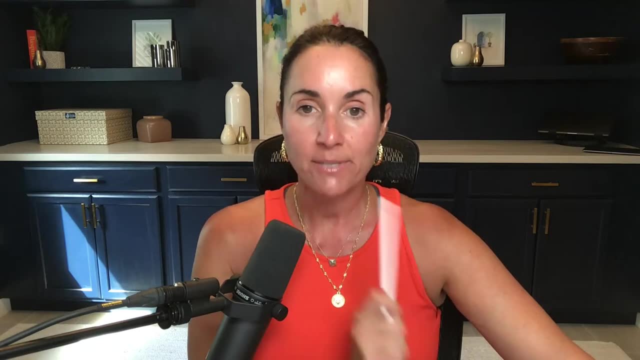 family. do not bother me. i am studying for my exam. for those of us who are intimidated by math and have test anxiety, do you have any additional tips? all right, brandy, good question. we have to stop telling ourselves stories about math. those of you have struggled with math i understand. and we say: 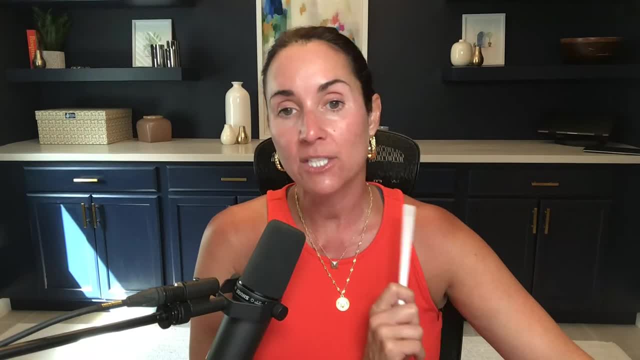 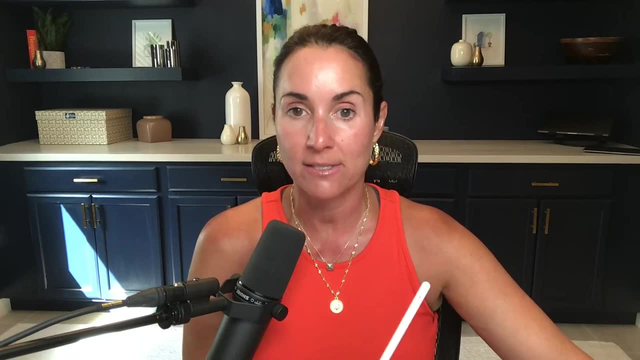 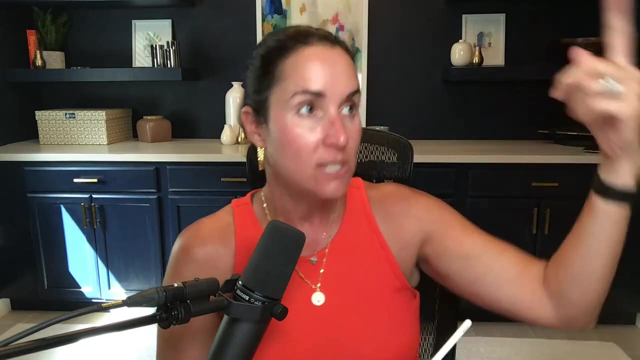 things like i'm just not good at math, or i'm english brained, not math brained. that's not true. we're telling ourselves those are lies. everybody is both brains. we can be a math person and an english person. in fact, some of the greatest philosophers and writers and artists were 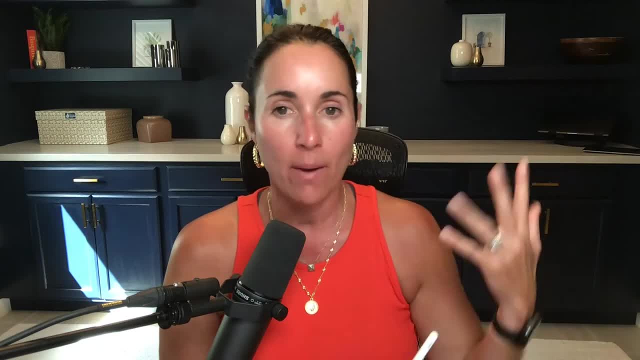 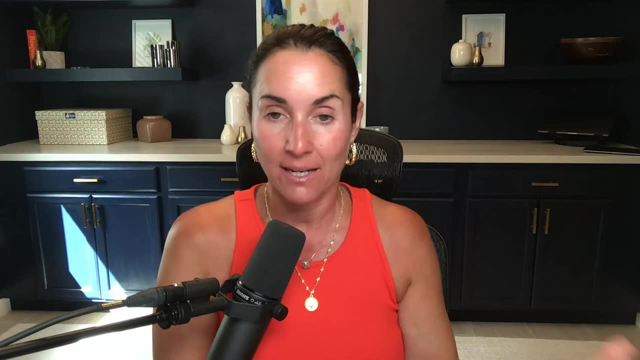 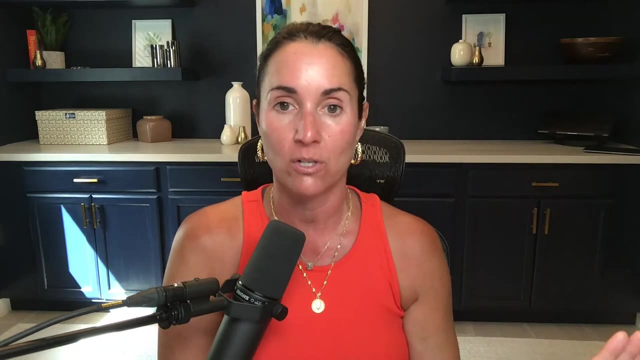 mathematicians. so that is a- i don't know where it came up- left brain versus right brain: we use all of our brain all the time. okay, now you might have had more success in english language arts or opposite. you might be someone who have has found a lot of success in math and not in english language. 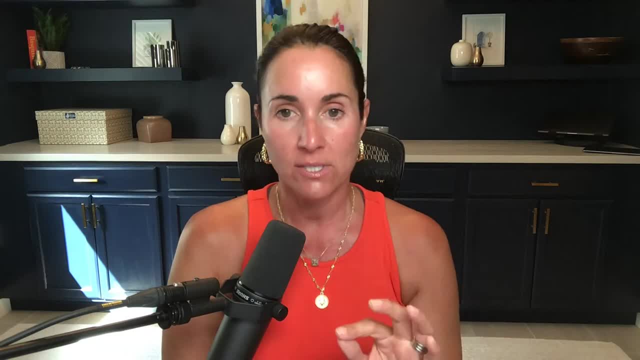 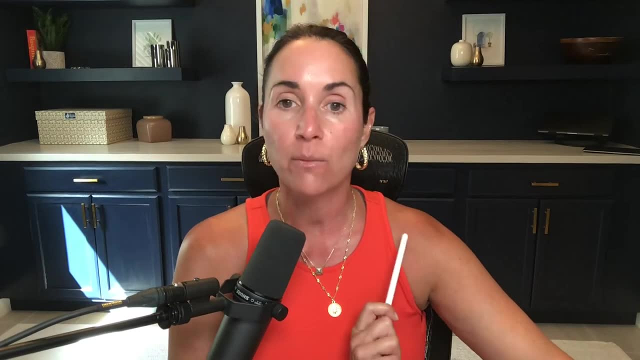 arts. but i would recommend stop telling yourself those stories and start saying: as soon as i brush up on this math, i'm going to be better at math. i'll give you an example. i thought i was an english language arts person. i thought i was not a science person. growing up, i did well in english language. 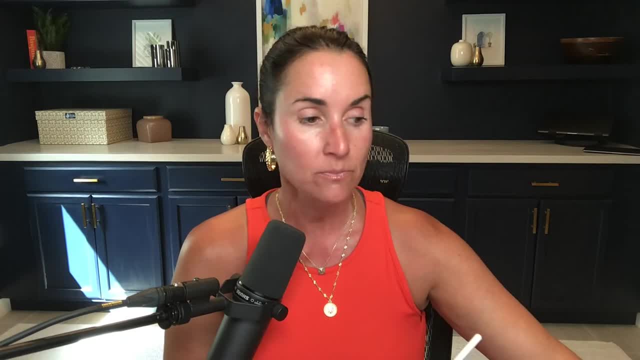 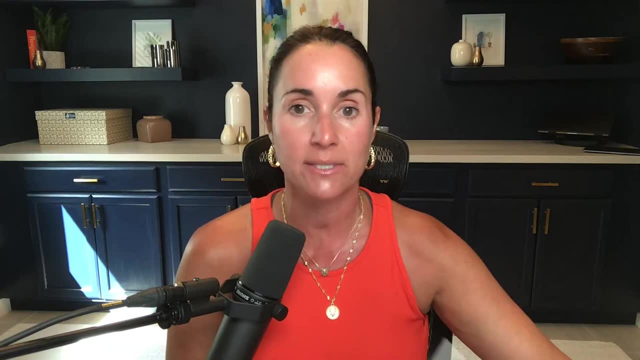 arts i studied in college. i did. i got a degree in english. my bachelor's degree is in english. then i became a teacher and the only open spot they had was biology, my worst subject in high school. so i studied it. i stayed ahead of the kids. i ended up really enjoying it and i started to 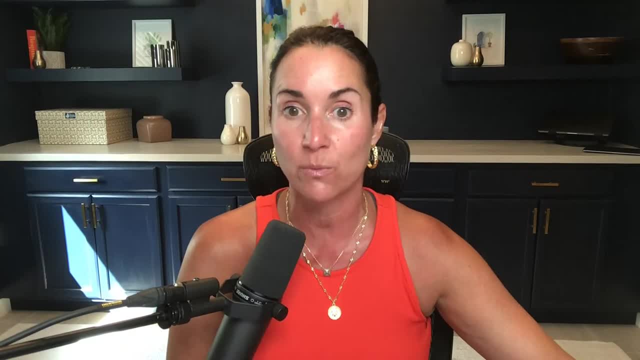 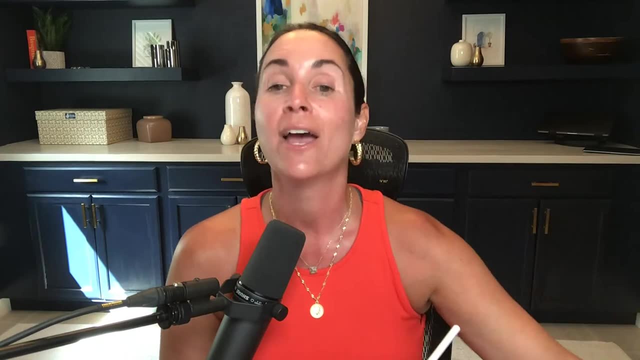 learn a lot and my scores became some of the best in the building, some of the best in the district, because i worked so hard on those- my scores for my kids. i also bribed them with chicken sandwiches from chick-fil-a, but that's another story. we worked really hard and we learned a lot together. 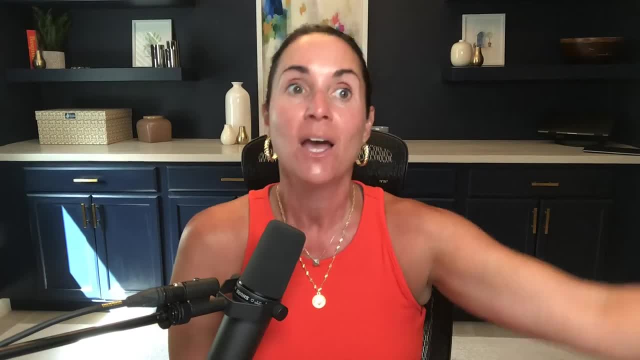 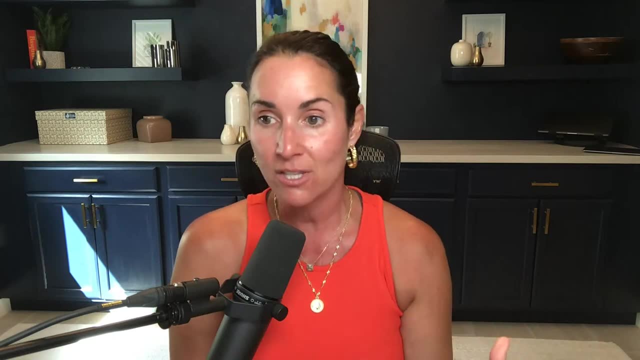 and i learned- it isn't that complicated- that i can be a science person and then i became a science teacher. i love science, so stop telling yourselves those stories. for test anxiety. here's the thing. you guys. lots of people have to take this test more than once. 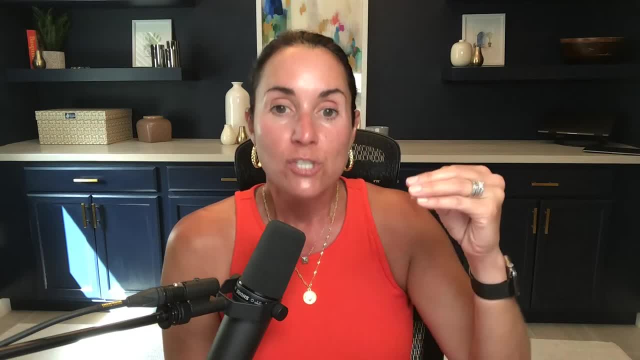 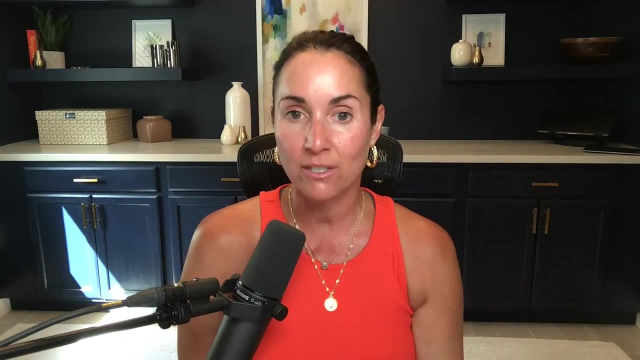 it's uh hard, it's a big test, okay, so just take it and if you're not successful, take it again. you're not going to die, nobody's going to put you in jail because you didn't, because you didn't pass, just take it again. it's expensive, i know, and that is problematic and there's nothing i can do about. 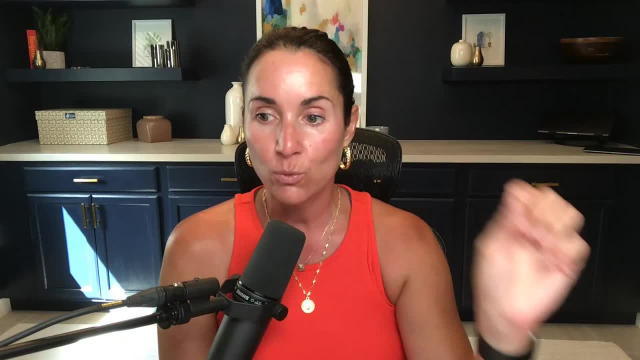 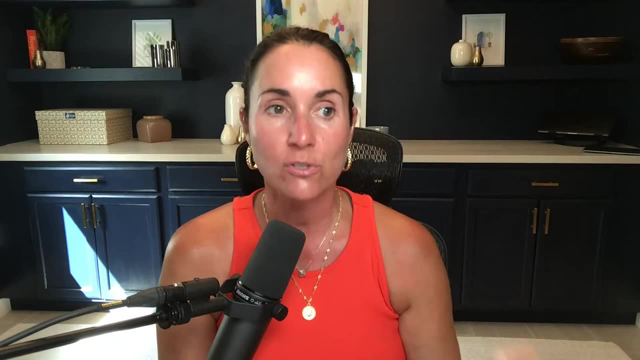 that, but you just take it again and talk to yourself the way you would talk to your students. hey, i know you can do it next time. i think you should brush up on this. start to learn those skills. work on that math. start to learn those skills. work on that math. start to learn those. 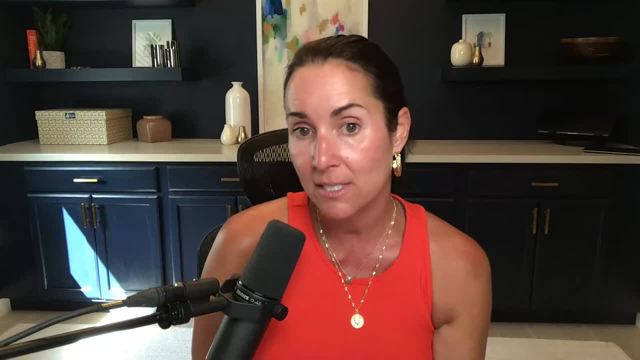 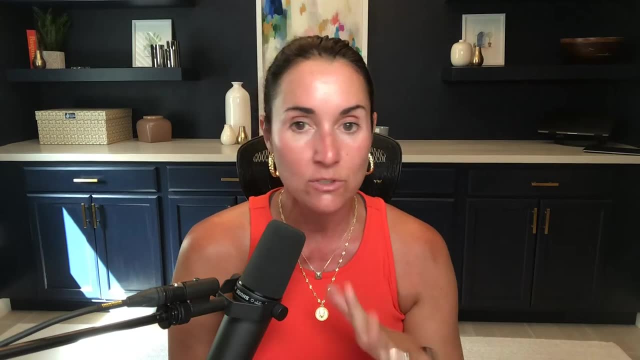 use my products. use khan academy. use released act tests. grab a book from your, from the math teacher at your school. start to work through those problems and you will get it. never say to yourself: i'm not a math person. because you are a math person, you've just had more success in. 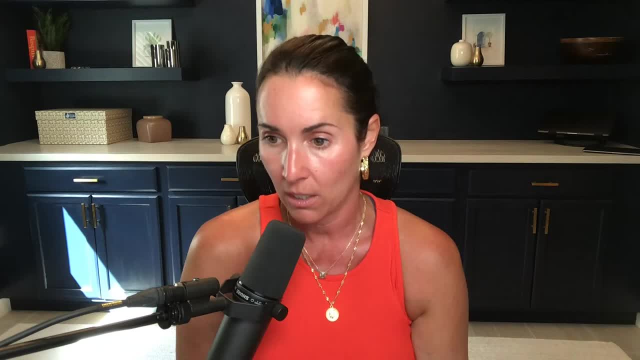 another area. it's time to have success in math. you can do it, i know you can. uh, jonathan, do you have online testing? in the online materials? does it tell a person's weak areas after the test? is the test the same questions or will it be different every time? okay, jonathan. 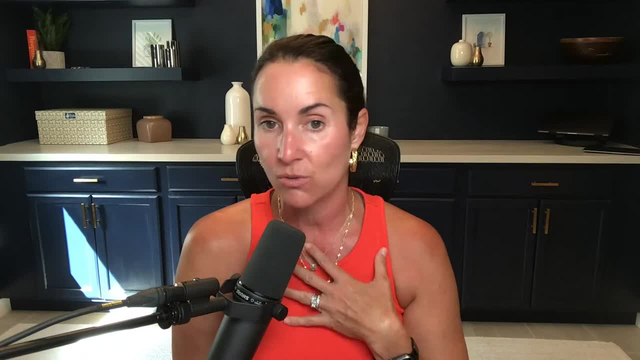 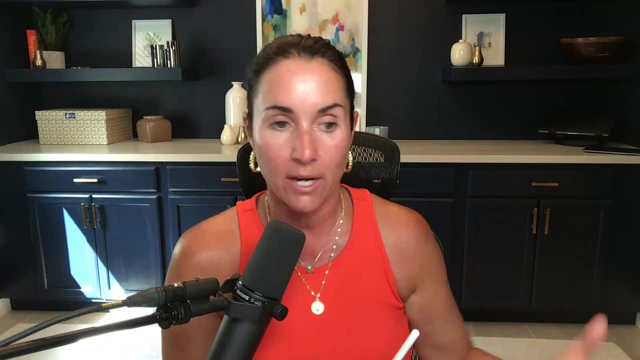 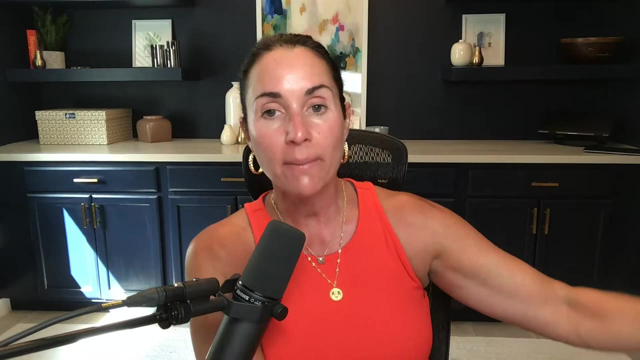 the questions in our tests, in our practice tests, do not change. we're not pearson, we're not ets. we don't have hundreds of test item writers to just keep writing different items. we do have additional questions in the online course and they are facilitated online. i recommend using 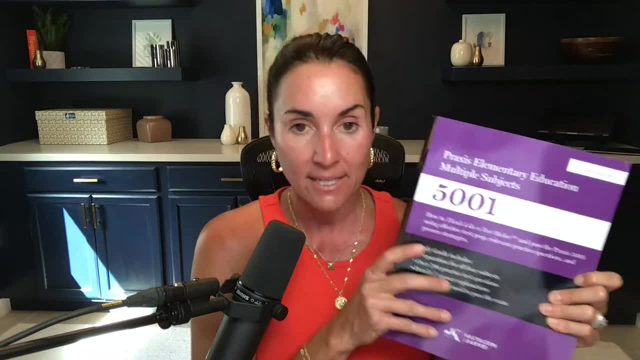 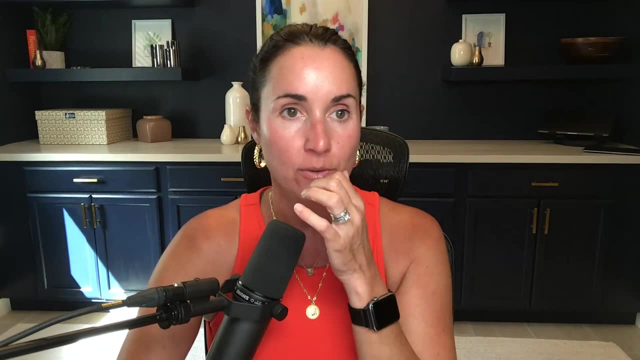 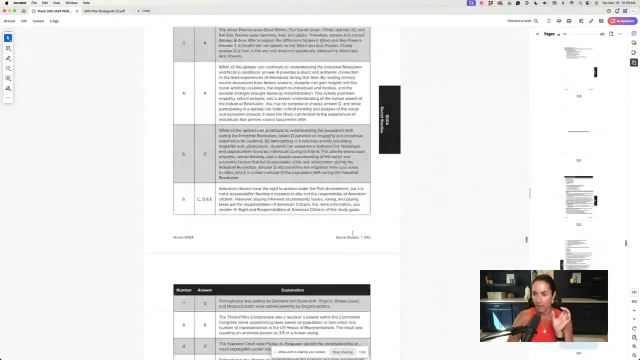 the study guide to see where you are low. because in the study guide let me show you real quick, just so you guys can see something here. uh, let me go here, let me show you how to do that. okay, so let's say: i am in, let me go to math real quick, because everybody's talking, talking about math. so 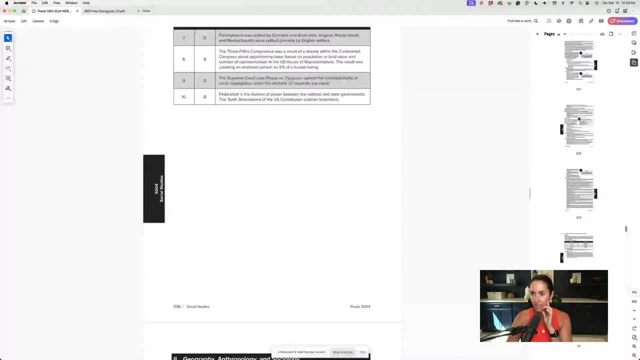 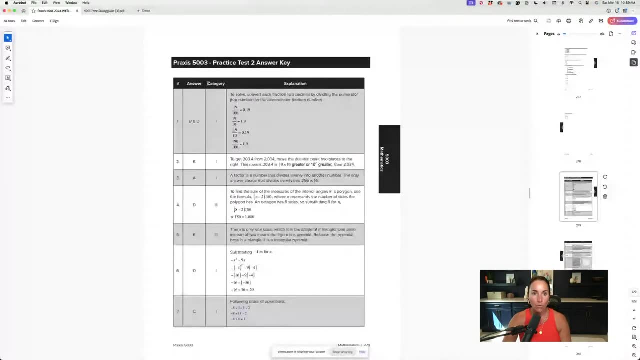 let me just scroll. oh, math is up here. sorry, i've been working in a lot of different study guides. okay, so you can see here in our answer explanations for math i always have what category these questions come from, so you can see if you're missing a lot of questions in section one. you 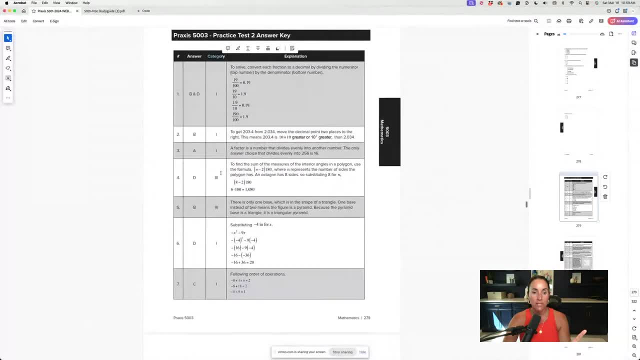 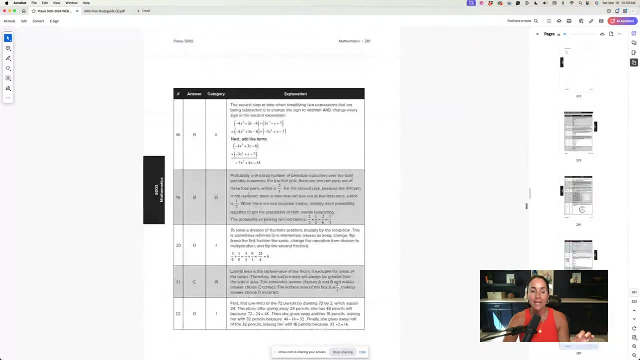 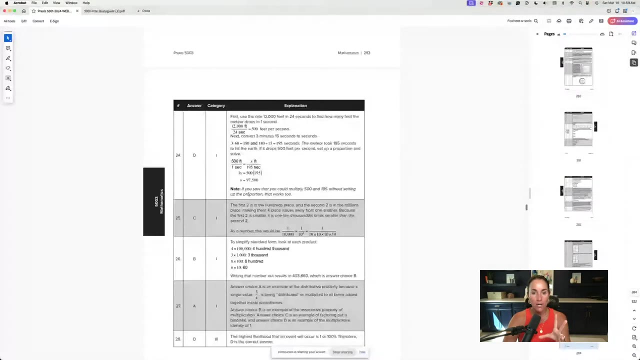 need to go back and work in section one. okay, if you're missing a lot in section three, you need to go into content category and work on those. i try to keep them in somewhat of an order, but it's hard because they assess a lot of different things and some questions assess more than one content. 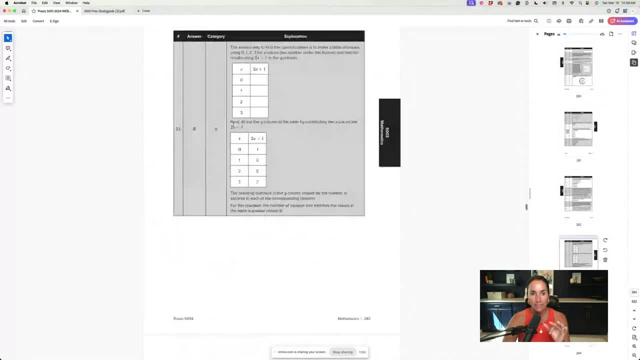 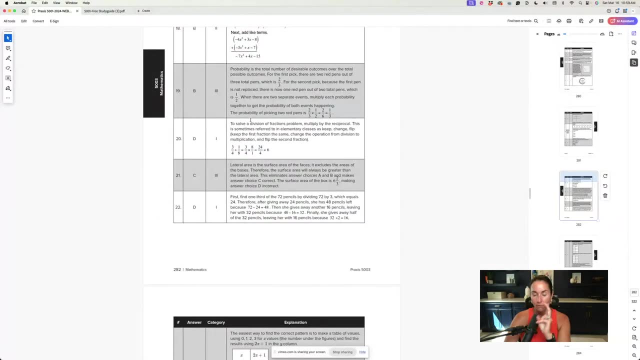 category, i try to go with the main one. so if you, i would use the practice test after you've studied all the material when you go in and take your first practice test. there are two for each content or for each sub test. so let's say i just finished math and i do my math practice test. okay, and i'm. 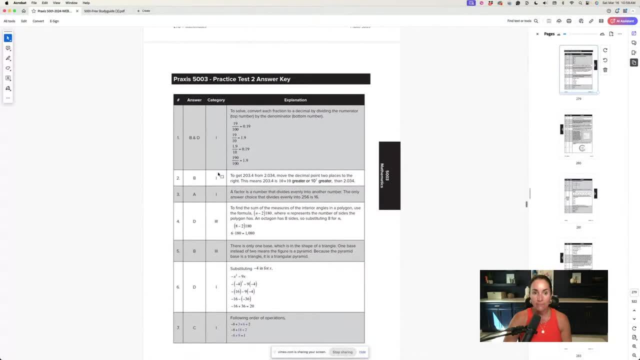 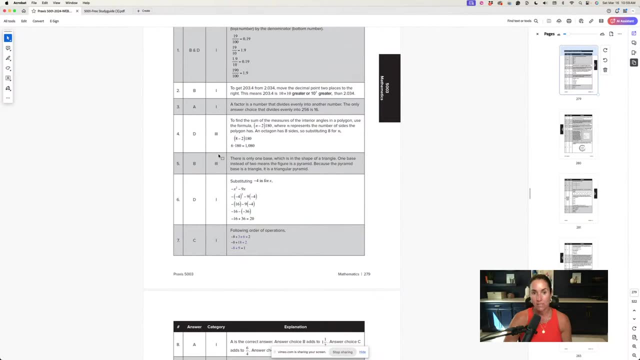 grading it. pay attention to this category here. If you've missed a lot in section three, like you've missed 70% of the ones in section three, you need to go back to section three and fix it up, go back through, work through. 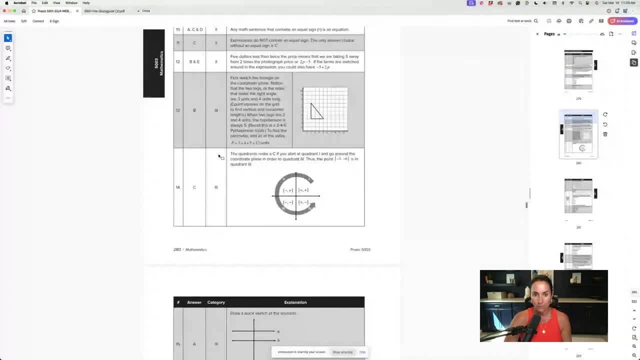 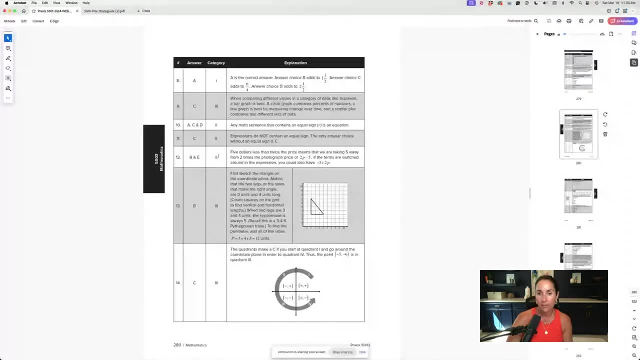 it and then retest on practice test two And that'll help you. Okay, Now on our online course. we don't just have an infinite amount of questions that keep changing. We don't have that capability. I wish we did. I would love to have a hundred item writers, like big testing companies, do We just? 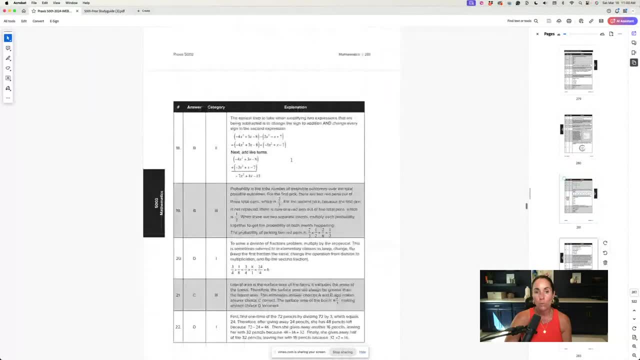 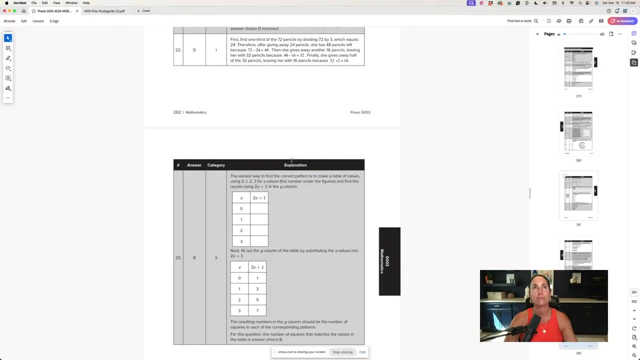 don't have that. It's me and a couple other people on my team, So we have a lot of questions. There's over 700 practice test questions in this book. There's over 500 or four- no, not 500.. There's. 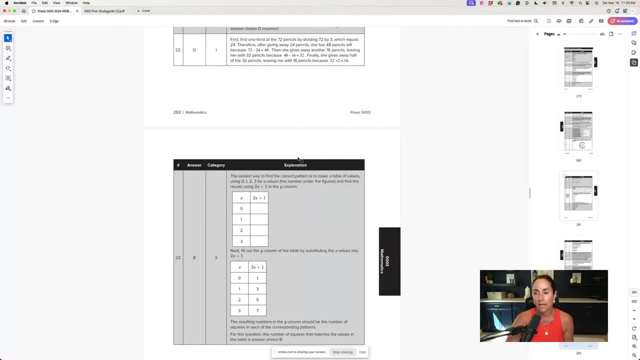 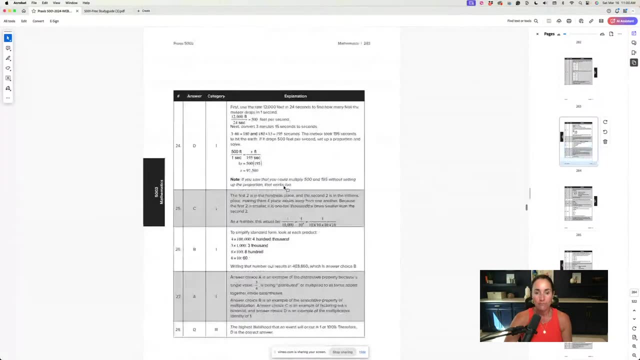 over like 300 for the math alone. I mean I there's not many more I can give you on that. All right, But you can always use ACT. You can always use other books as well for different questions. Okay, So that's how I would do that, All right. Thank you so much. 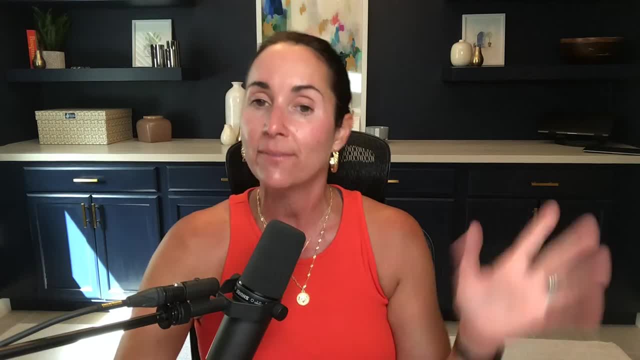 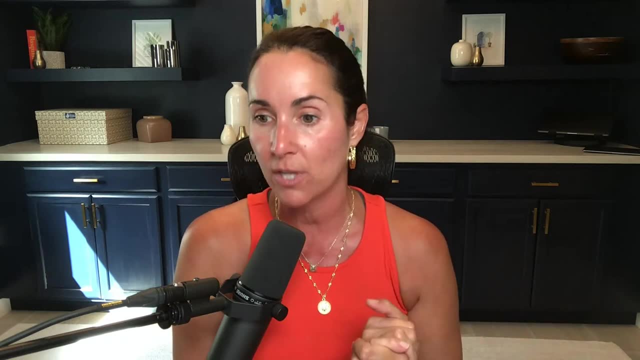 Thank you, Maria. Thank you, Thank you, Rosa. Helpful Helping please with 5025.. Okay, Rosa, we have a webinar on that, But we're talking about the 5001. today I'm having a lot. I have lots of webinars on different ones. Check out our webinars. 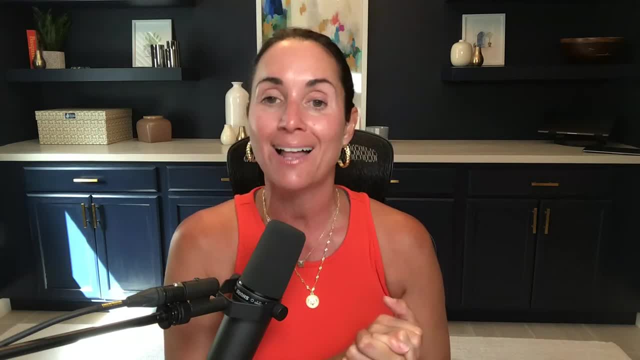 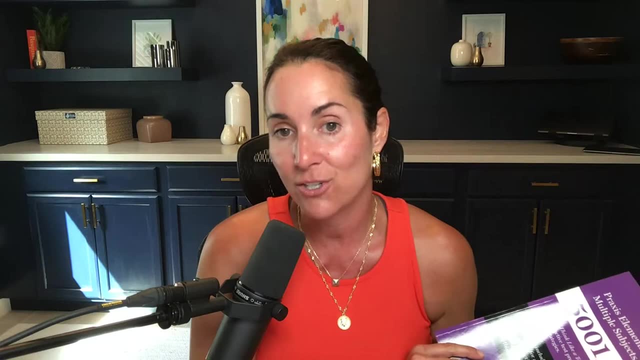 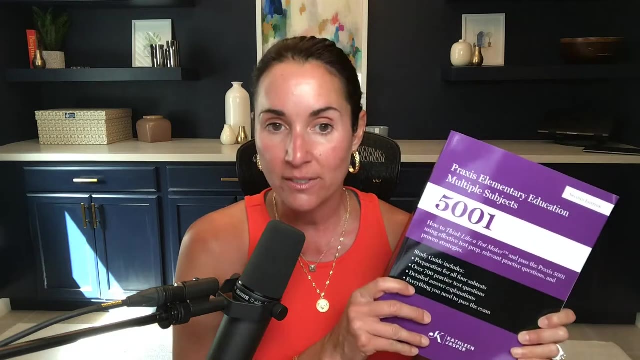 page. Do the videos explain each question? The videos explain a lot of the questions. They don't explain everyone in the 5001 because there's 700 questions And I couldn't. I couldn't do that. So most of my online courses I explain all the practice tests. for this one It's just, I mean. 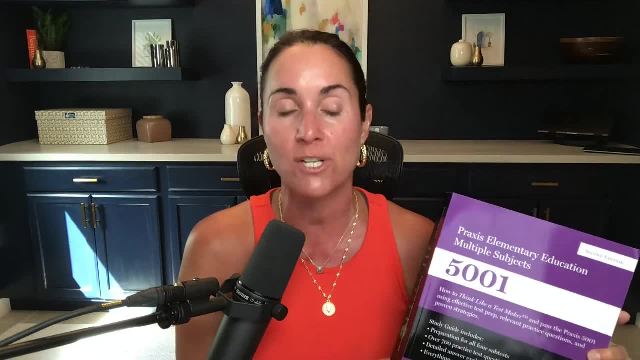 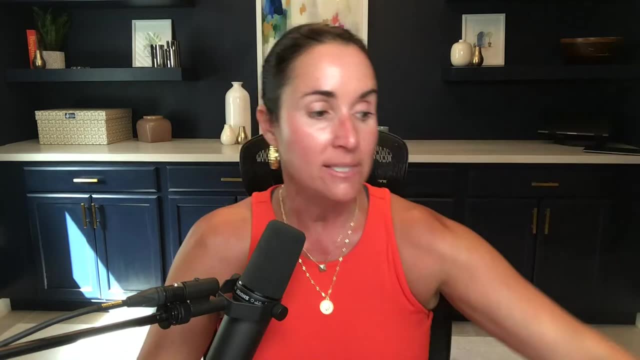 I, I couldn't do it. So I go over the skills and I go over some of the harder questions, but I don't have a video explaining every single question. but we do have detailed answer explanations in here. Okay, All right. Now let's get to the other one, because we have somebody. 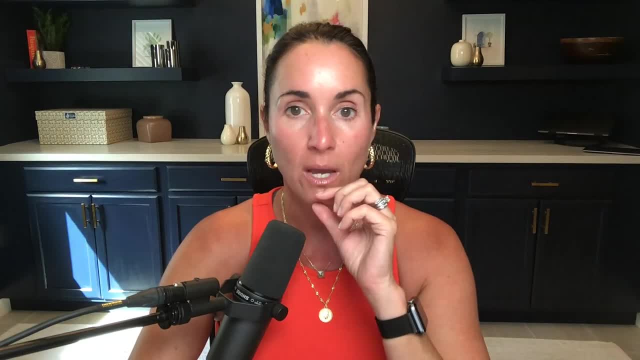 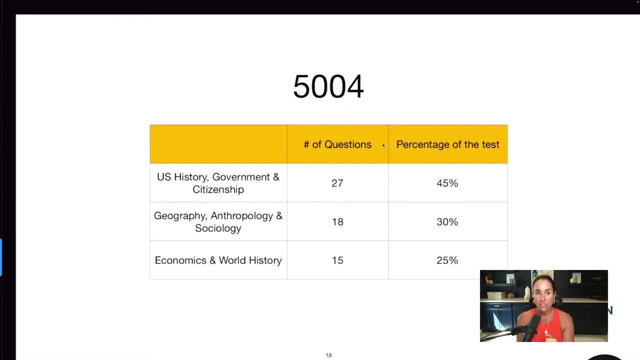 taking this exam soon, So I want to go over the. let's go over the social studies. All right, Social studies is mainly memorization, but remember, I don't know what tests you're going to get, And so we need to make sure we understand these concepts a lot. So there are three main 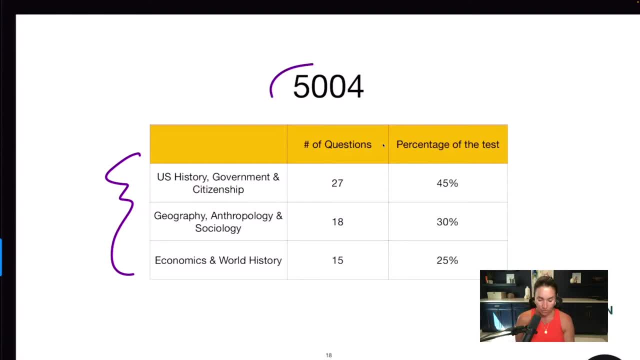 content categories in the 5004 sub test. This is social, social studies. Okay, First we're going to have us history, government, government and citizenship. This is all about European exploration to the Americas, indigenous people, what happened and and and what Europeans did. 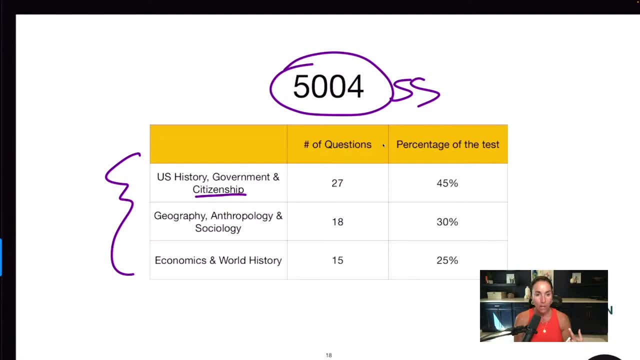 to them: slavery, the colonies, the American revolution, the stamp act, the T act, the, the articles of confederation, the declaration of Independence, the Constitution, the amendments, three branches of government. It's got a lot, This. 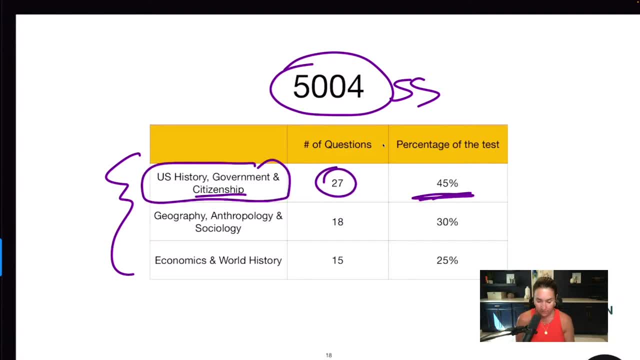 is the biggest part of it right here, You can see, at 27 questions, at 45%. Now again, I don't know what questions you're going to get on that. I have covered everything in the specs, but you have to be able to understand these sections so that, no matter what you're asked, you can grab it, because 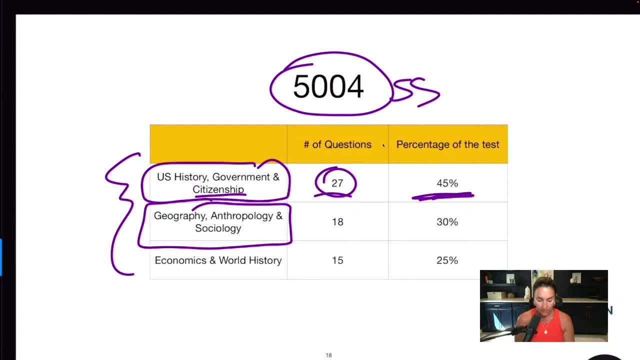 you have that information. Okay, Then the next one is geography, anthropology and sociology. So this is going to be things like, you know, longitude, latitude, maps, things like that, but also about people, different types of people, and anthropology and sociology, languages, how people farmed. 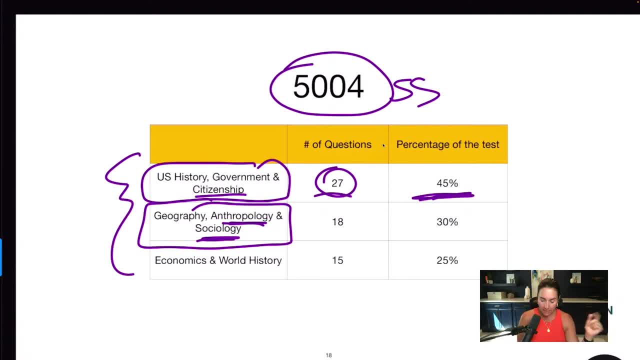 how human societies developed, things like that. Okay. And then the last part is econ and world history. They lump those together for the elementary grades. As you go up in the grades like middle school, these are sectioned out. In high school they're also sectioned out. 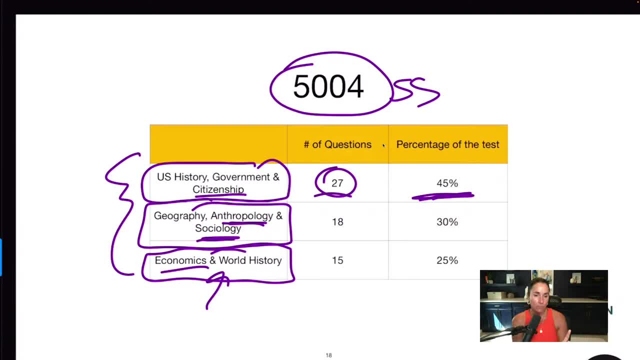 But for this they're together. So economics, basic principles, nothing too crazy: supply and demand, Price floors and ceilings, Opportunity, cost, things like that. And then world history. I mean anything from the Paleolithic era all the way up to the 21st century. It's a big category, So you. 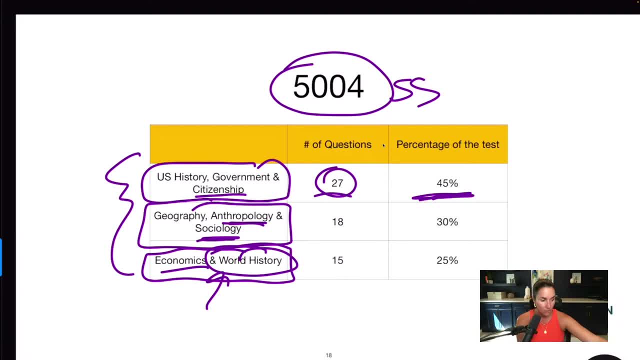 got to kind of know that Timelines. I have a lot of timelines in my book and major things that have happened, But again I don't know which ones they're going to pick for you guys, It's history, It's infinite, right? So there's lots of different questions that we can do, So let's talk about. 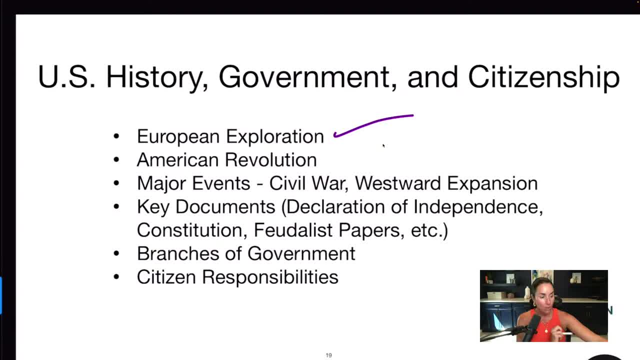 US history. We talked about this already: European exploration coming over on boats exploring the New World. Why did they? They were looking for the passage between Europe and the Orient, So they were looking for the Northwest Passage and they got. 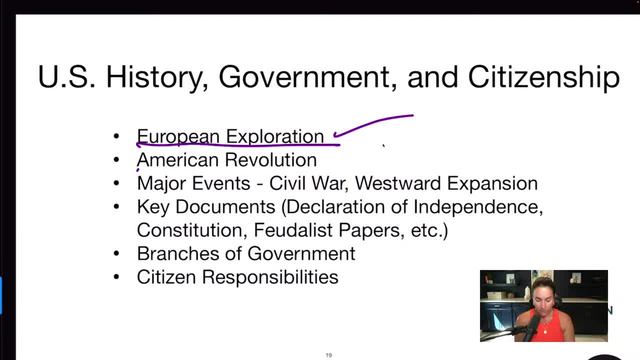 the Americas instead. Then, as we colonize- and I say we, because I am from European descent- but as Europeans colonize, American Revolution takes place. Then, after that, major events: Civil War, wayward expansion or westward expansion. key documents: Declaration of Independence Constitution. This should say Federalist. 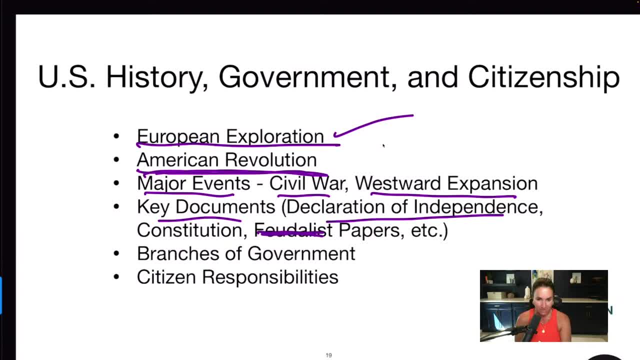 Papers- Sorry, that says Feudalist Papers. It should say Federalist. I mistyped there, Sorry about that. Branches of government and then, of course, citizenship. This is civics. A lot of information here. Let's have a look at a question. This is number one on page 16.. All right, so we 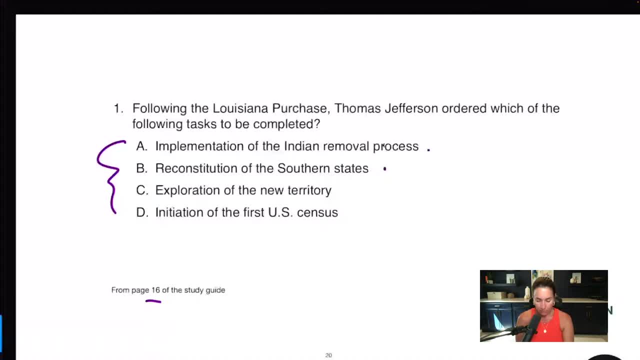 have: implementation of the Indian removal process, reconstitution of the southern states, exploration of the new territory, initiation of the first US Census, Can't do much there. Let's read the question: Following the Louisiana Purchase, Thomas Jefferson ordered which of the following tasks to: 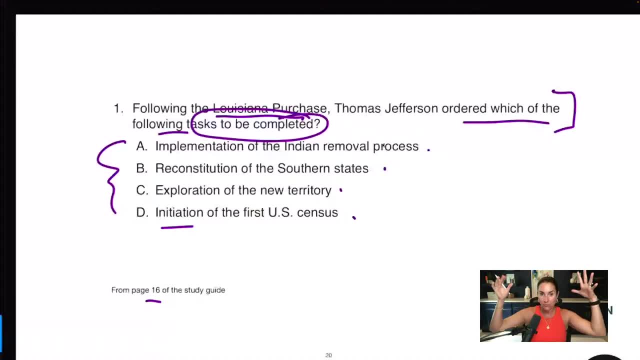 be completed Now. remember: the Louisiana Purchase was a big purchase from France. It ranged all the way down from Louisiana over I can't remember exactly where over, but then up all the way into Canada. So we got all this new land. What do we need to do? We need to explore the new territory. and if we got even more specific, this was the Lewis and Clark Exploration. This is where we went out west, started to go out west and explore that new territory, all right, and see what it had to offer us, as you know, colonists. So that's C. 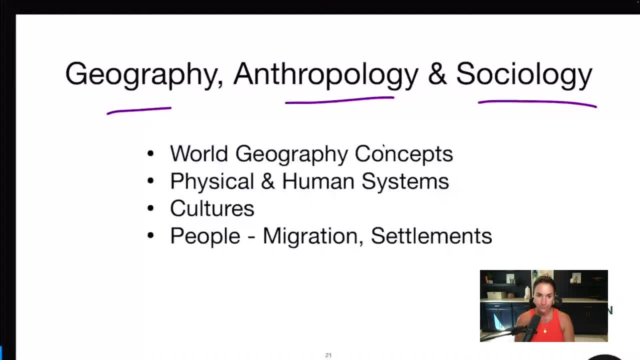 Let's have a look at geography, anthropology and sociology. So we've got world geography and concepts, longitude, latitude, prime meridian, equator, things like that- Physical and human systems. So physical systems are things like the world doing its thing or the earth doing its. 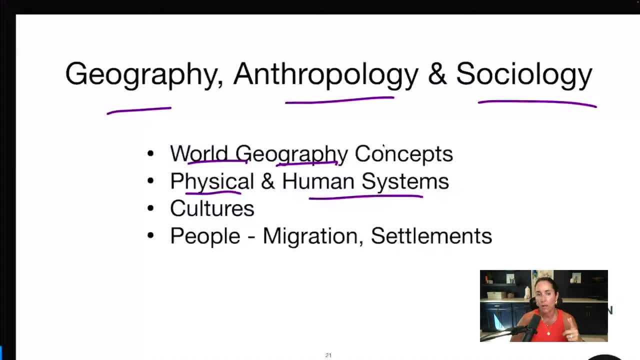 thing, Seasons, and all that ties a little bit into science as well. Volcanoes, mountains, mountain ranges, things like that Ring of fire for earthquakes and stuff, And then human systems. How did humans move around the earth? How did they farm? How did they like? did they use terrace? 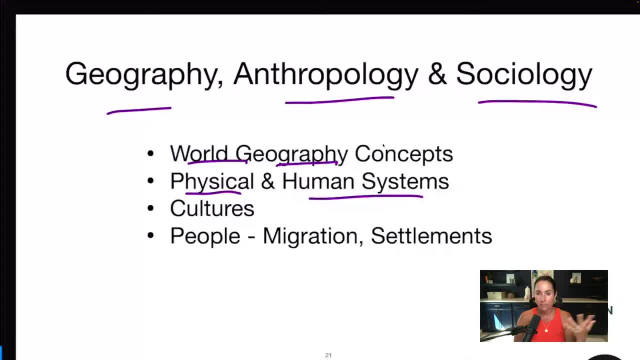 farming versus irrigation versus whatever, And how did we make these human systems? How do we communicate Stuff like that? Cultures of course goes in with that. human systems, And then people, migration and settlement. So it's all about the geography, but then of course the anthropology and the sociology. 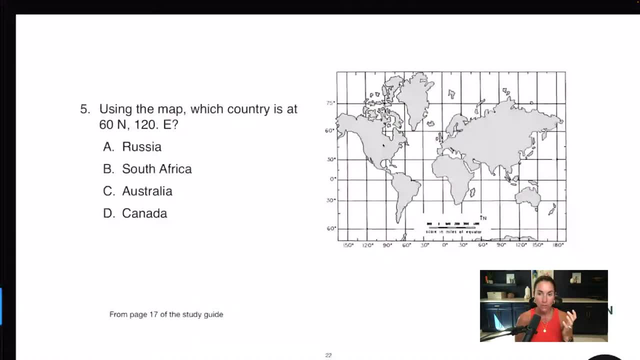 So let's have a look at what a question might look like here. So we have a map. So it says, using the map, which country is 60 degrees north and 120 degrees east. So I got to use my longitude and latitude here. 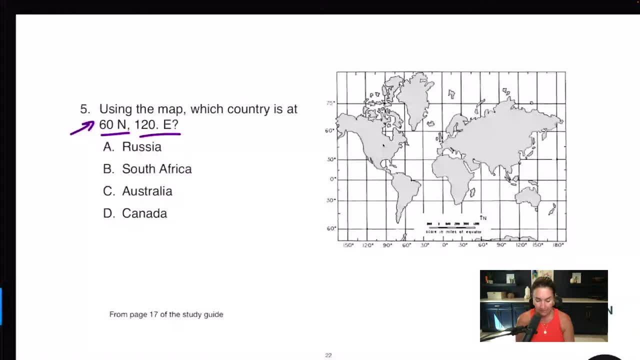 So I need to know that the first one is longitude and the second number is latitude. So if I went 60 over to 120, we'd be here. This is going to be Russia. Now, this one seems pretty easy, but they might say something like: 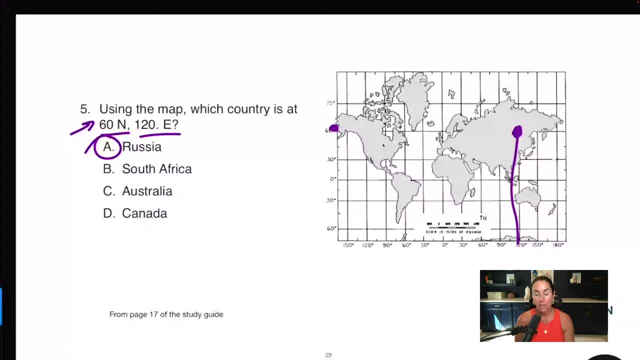 which country is in the northeast hemisphere? You would need to know your north, south, east, west hemispheres. You know there could be a lot of different ways in which this is asked. So this is just a longitude latitude exercise. 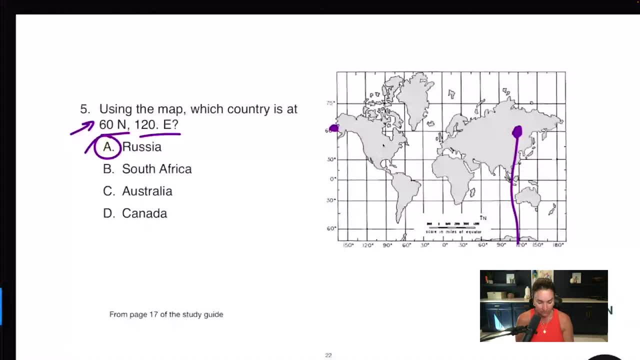 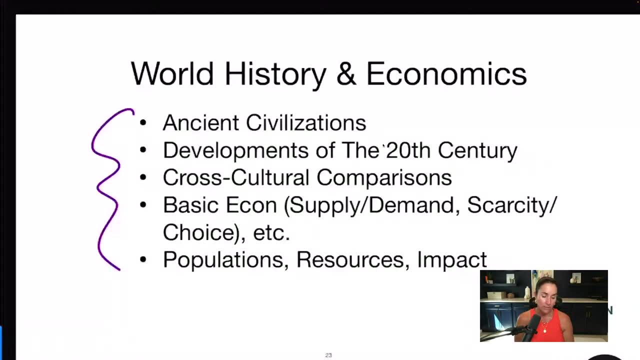 But you may have- it may be asked a lot of different ways. So make sure you understand that. Now let's talk about world history and economics. So we're going to have ancient civilizations. These are like the Romans, the Mesopotamians, the Egyptians. 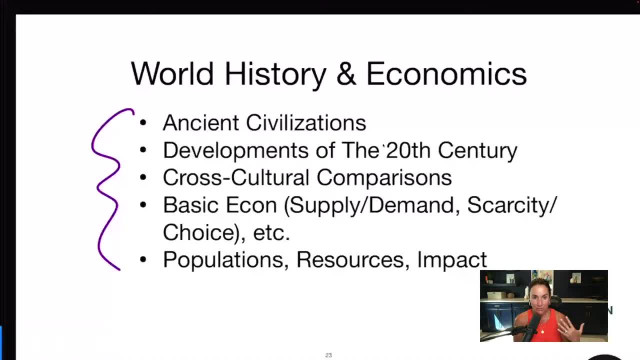 I mean, this goes back a long time and it's going to go all the way up to the beginning of the 21st century. So we're talking a lot of stuff happening. I try to break down the most important parts, but it's everything from the world wars. 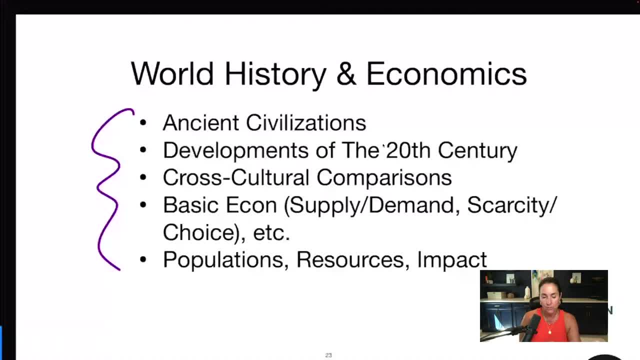 the civil war. even though that's covered in US history, It's also a piece of world history. World War I, World War II, the Cold War, stuff like that- Those are all developments of the 20th century. 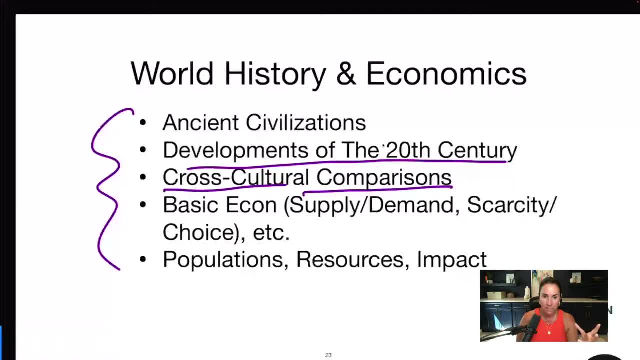 Cross-cultural comparisons. what was going on in these different ancient civilizations. Then we're going to get into economics. We said this before: basic econ: supply and demand, scarcity, choice, opportunity costs, things like that Push-pull factors why people emigrate and immigrate to other countries. 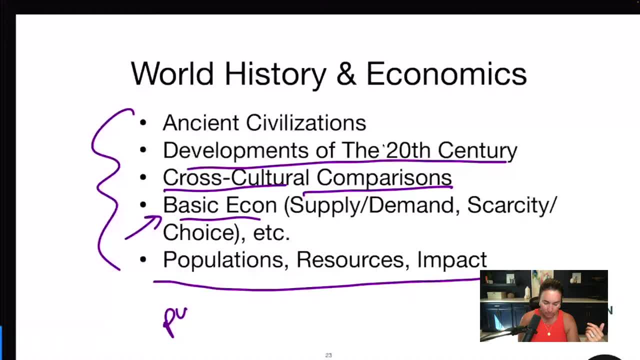 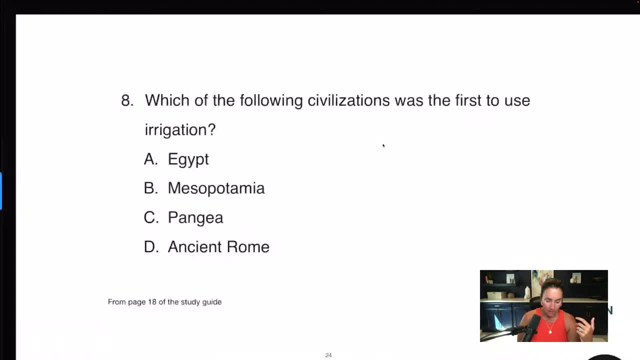 And then, of course, populations, resources and impact. That has a lot to do with the push-pull factors: Why do people leave? Why do people leave And why do people come? Typically economics and a better life. All right, let's have a look at this particular question here. 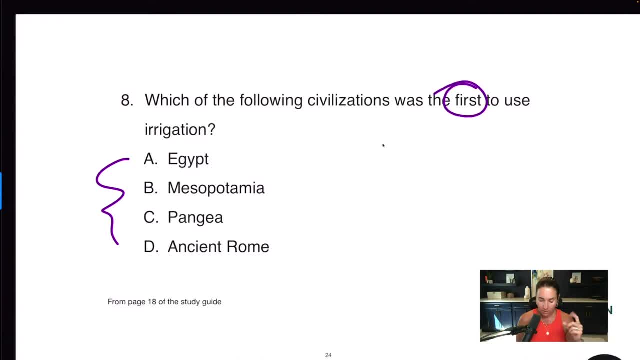 Which of the following civilization was the first to use irrigation? This is kind of a tricky one. Mesopotamia was the first to use irrigation, but Rome actually perfected irrigation later. But it's asking who was the first, So B is the best answer, but be careful: Rome did perfect irrigation to have these systems. 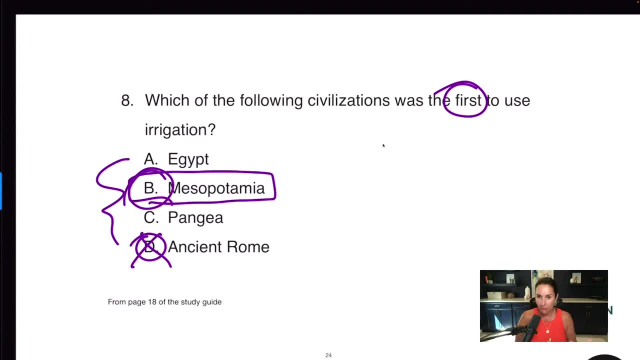 of pipes and things like that for their farms. So just be careful with the question. I hate how they lump these together because sometimes it's not clear If you see ancient Rome and Mesopotamia together and it's about irrigation, make sure you see. 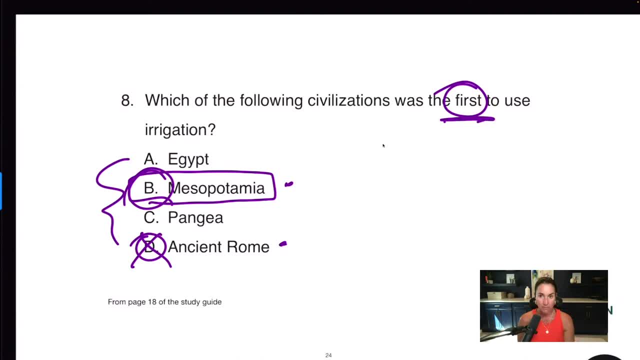 what they're asking you. If they're talking about the very first people to use it- Mesopotamia- If they're talking about the people who perfected it, it's going to be Rome, all right, And Pangea is not a civilization. 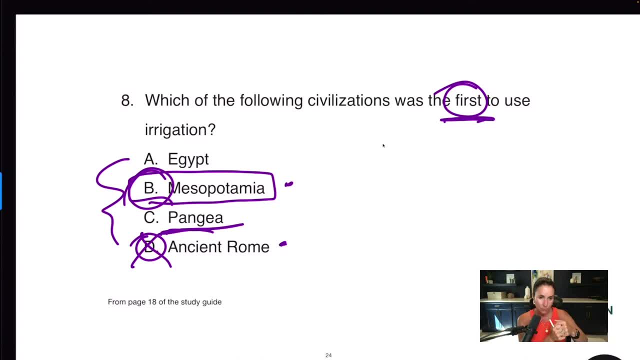 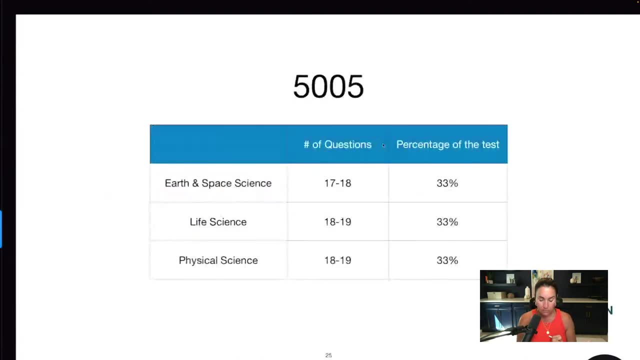 Pangea was when the earth was all connected, all the continents were connected And then they broke apart. That's Pangea, or continental drift. We also cover that in science. Speaking of science, let's move on to science 5005.. 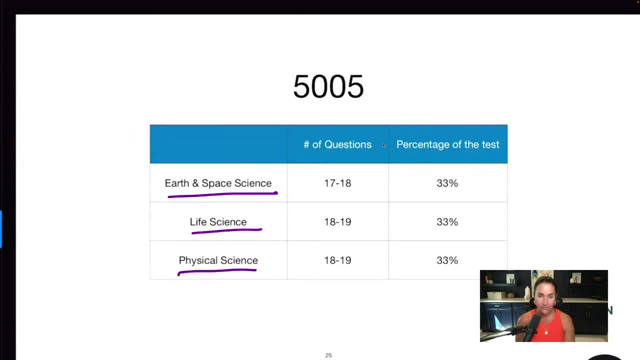 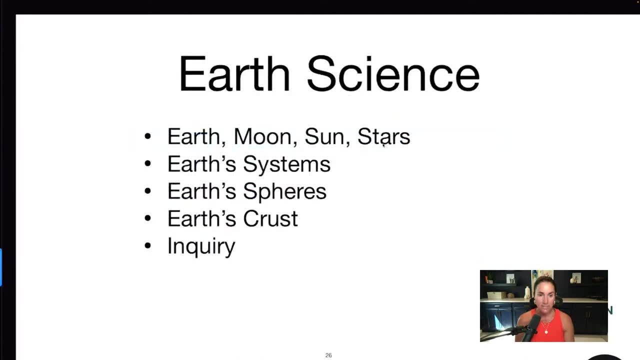 Three content categories here: earth space, life and physical science. So they're all pretty much the same: 33,, 33,, 33.. So earth space science is the earth, moon, sun, stars, earth systems like the water. 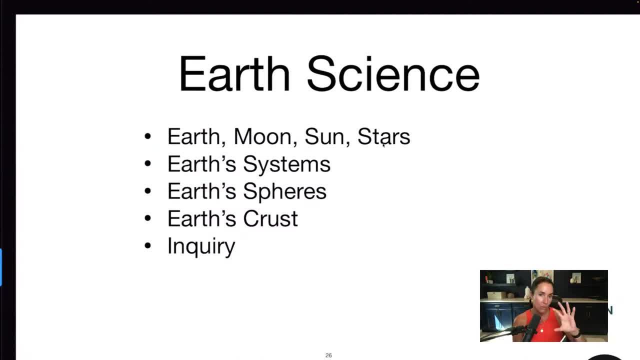 cycle and earthquakes and its rotation, And it's revolution around the sun. Those are all earth systems. They cause seasons, they cause all kinds of things: weather, all that different stuff, Earth spheres, the cryosphere, biosphere, hydrosphere, atmosphere, all of that. 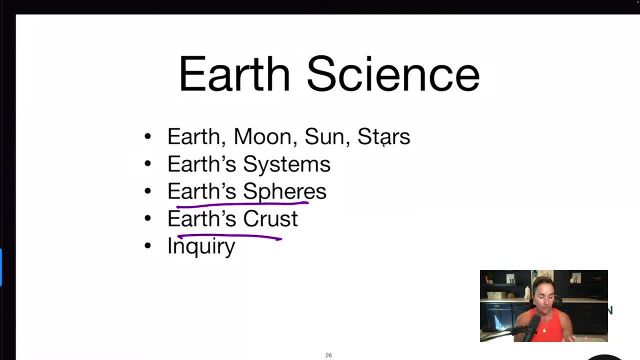 Earth's crust, the lithosphere- that's going to include mountains, canyons, anything on the top of the earth, bedrock, soil, all of that, And then, of course, in all of these We want to make sure we're fostering a student's inquiry. 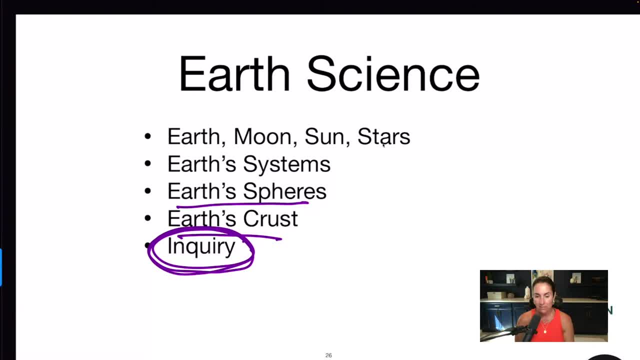 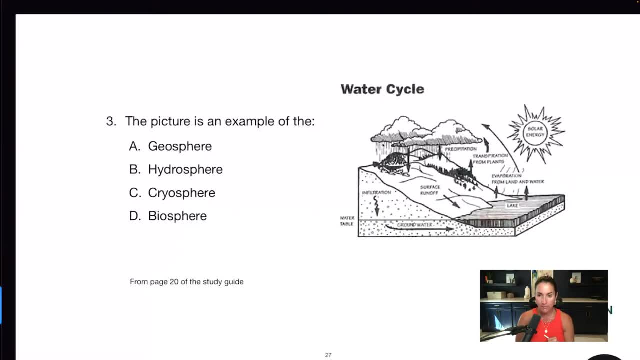 Science is all about asking questions using the scientific method, testing hypotheses. We always want students to be inquisitive, So anything that has to do with inquiry is going to be a good word on this exam. Let's have a look at the water cycle here. 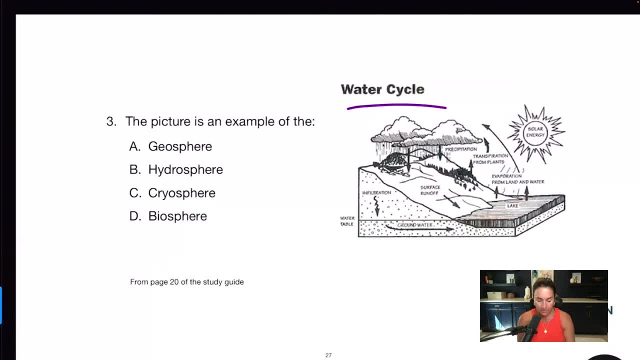 I can see that's going on here. The picture is an example of this- is the hydrosphere, So anything that has to do with water is hydro. Hydro means water. Geosphere is anything that has to do with, like, the minerals. 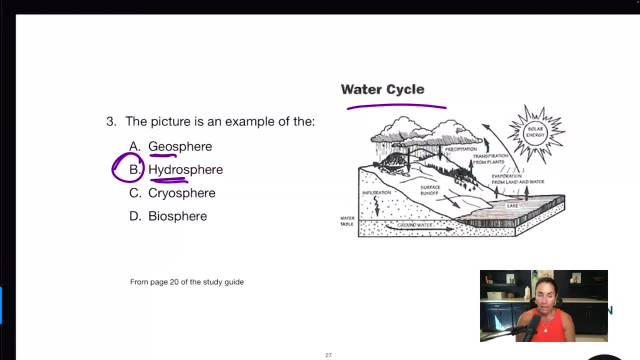 In the ground like a geologist. Cryosphere is all the ice on all the frozen water, all the ice on earth And the biosphere is anything living? So we want to make sure we know that. You can see, we've got precipitation, transpiration, condensation, runoff. 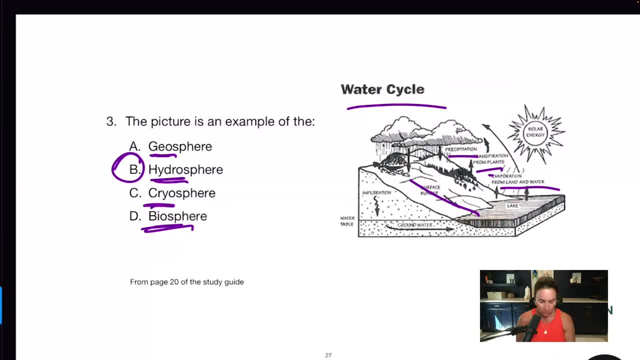 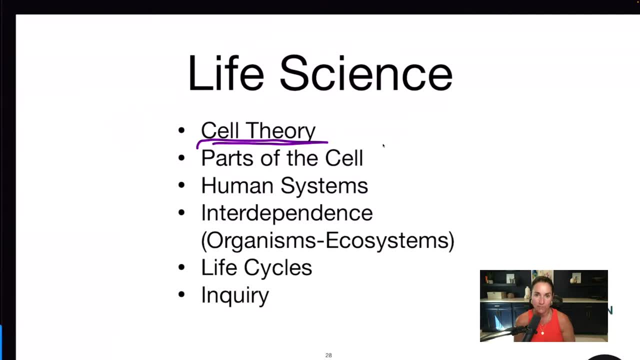 You know this is all about the water, And so that's going to be the hydrosphere there. Now, with life science, This is tough. This is everything from the basic unit of life, which is the cell. This was my favorite. 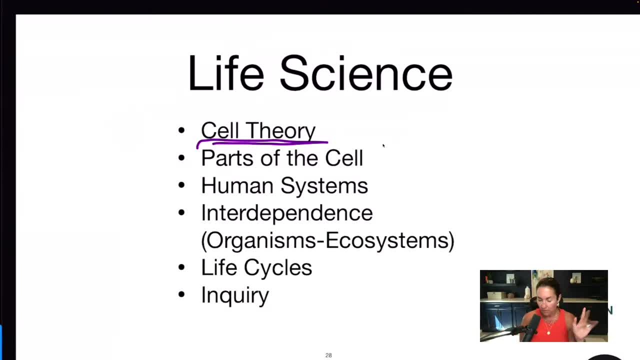 I taught bio in high school. This is when I fell in love with science. Cells and DNA and heredity was just like the coolest thing ever. I fell in love with it, teaching it. But life science is everything from cell theory all the way to life cycles like big life. 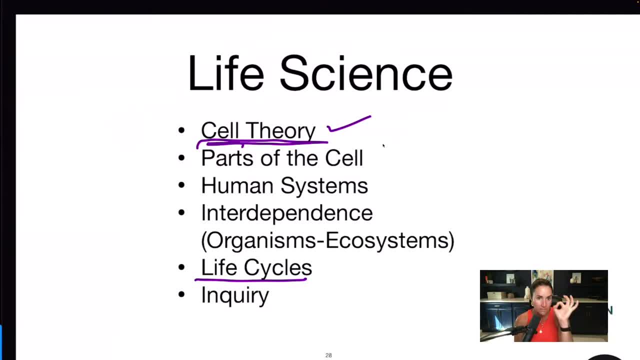 cycles on earth, in the biosphere. So everything from a single cellular organism all the way out to like an ecosystem full of different organisms. So, yeah, So it's got a lot and you're going to be asked a lot of different questions. 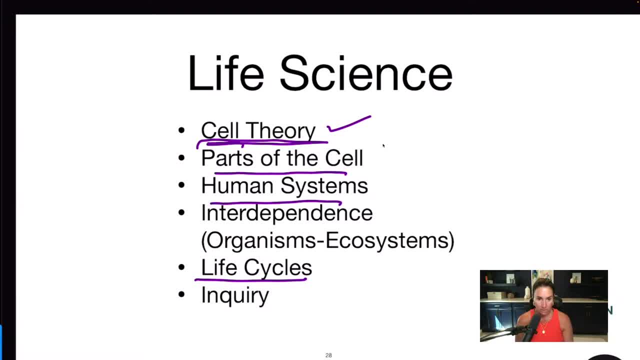 So everything from parts of the cell and how they work, to parts of humans and also animals, interdependence, organisms and ecosystems and how other organisms are interdependent on one another, Life cycles of you know, life cycle of a butterfly, life cycle of a frog life cycle. 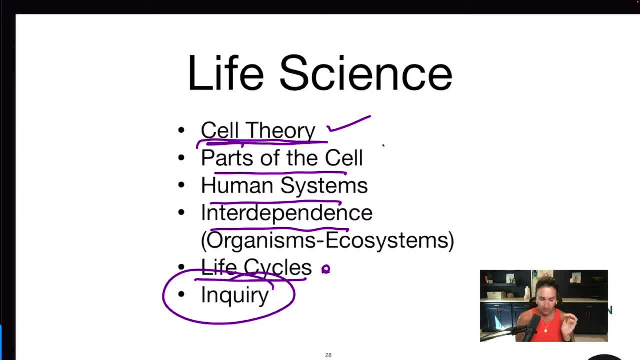 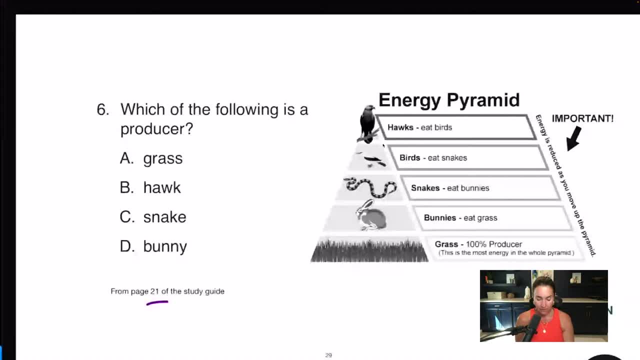 of a human. They're all different. And then, of course, inquiry again is going to be a good word on this exam. Let's have a look here. This is on page 21 of the free study Study guide number six, which of the following is a producer. 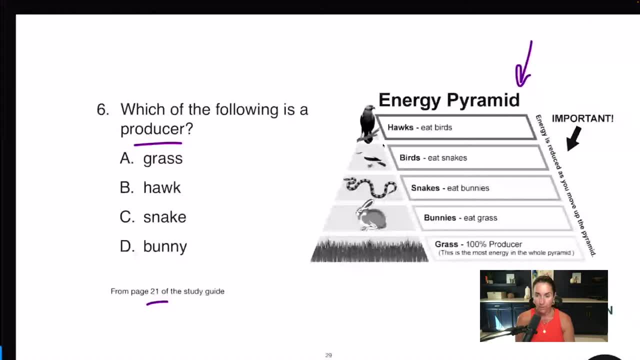 All right Now I added this here. This is from the actual study guide. I have this pyramid- energy pyramid- in the study guide and you could see it says a hundred percent producer, which is grass right, But you may not have this on the test. 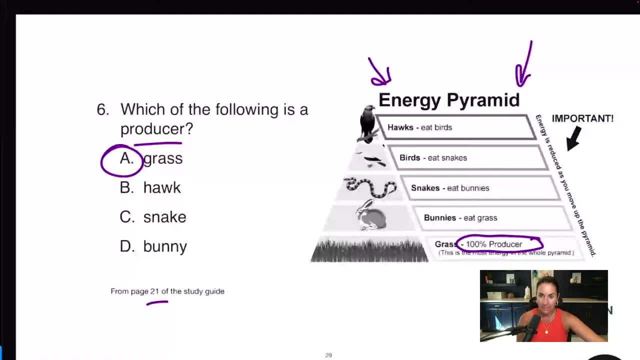 They may not give you the actual diagram. I added it here because I want you to see that the grass is a hundred percent producer. Why? Because the grass goes through a process of photosynthesis And it produces carbohydrates. The bunny eats the carbohydrates and gets energy. 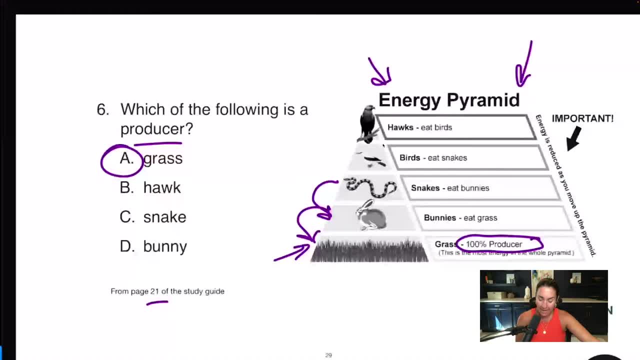 The snake eats the bunny and gets some energy, but energy is lost. A little bit of energy is lost And then the bird eats the snake, and then the Hawk eats the bird. The further up you go up the energy pyramid, you're losing some energy. 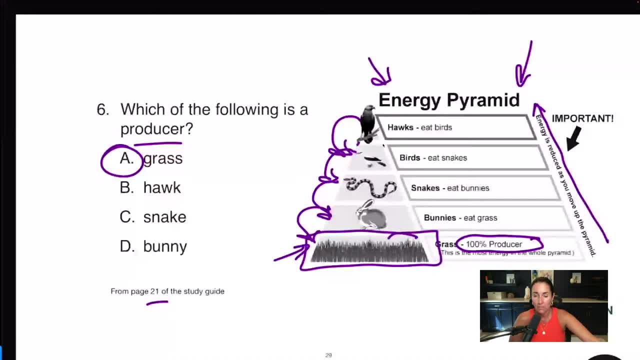 Most of the energy is stored down here in the grass and carbohydrates, Remember So. photosynthesis is um when plants take water and carbon dioxide and light and make sugar, carbohydrates and oxygen. that's the byproduct. We then eat animals, eat the carbohydrates and breathe in the oxygen. 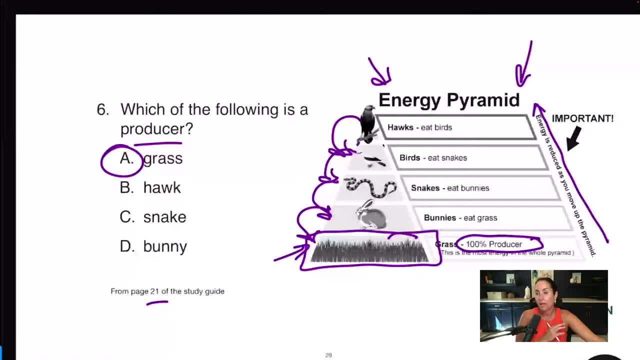 And then we give off CO2 and uh uh water, and the cycle goes on and on. So when you are moving up this pyramid here, you're losing energy. You're losing energy, You're losing energy. You're losing some energy because the bunny got most of the energy from the grass. 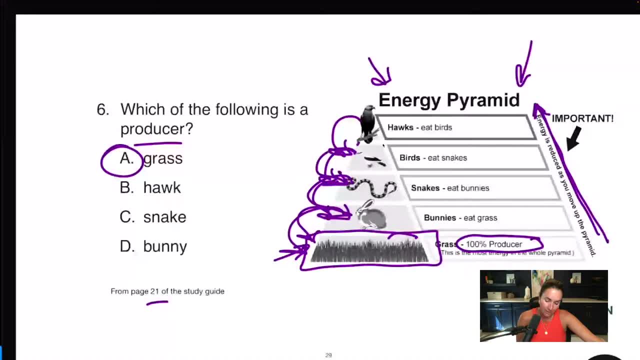 Then the snake gets some of that from the bunny, And then the bird gets some of that from the snake, and then the Hawk gets some of that from the bird. All right, But grass is the producer. trees, grass, flowers, things like that. 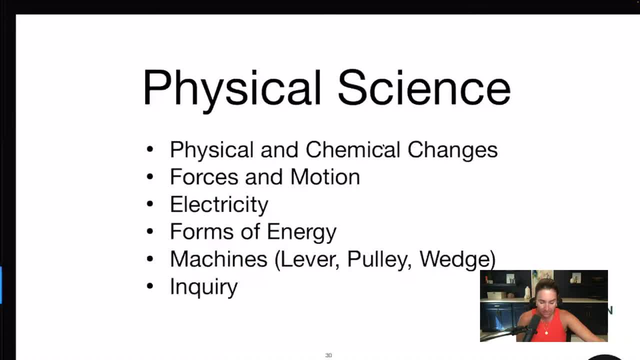 They are producers. All right, And let's go to the last one: Physical science. here I've got two to go with this one. Physical science is physics and chem, So anything that has to do with physical and chemical changes of forces in motion- electricity. 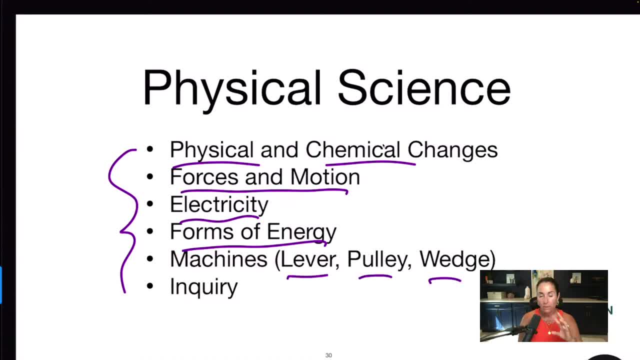 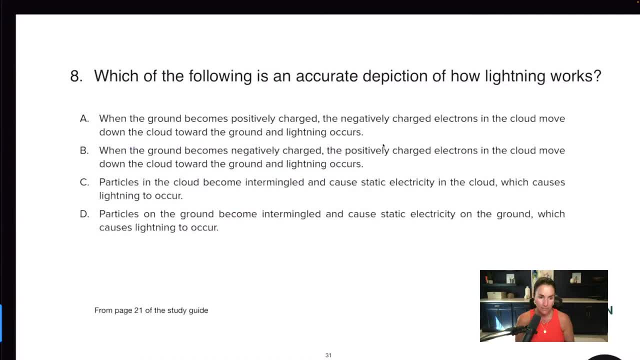 forms of energy machines. You got to know your um, you have to know your basic machines. And then, of course again, inquiry, good word. Let's have a look at this one. This one's about lightning. This is, uh, number eight, page 21.. 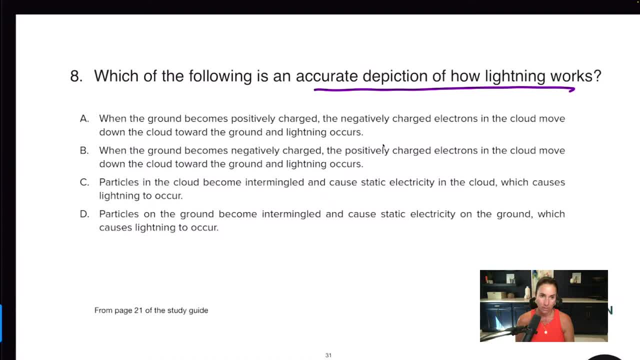 Okay, So which of the following is an accurate description of how lightning works? All right, So you can see. they do this a lot on the test. They'll have like things listed in different orders. You can see: a- when the ground becomes positively charged. B- when the ground becomes negatively. 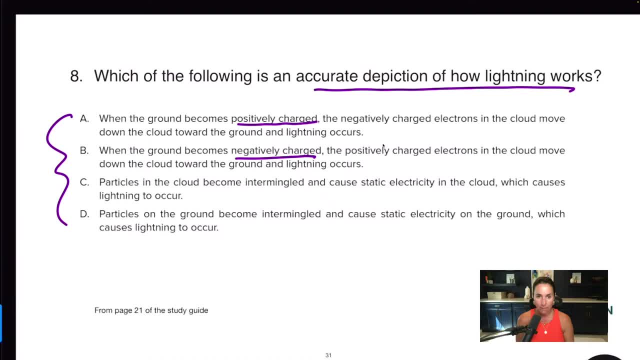 charged. Yeah, So they're the same thing happening. We're just mixing up what's going on here. So when the ground becomes positively charged, the negatively charged electrons in the cloud move down the cloud toward the ground and lightning occurs. A is actually correct. 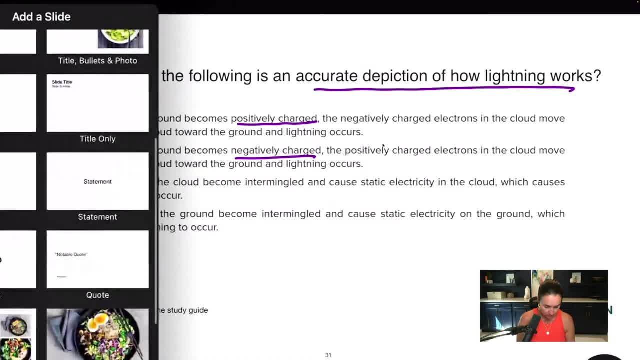 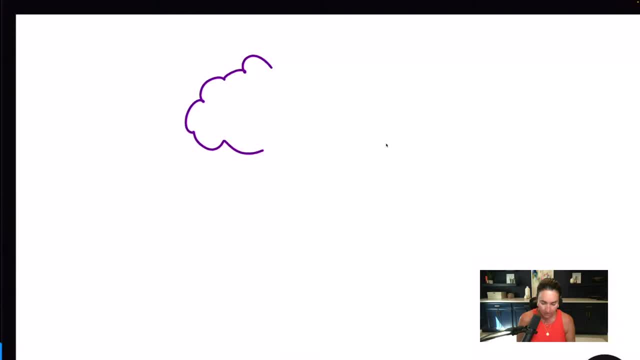 Let me do a little. um, let me see, Let me do a little. I'm going to draw a picture for you guys. It's not going to be pretty, All right. So here we have a cloud, All right, And, and here's the ground. 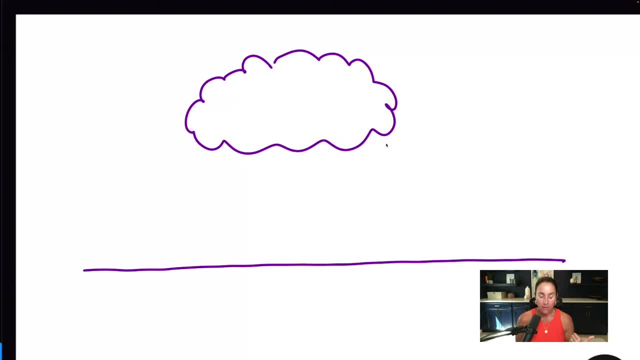 And what happens is At different parts, at different times, um, the negatively charged particles will start to move below the ground because everything's charged right, And then the positively charged particles will move up to the ground. And then what happens is because, um, uh, opposites attract negatively charged particles. 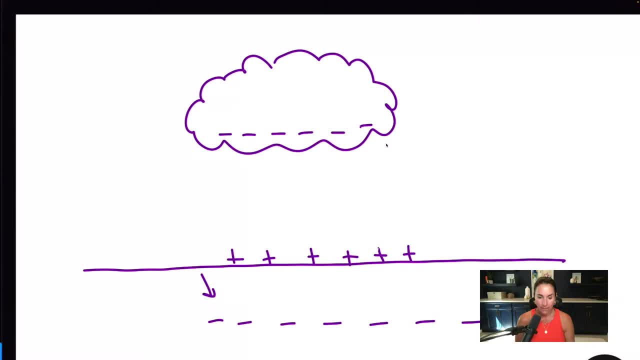 will start to move down the cloud. Okay, So the positively charged particles will move up into the cloud and notice we got negative and positive And when this becomes strong enough, shh lightning, shh. now, of course, it's a lot more. 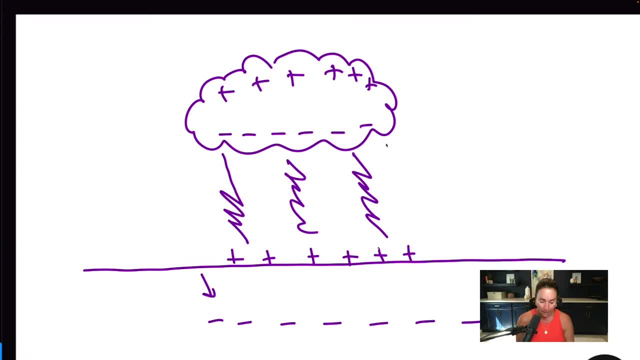 technical than that, but for this test that's all you need to know. So the ground becomes positively charged and the cloud becomes negatively charged at the bottom. It's and it doesn't happen the other way around. It's not. you don't have positively charged in the cloud at the bottom and negatively. 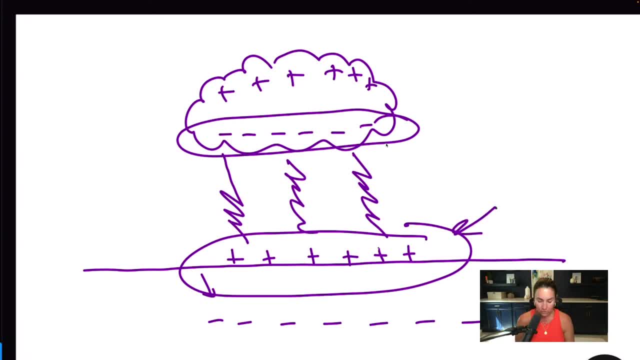 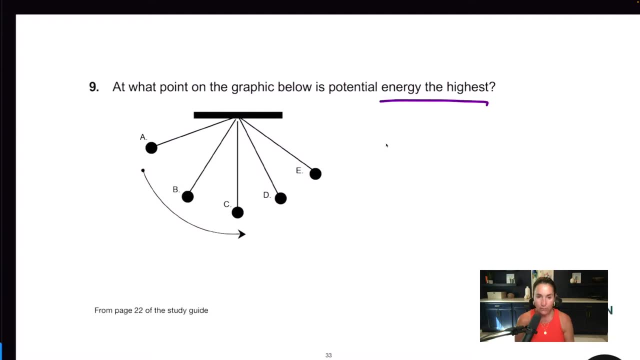 charged ground. Okay, So when the ground becomes positively charged and the cloud gets that negative charge at the bottom and lightning occurs, okay, that happens periodically. Let's have a look at energy. At what point on the graphic below is potential energy? the highest potential energy is the. 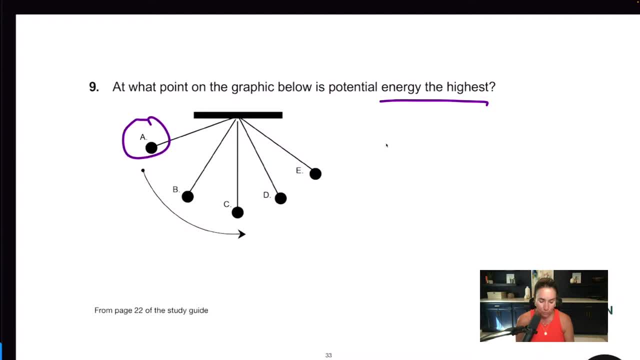 highest when kinetic energy is the lowest. a is when potential energy is the highest. If I were to pull that pulley up here before I let it go, It's at its highest potential energy. When I let it go now, it's in kinetic energy. 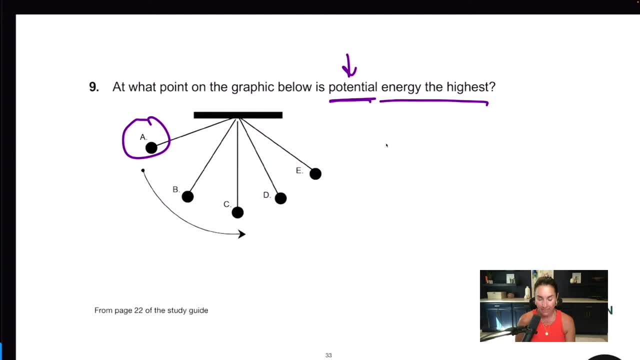 If it asked here at what point of the graphic is kinetic energy the highest, that's going to be C. kinetic energy is going to be highest when it's right at the bottom and it's moving down towards that pendulum. Then we got a little bit of potential energy here at E, not as high as a. a is the highest. 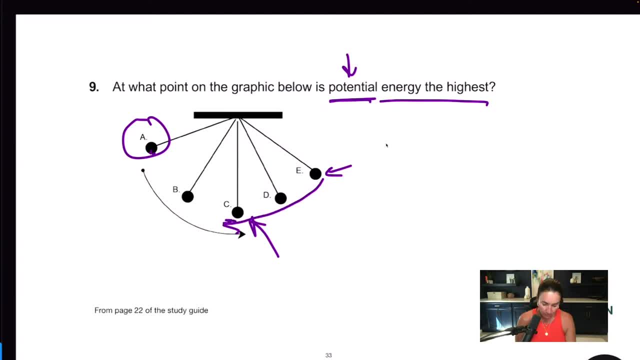 potential and then you know it comes back down here and then here and it swings back and forth until it comes to a stop. Okay, So potential energy is a it's at the top, If you see it as like done on a hill, and maybe it's a car or a person, I don't know- like 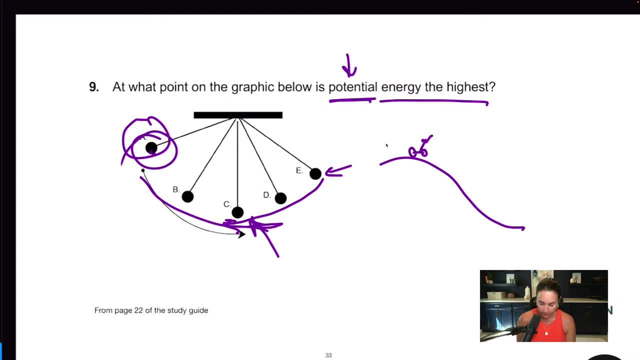 a bike. let's just put a bike here and the bike is moving down the hill. Um, the potential energy is highest at the top of the hill and a kinetic energy is lowest right here before it. right before it hits the bottom of the hill, it's at its highest. 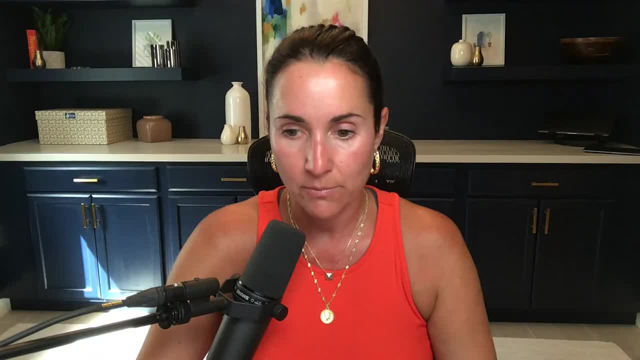 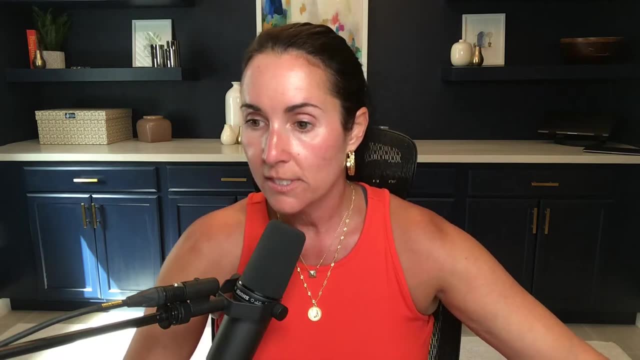 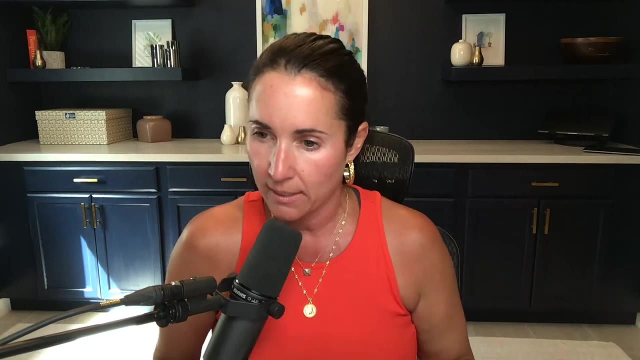 Okay, All right, Let's go back here. Stop sharing. All right, Let's go back here, All right. So that concludes the presentation today. Um, is this the test that will replace the Mogea Dawn? I don't know what you're asking. 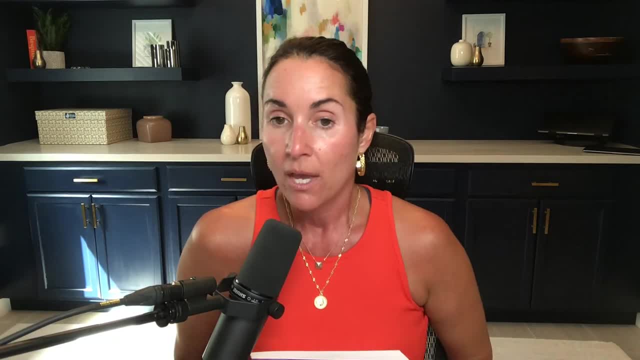 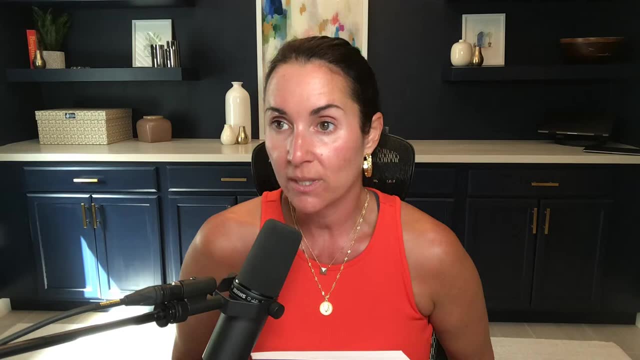 the M O G E A. I don't know what tests you're asking about. There is a new elementary education test coming out, the seven zero zero one that was just released. The specs were just released, but the states that are using it has not been released. 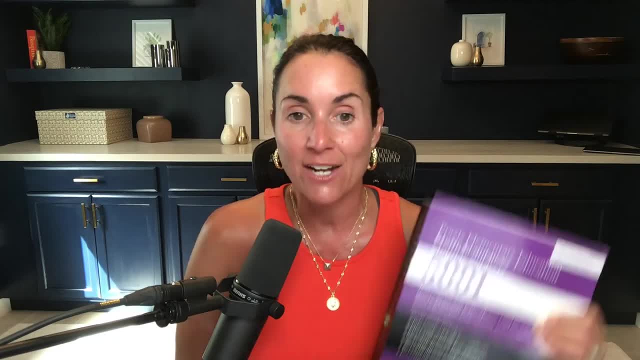 I've been monitoring it like crazy. Okay, Does the specs look identical to this? So not much has changed. Um, but I will be keeping an eye on on that, All right. Is there a social studies glossary? Um, Mike, there's not a glossary, not in my book. 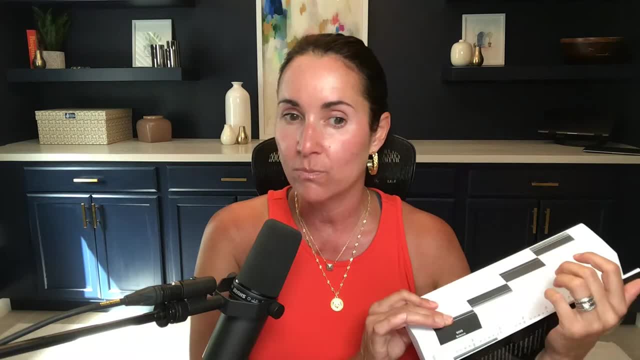 There are some um charts and graphs and things like that, but I cover everything that's in the specs in the book. What is the best way to study for this part? I do not remember these dates so well. Um, you might be asking about, let's see, it's 1110.. 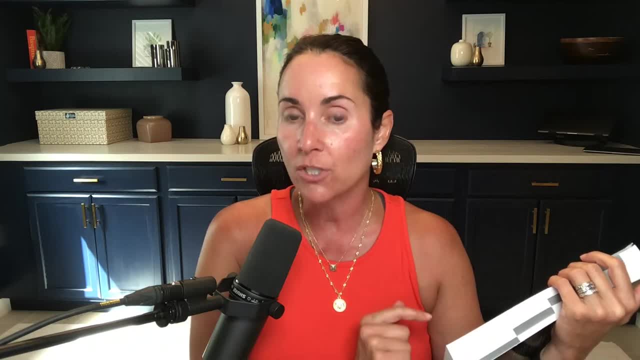 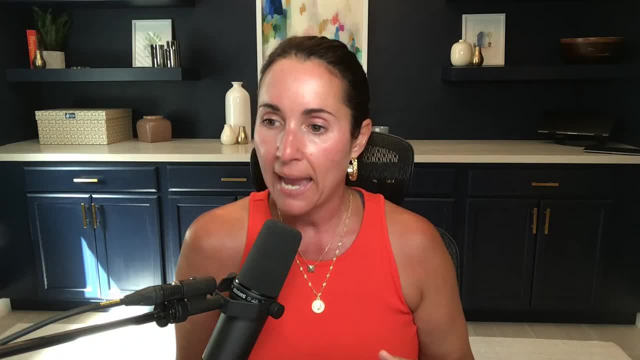 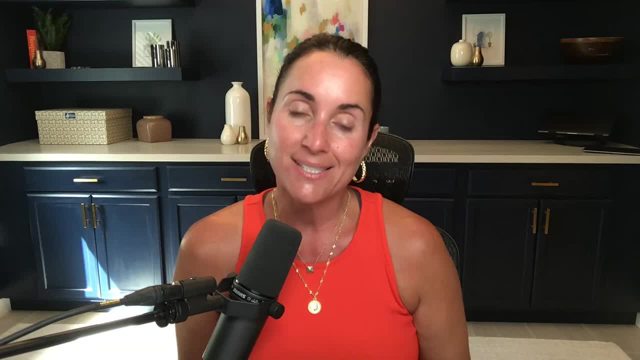 Um, you know it's kind of hard with the social studies and science because it's more memorization of concepts than it is really of anything else. I know it's hard. Um, you just really have to understand what's in the specs and I outline everything that's. 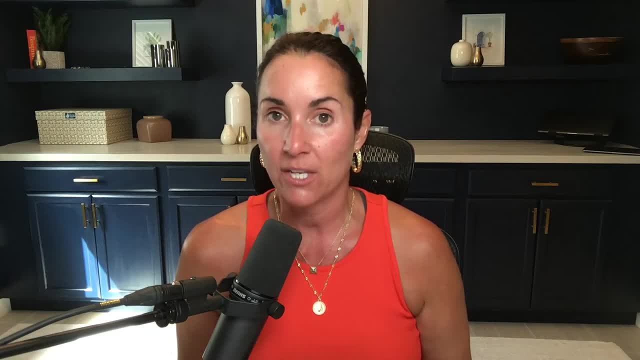 in the specs in the book. but you can also download the test specifications by Googling praxis 5001 study companion. If you Google, that will be taken to a document. make sure it's on the ets website and it's a pdf and it shows you. 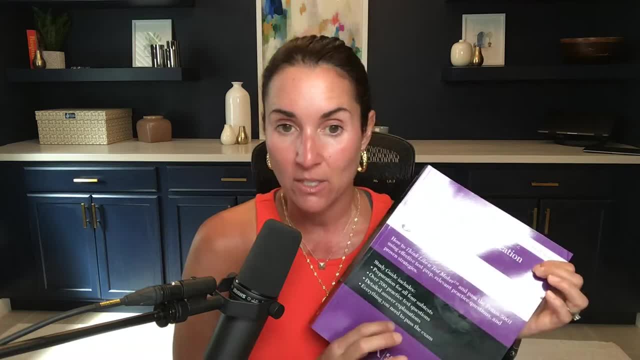 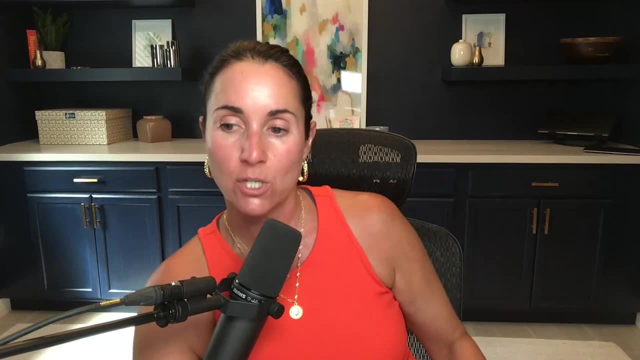 everything that's on the exam. now i cover everything that's on these specs in the book, but you might want to look at that document yourself, all right, and that'll help you. uh, do you have a test for business education? no, i do not, charles. sorry about that. uh, sabrina, thank you for. 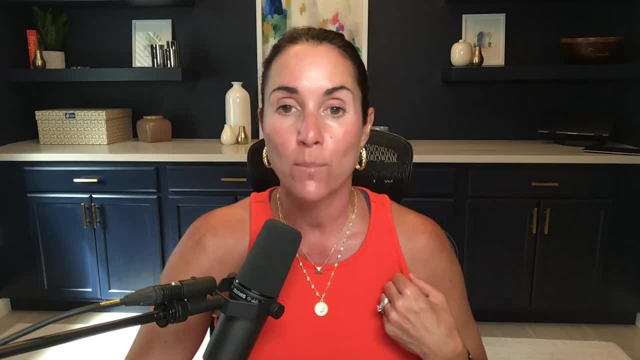 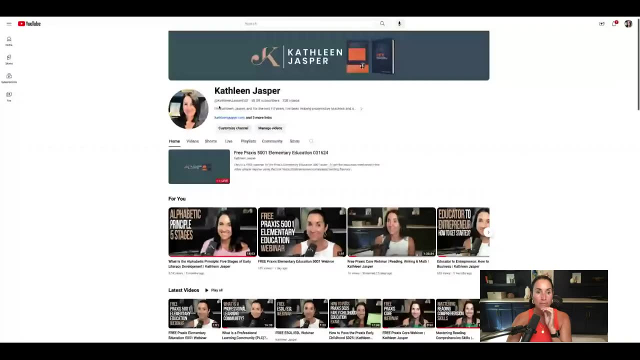 all your help. thank you for attending, sabrina. all right, real quick, i want to show you where you can get more resources. okay, uh, free, free resources. so let me just share my screen here. so, on my youtube channel, i talked a little bit about that today. um, i've got test strategy. you're definitely going to 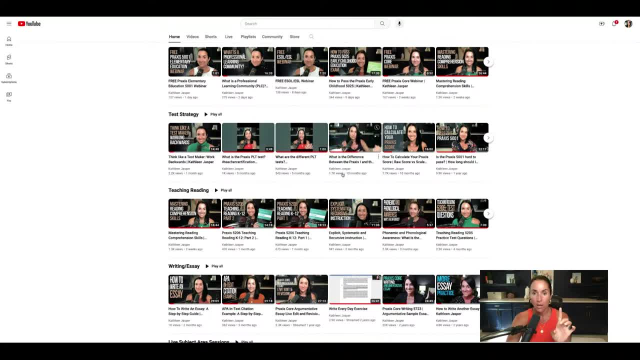 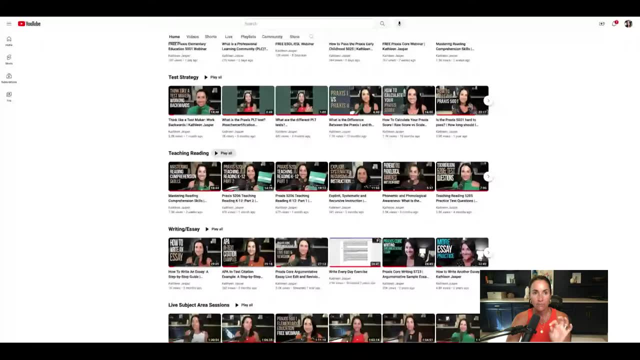 want to look at that. somebody was asking me about the difference between, uh, praxis one versus praxis two. i have a video on that here. the teaching reading playlist is going to help you tremendously with the 5002. that's going to help you a lot. um, and then, of course, um, you can check out our online. 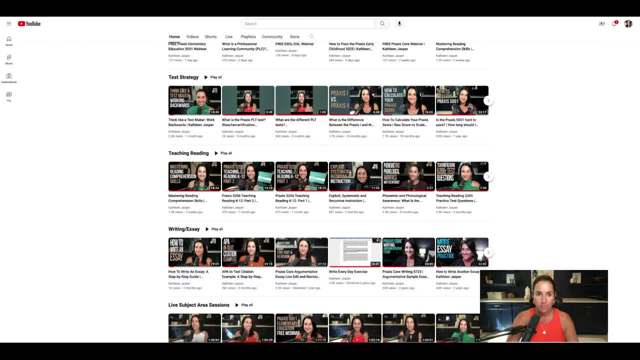 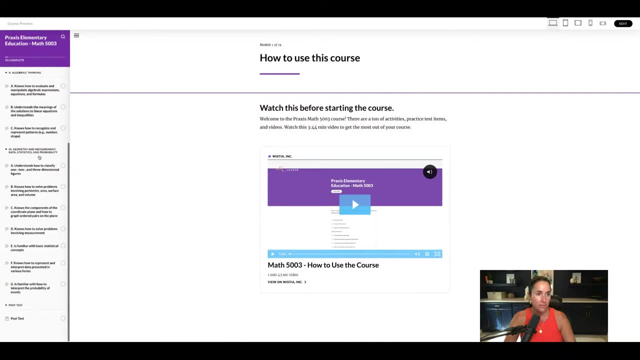 courses, which let me just give you like. this is the math. let me just show you the math really quick. hey, on one second preview. so this is the math and you can see that when you start course, i mean: look at this menu on the side, it's got everything here. um, of course, you get the study guide with all. 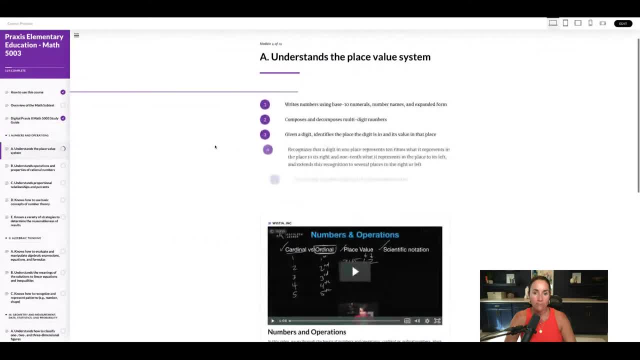 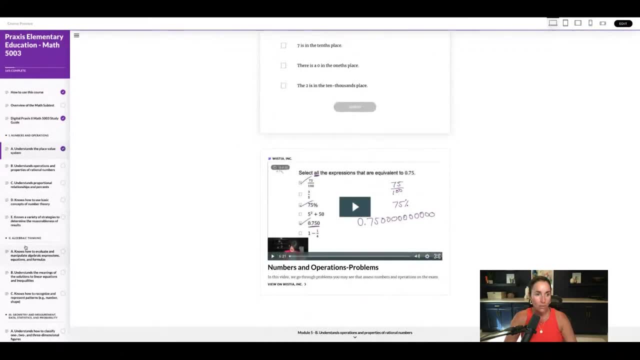 of our online courses. you get the study guide, but you're going to get videos, extra practice here. you're just going to continue through the module. i do go through a lot of the questions, some of the harder questions, and i do that for everything. so there's going to be questions and then 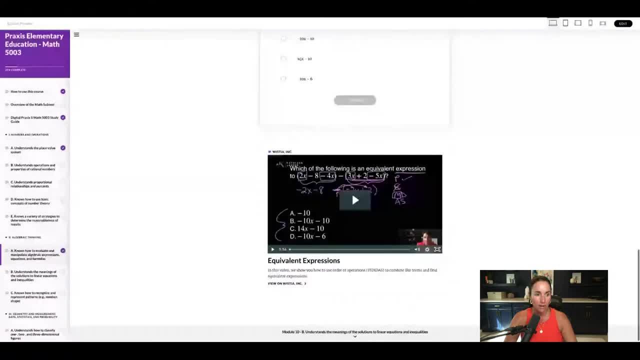 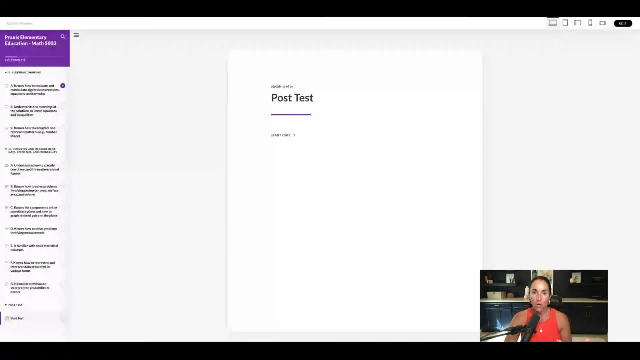 explanation of the questions. these are all extra practice within there. and then, of course, you know we have a post test which is simulated like test day, although ets has their own, their own stuff. so mine is the way, mine looks right, but you know you can go through this and it's similar. and then 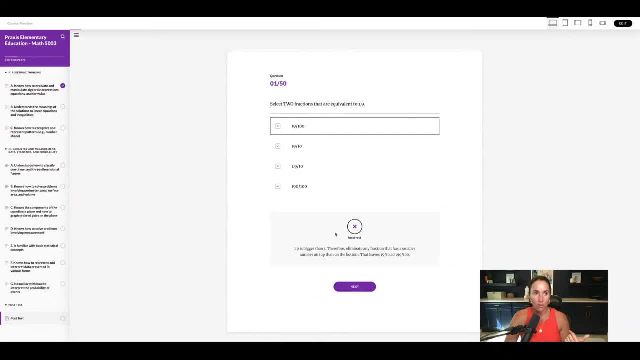 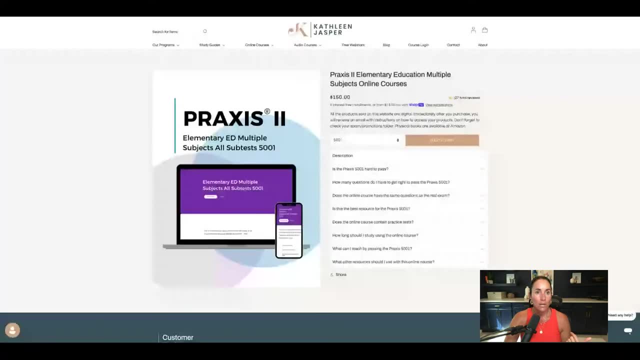 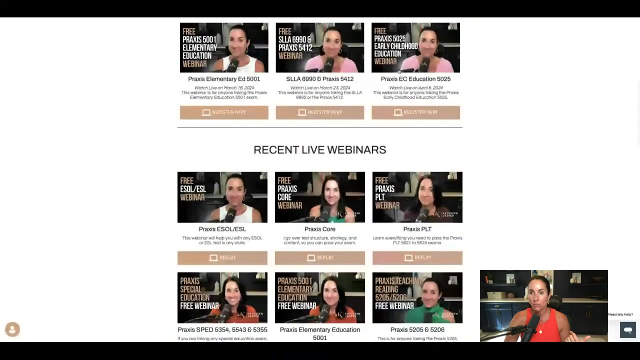 it has answer explanations in there for you as well. all right now i also have let's see here, let's go to. we've got free webinars and a couple of you were asking about those coming up for uh, praxis, early childhood education. i've got that coming up here next week is going to be the slla. that's our. 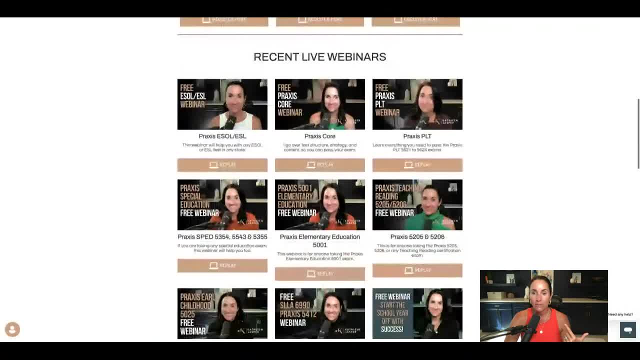 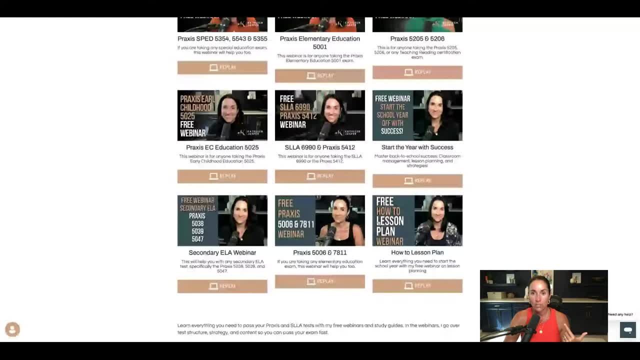 leadership exam. a lot of you are going for leadership, and then i have all these other ones. if you don't have time to wait, i've got all these other ones here. early childhood: here: how to lesson plan. this is really good for new teachers. how does this one's about classroom? 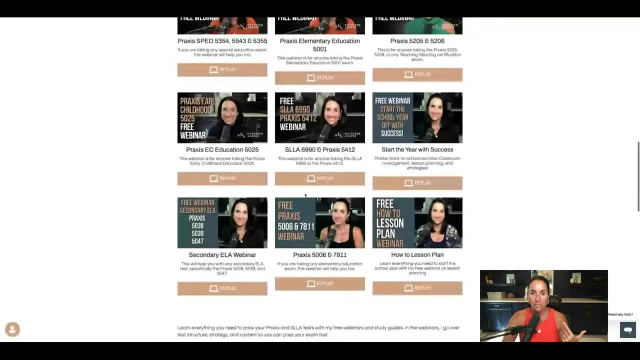 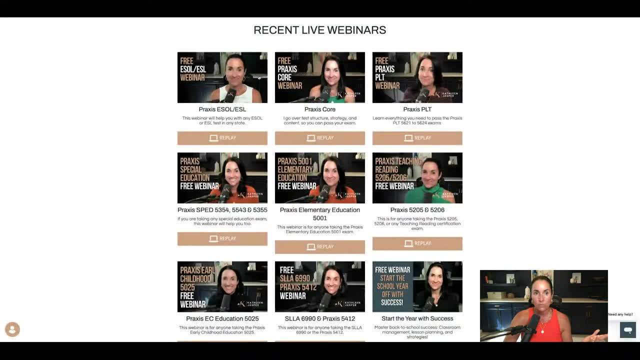 management. this one's about secondary ela. five zero zero six. some of you are asking about other tests. i've got them all here. some of you are asking about other tests. i've got them all here. plt i just did here. it is plt. praxis core was last week esol, so check out those. we'll link that. 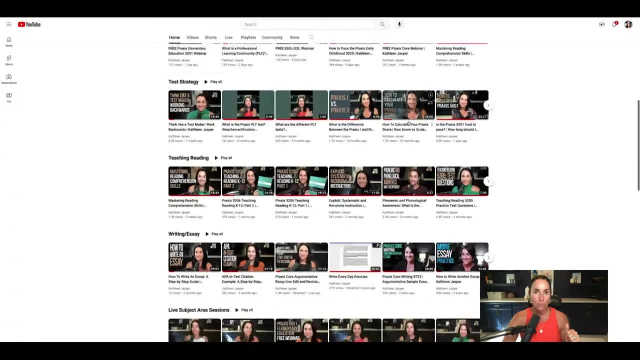 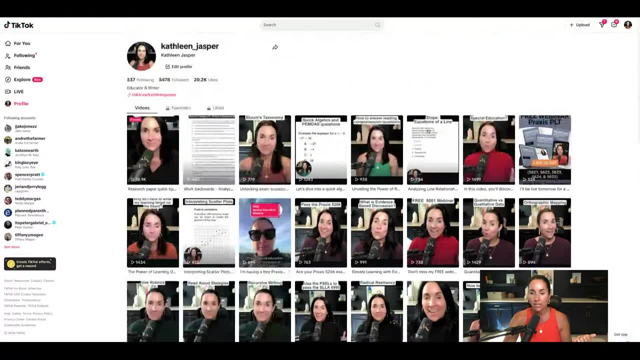 up. then, of course, i've got my youtube channel, which i already shared, and then tick tock, if you like shorter videos. i do a lot of short videos. i do math, i do science, social studies and i do a lot of reading instruction here. so check me out on tick tock if you like tick tock. and then, of course, 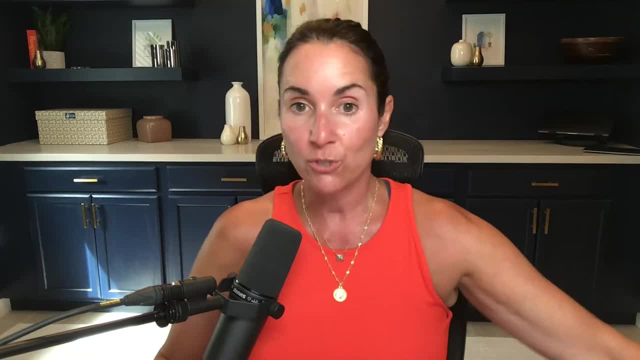 facebook. i'm always live on facebook, so be sure you check out our study guide if you're interested in that. if you're interested in our study guide, there's a link that's in the description box below on how to study social studies here and we'll give you a link to our study guide link in a second in. 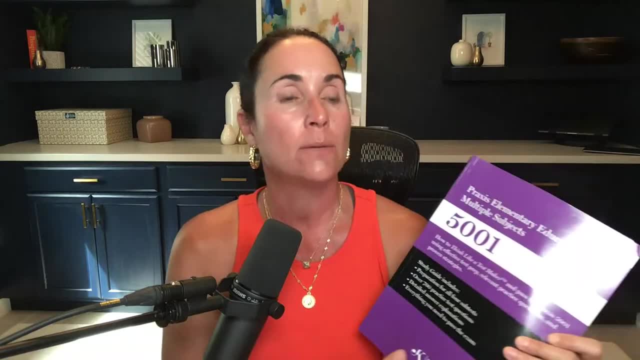 If you liked it. leave me a review on Amazon if you wouldn't mind, And you can always email us if you have any questions or concerns about anything. I'm so glad you guys were here with me today. I know it's a long one. 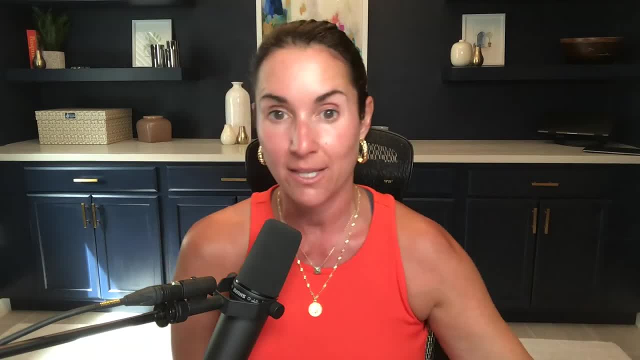 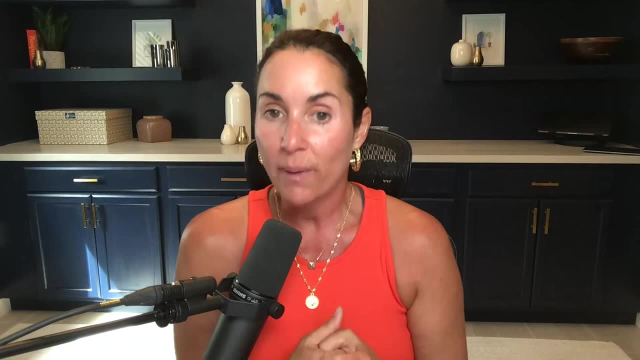 This is a big test and it's Saturday and you guys are probably tired. You're coming to the end of the year and you want to chill out, not work. but you know, get through this test and remember it's okay if you don't pass everything the first time. 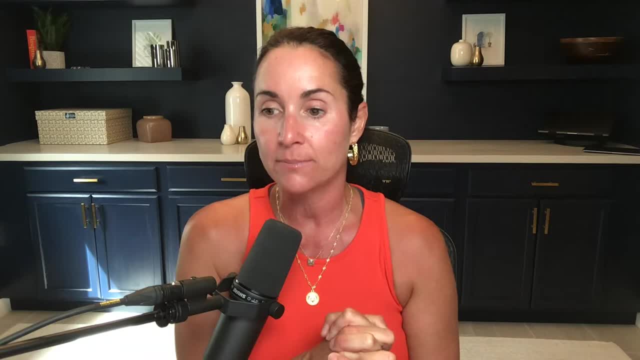 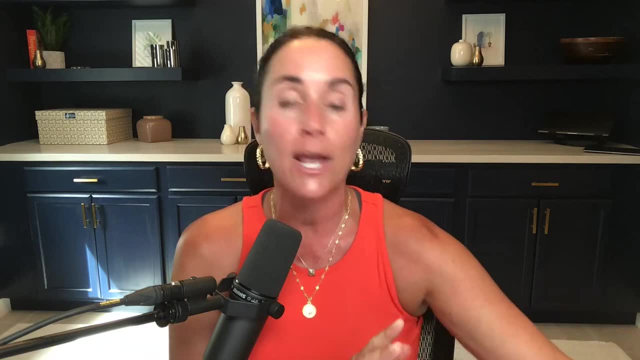 This is a big test, So go easy on yourselves and all of that. So if you have any questions about your orders or you want to apply, oh, here's one thing: If you've already purchased this on Amazon and you want the online course, email us. 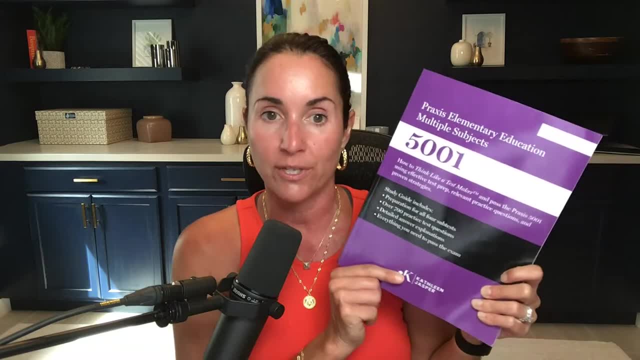 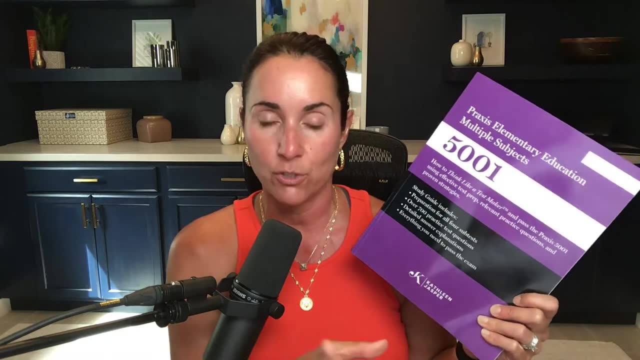 We'll give you an offer code to apply this to the online course, So you'll get this money off. It's $42.99 on Amazon. We'll give you an offer code and you'll get that off the online course. You don't have to pay for it twice, because you get the book with the course. 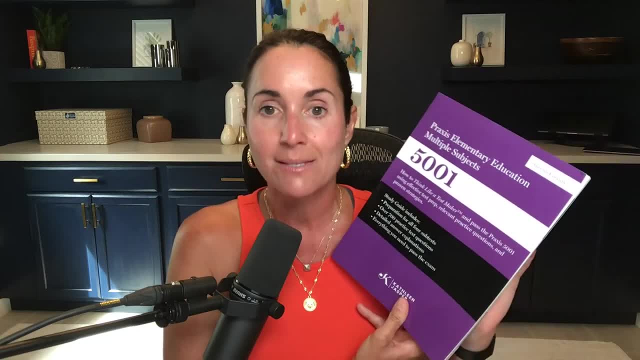 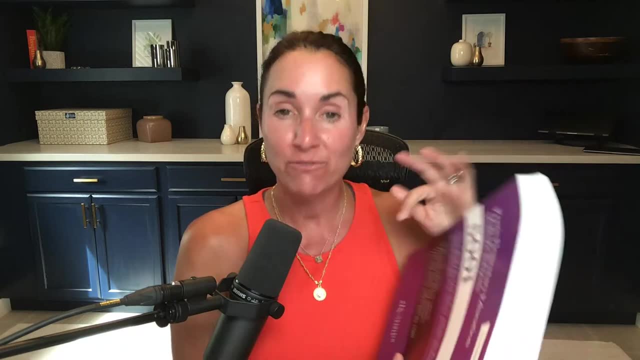 So, if you purchase the physical, email us. Hey, I purchased the physical. Send us a picture of the order, Not just a picture, A picture of your book, of the order and your name visible so we can see that and we'll. 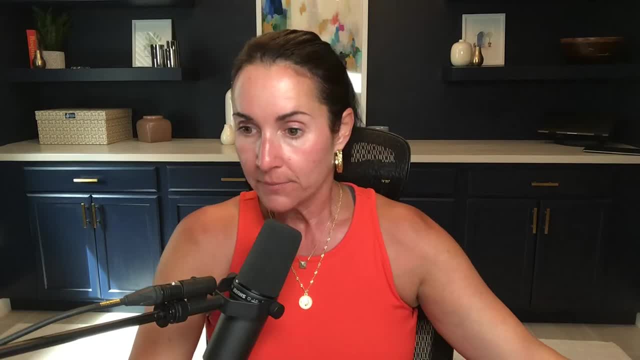 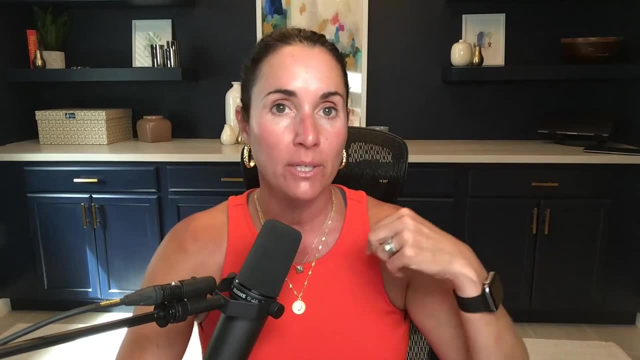 send you an offer code and it'll take that money off the book for you. Okay, Can you put up the YouTube link? It's Heather, It's Kathleen Jasper on YouTube. I'll also link it up in the email, but here you go. 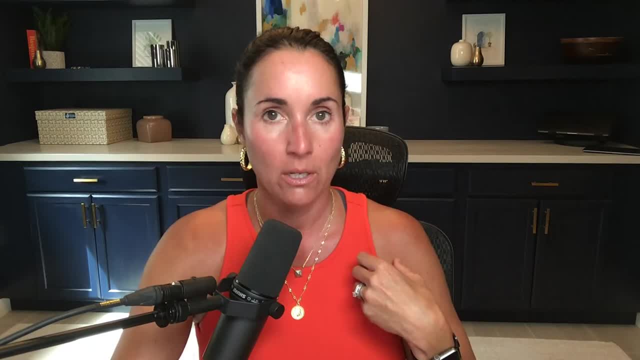 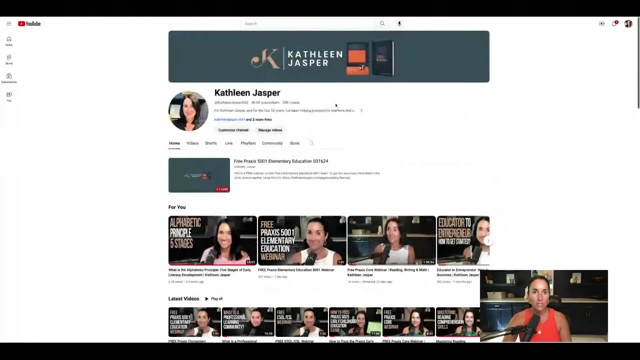 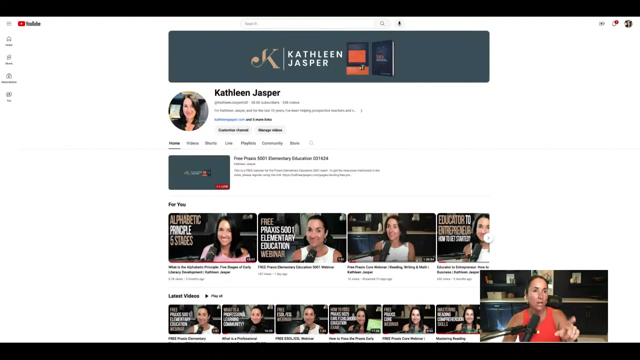 Let's just make sure screen It's all right here. Kathleen Jasper. If you search Kathleen Jasper, it'll come up, But I'll go ahead and throw this. You can also. it's YouTube slash Kathleen Jasper. EDD will help it as well. 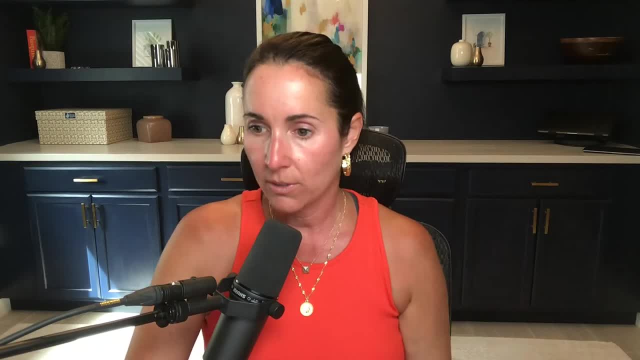 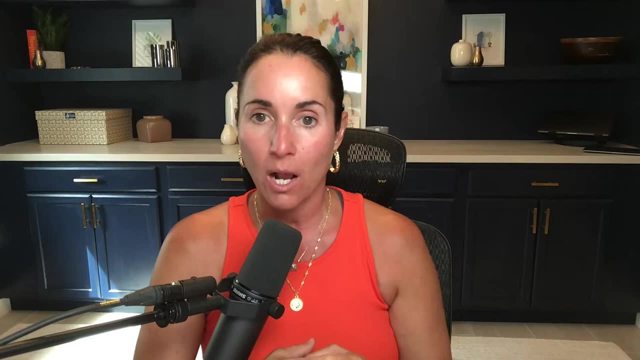 But let me just go ahead and grab that. I'll throw it in here. There you go. There's the YouTube link. What is your email, Latoya, if you want to email us, it's info at KathleenJaspercom. 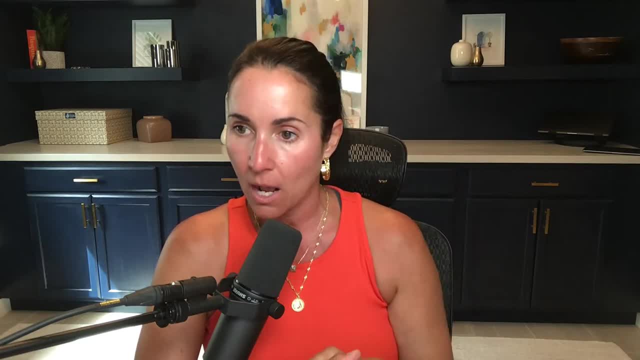 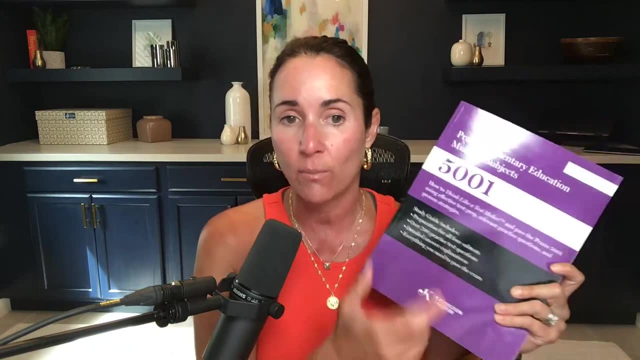 You can also find it on our website info at KathleenJaspercom. All right, I have the book. Awesome, I'm so glad you have the book. If you guys like the book, please review it on Amazon, if you don't mind. 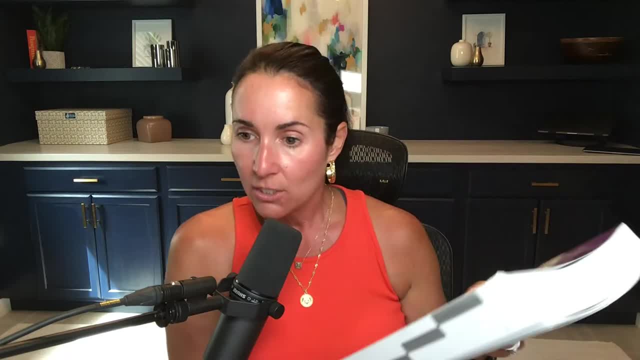 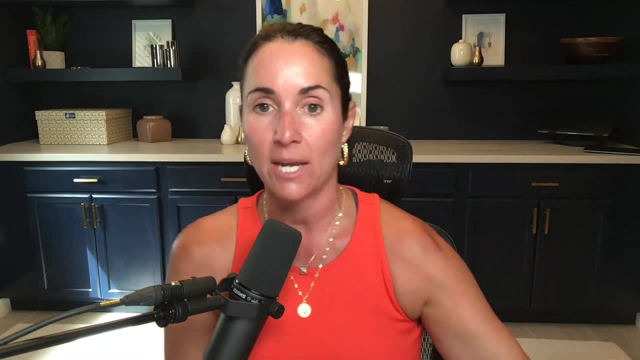 This one just came out, so we need as many reviews as we can get. Do you think your online course will help me with pre-K-3 science and developmental knowledge? in Florida, Mercedes, we don't prep for Florida exams anymore. I do have an early childhood education free webinar. 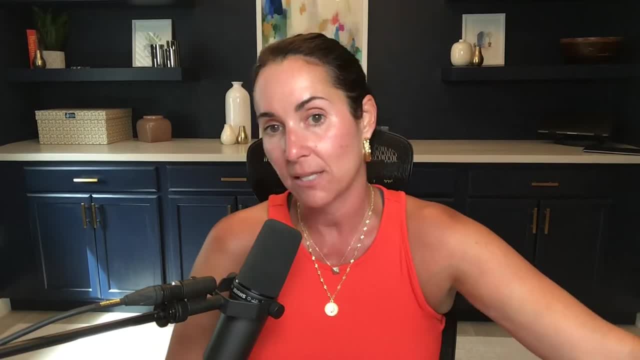 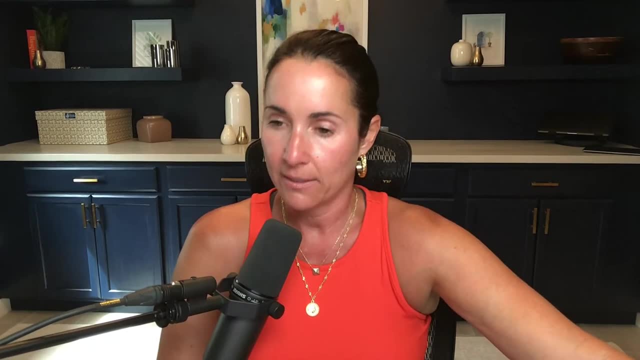 I recommend our free stuff first because our stuff is aligned to Praxis, not the Florida test. But check out our free stuff and if you think you like it, you can certainly use it, But it's not aligned to Florida. Thank you so much, Brandy. 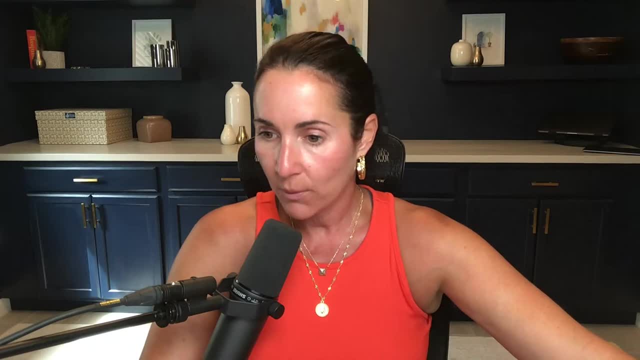 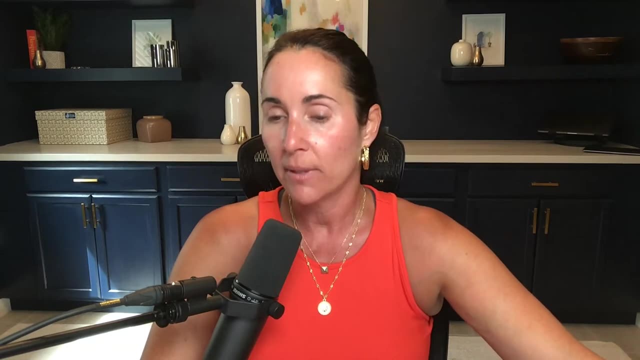 I appreciate your support. I'm glad you're here. Do you have anything to help with SEL standards, SEL, social emotional learning- not at the moment. A lot of that's embedded in our books already because we do a lot of teaching scenarios. 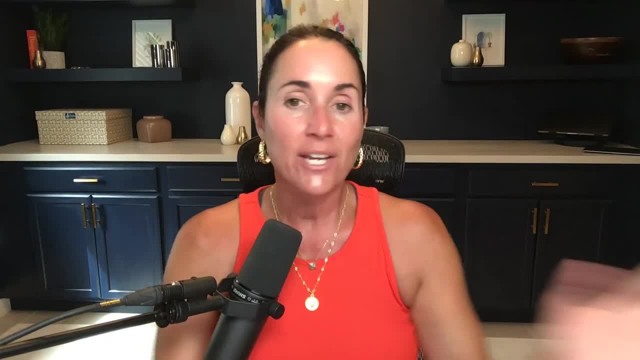 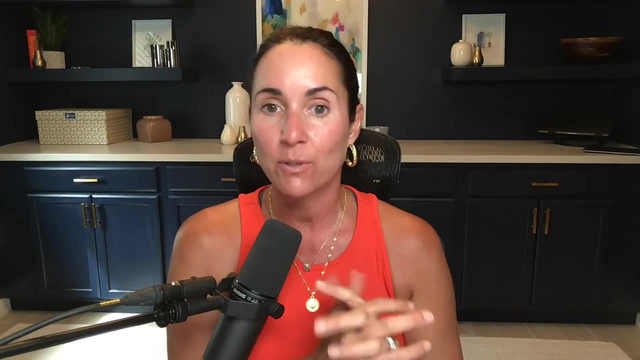 but not specifically SEL. All right, All right, you guys. Well, thank you so much for joining me today. I'm going to cut you guys loose. now. It is almost 1130, and I'm really happy you guys joined me today.